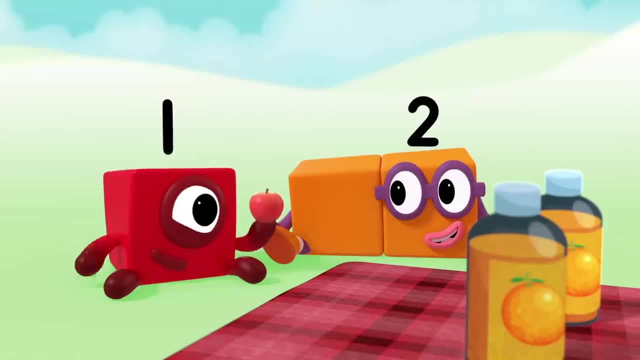 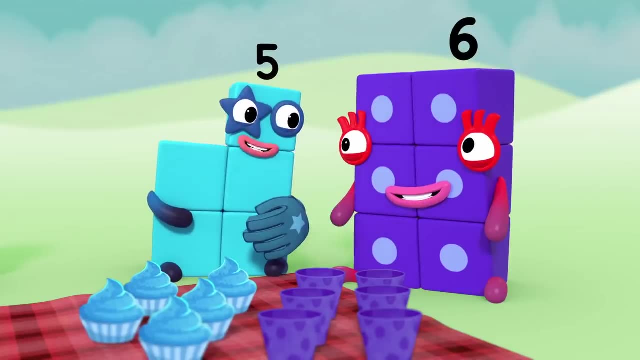 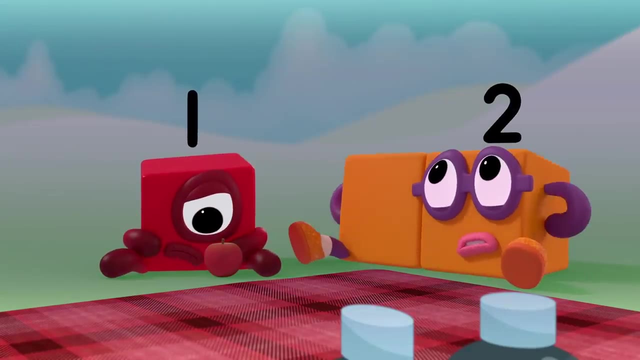 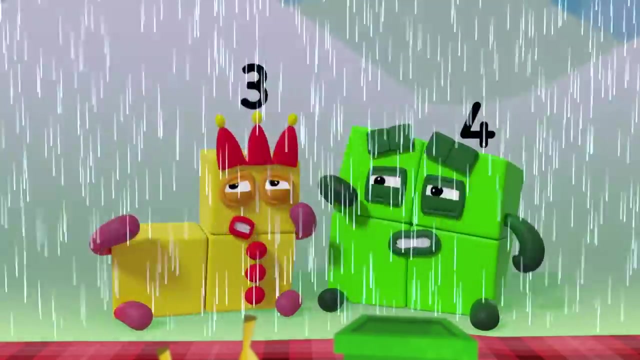 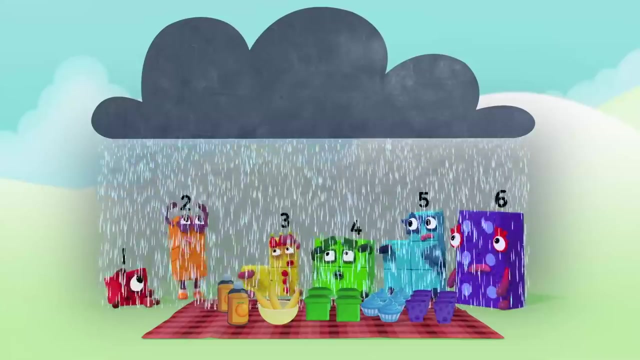 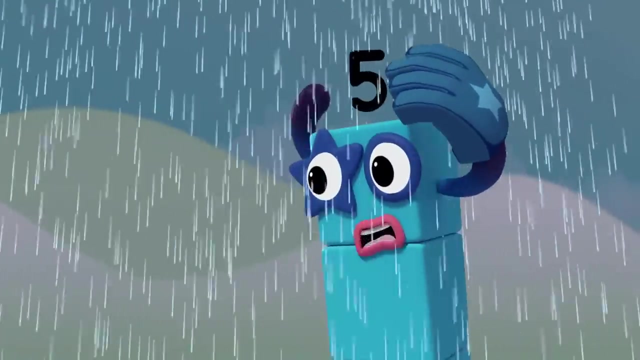 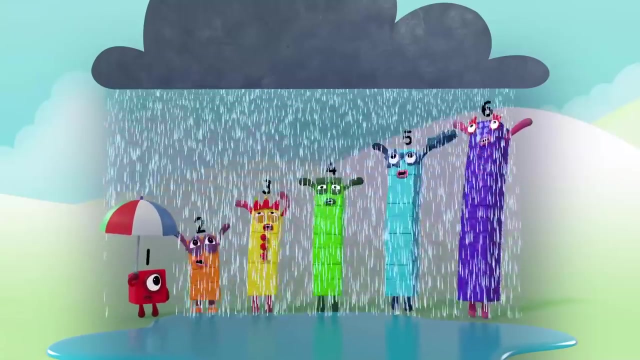 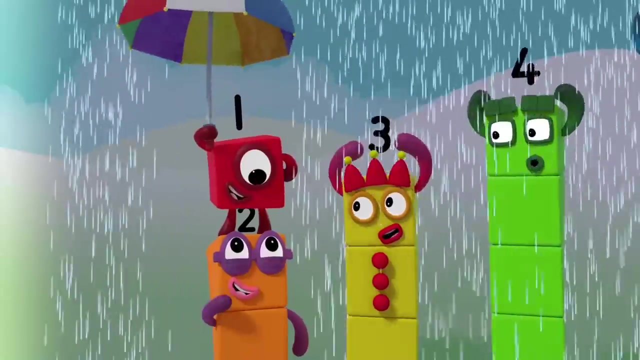 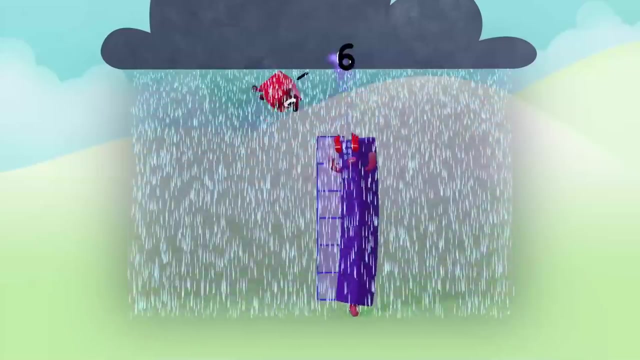 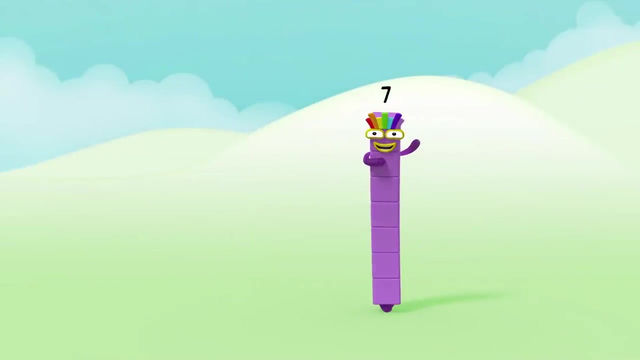 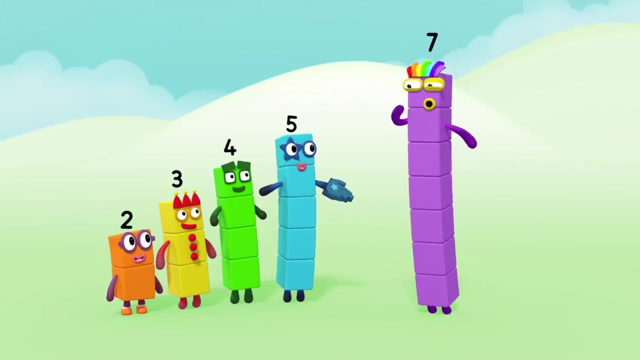 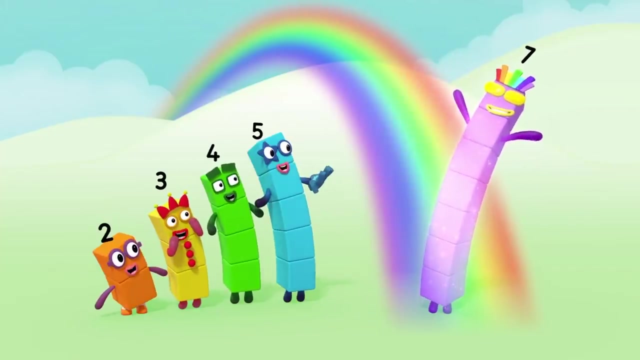 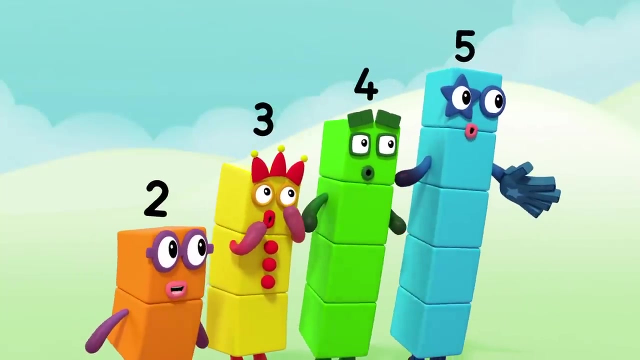 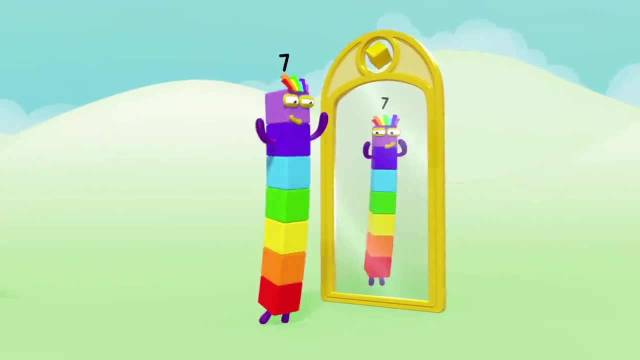 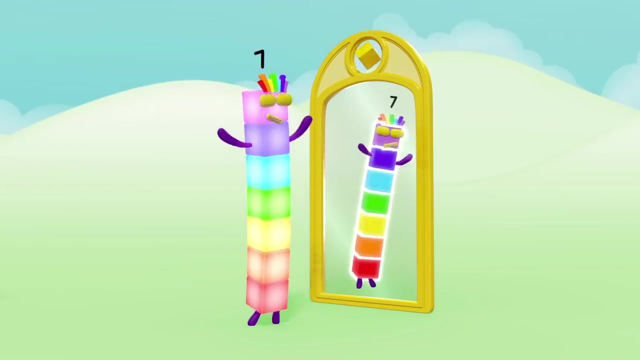 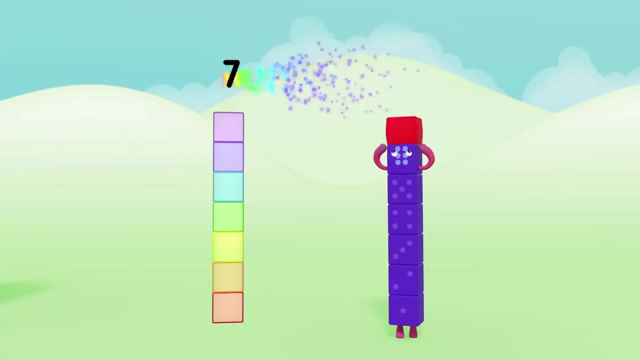 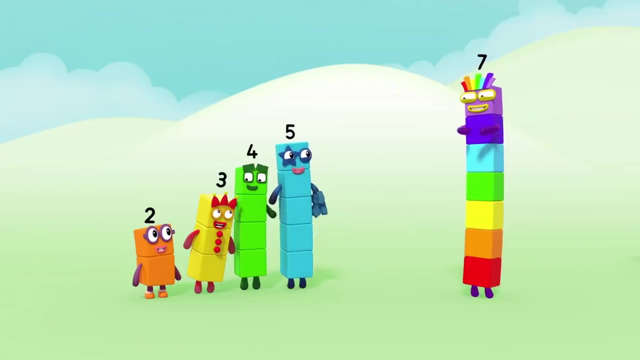 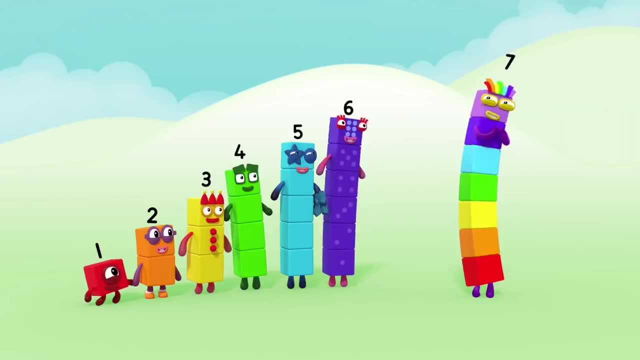 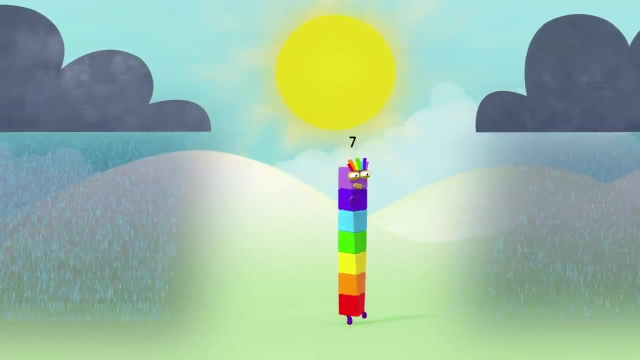 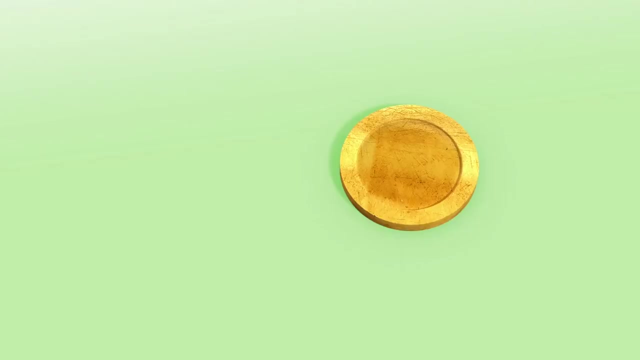 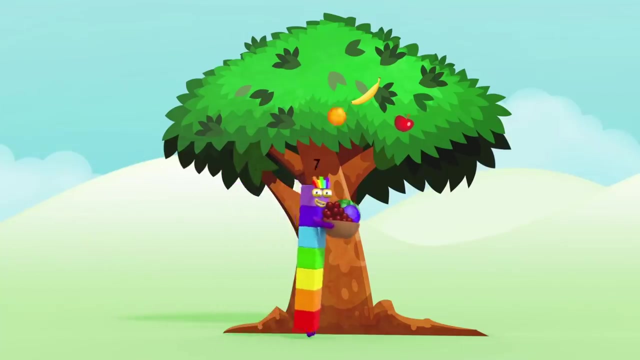 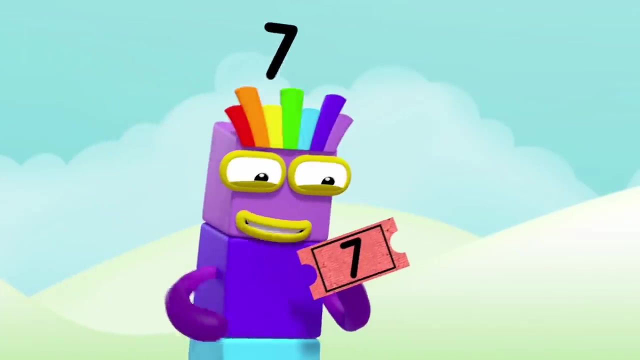 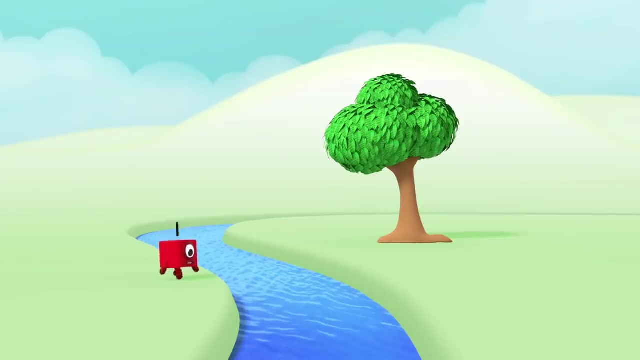 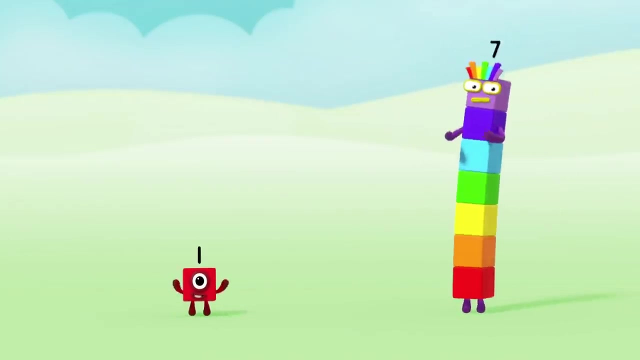 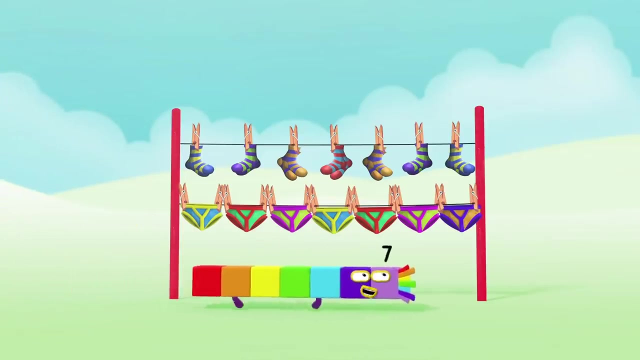 Please subscribe to our channel for more videos. Thank you for watching. Please subscribe to our channel for more videos. Thank you for watching. Please subscribe to our channel for more videos. Thank you for watching. Please subscribe to our channel for more videos. 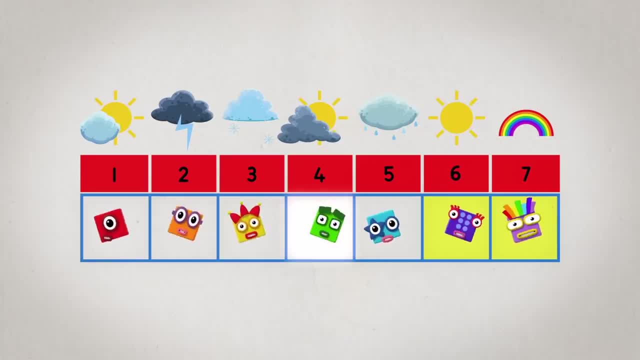 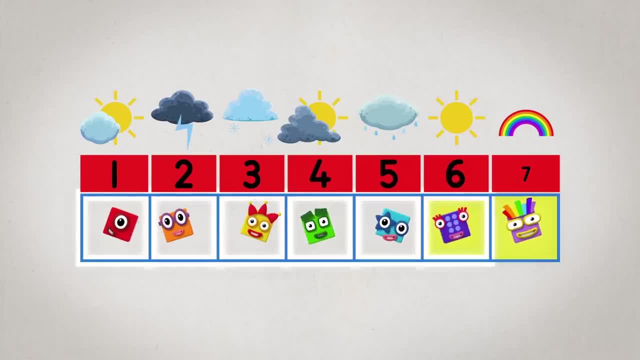 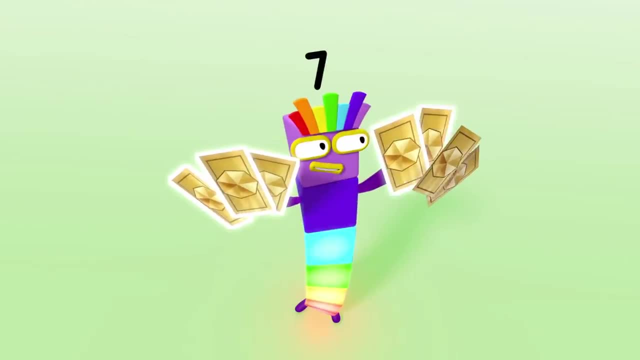 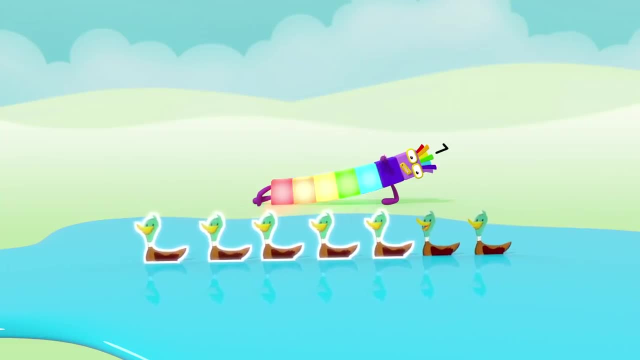 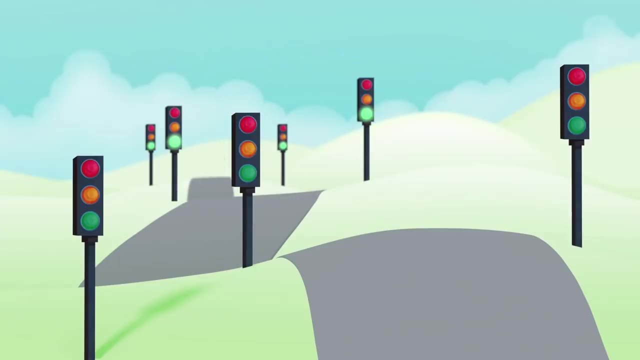 Please subscribe to our channel for more videos. Please subscribe to our channel for more videos. Three, four, five, six, seven. Nothing's gonna stop me. All my traffic lights Are on. go. I'm lucky number seven. I'd like to chance my arm. 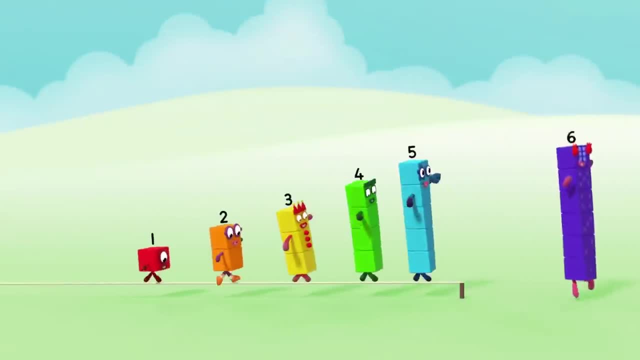 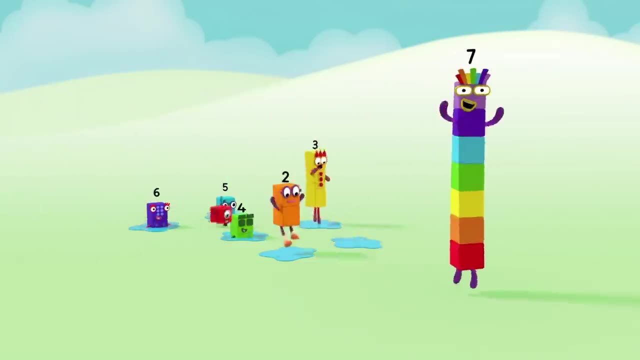 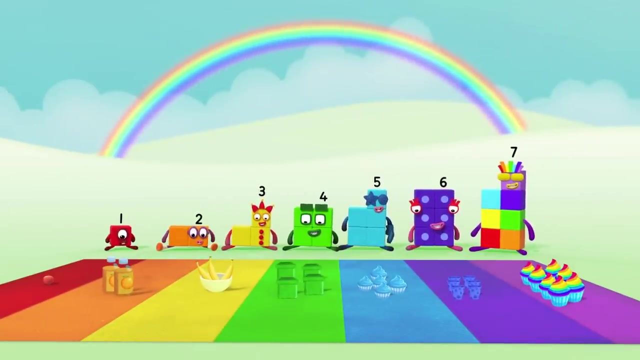 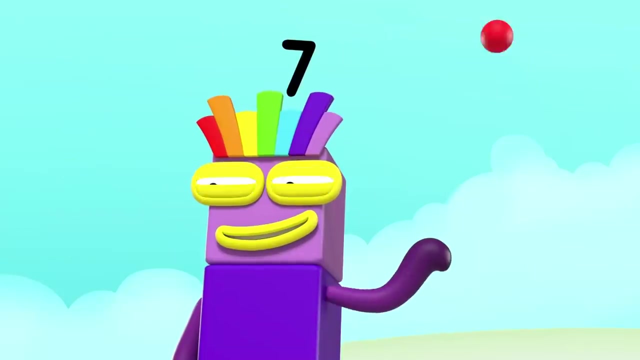 In tricky situations. There's really no reason for alarm. I take problems in my stride. I've got fortune on my side. I'm lucky number seven. When you're with me, I'll be your lucky charm. One, two, three, bump, bump, bump, Lucky catch. 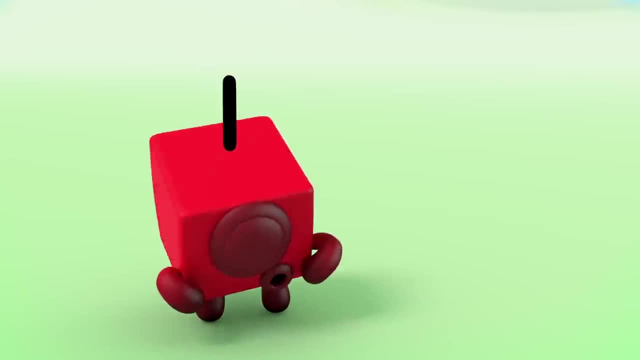 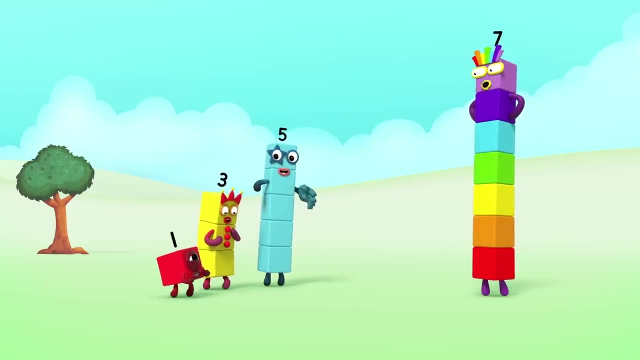 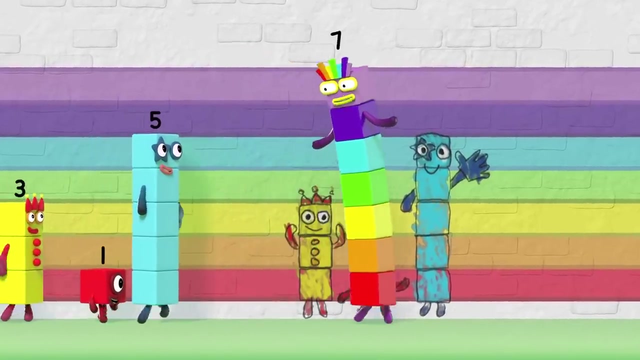 I wish I could be you. Seven, You're so lucky You can be me. Just ask a friend to jump on your head, But first You've got to be lucky. You have to know the difference Between you and me. We all have our place, But we're different. 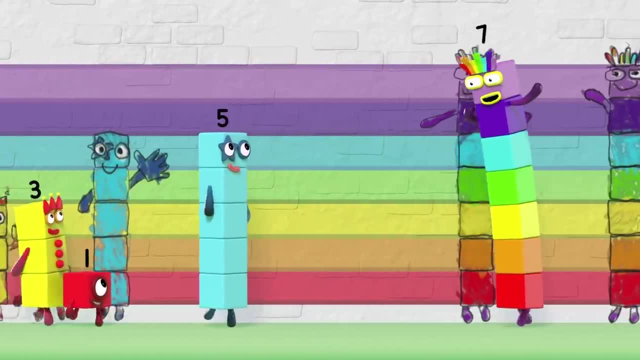 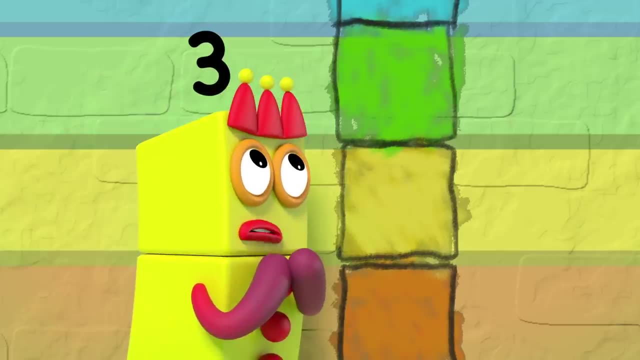 That's very easy to see. We're all friends here But we're different. But what makes you you and not me? I'd love to be you, But I come up short. I need to add something. But what? I'd love? to be lucky Like Seven. 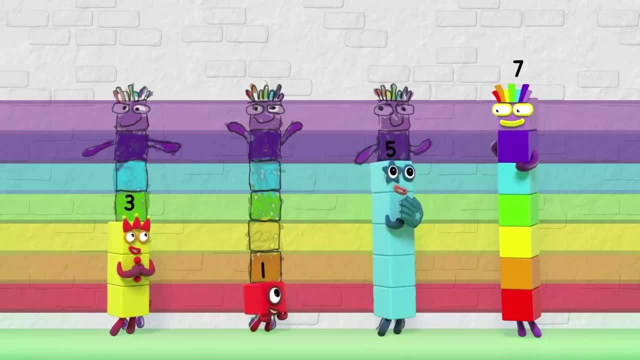 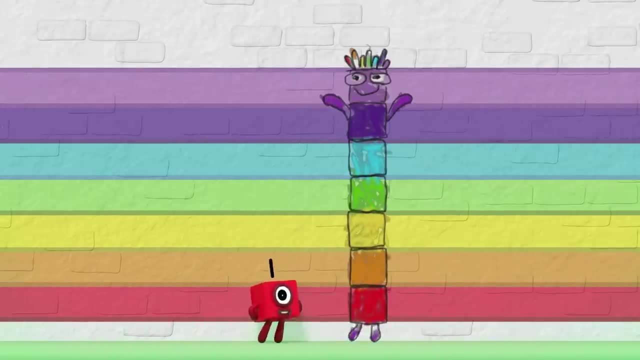 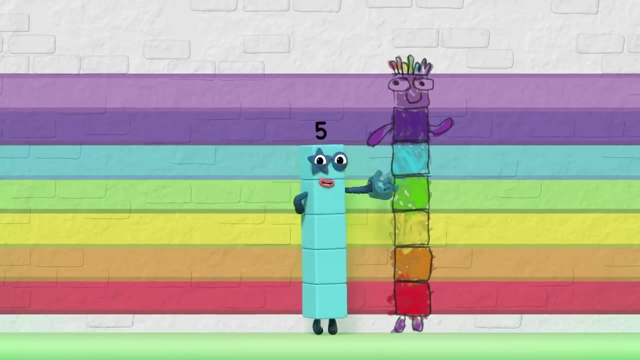 What have you got That we haven't got? I could try on a hat, That's the difference. Or I could stand on a box, That's the difference. And if the difference Won't pop into your head, You can count the missing blocks: One, two, two. 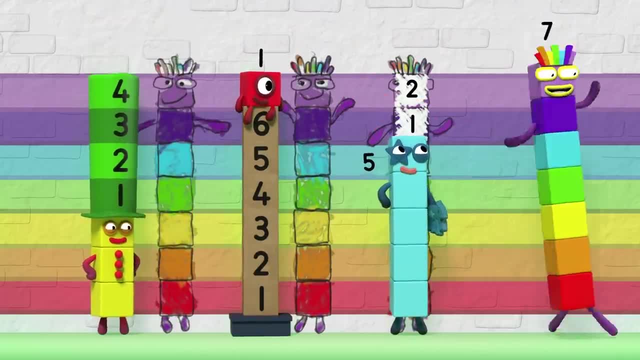 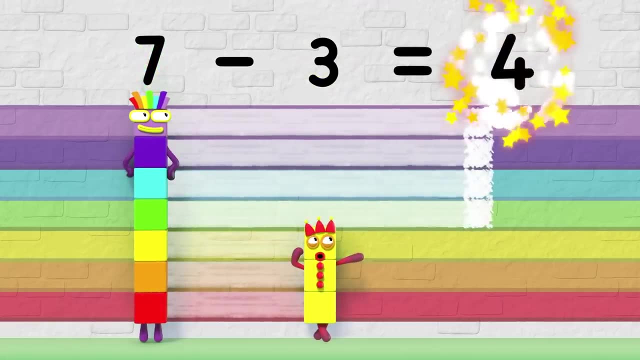 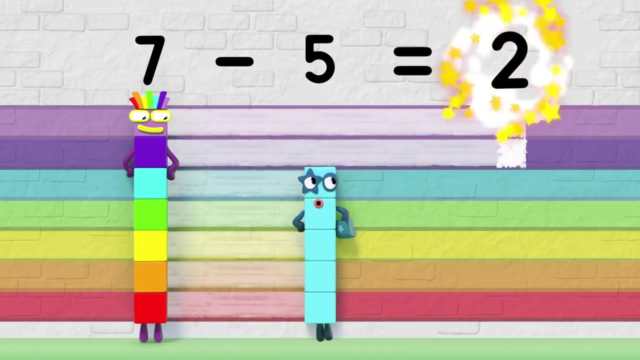 The difference is two. So what's the difference? Seven minus three equals four. That's the difference Four. Seven minus me equals six. That's the difference Six. Seven minus five equals two. That's the difference Six. So make up the difference And everyone will see What the difference is. 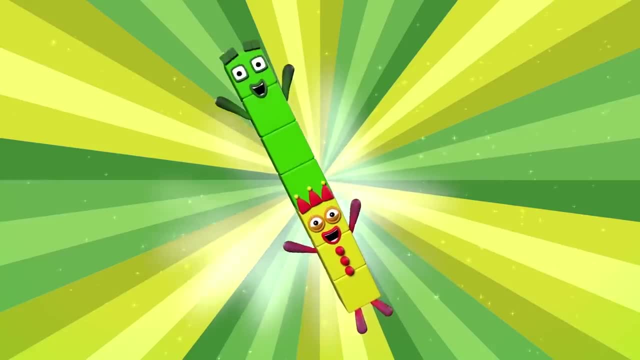 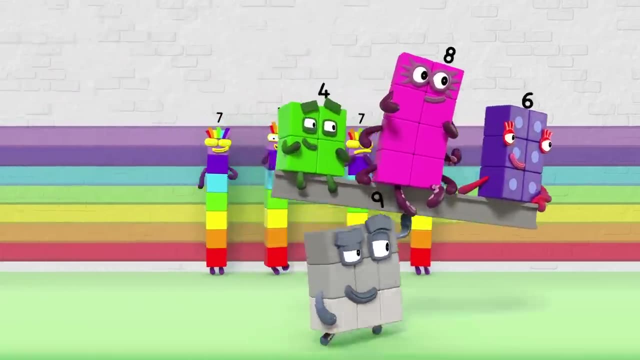 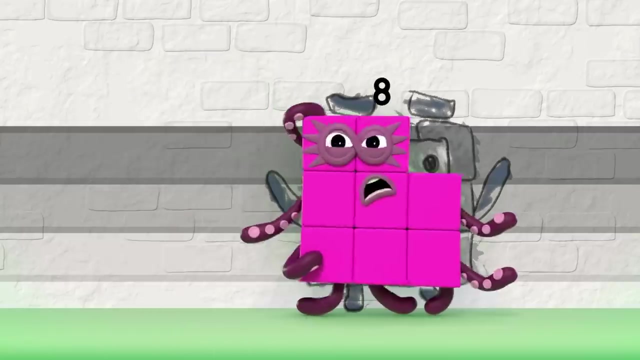 Between you and me: Ha-ha-ha, Ha-ha-ha, Ha-ha-ha, Ha-ha-ha, Ha-ha-ha. I'd love to be you, But I come up short. I need to add something, But what? 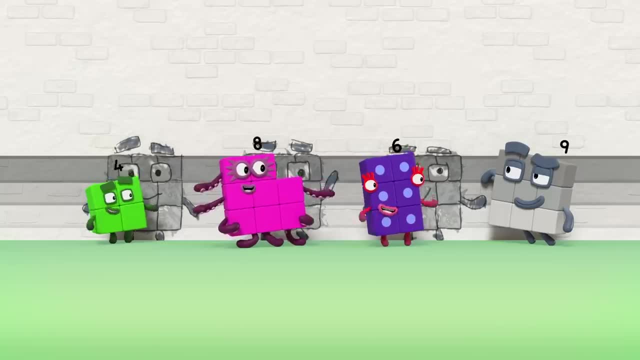 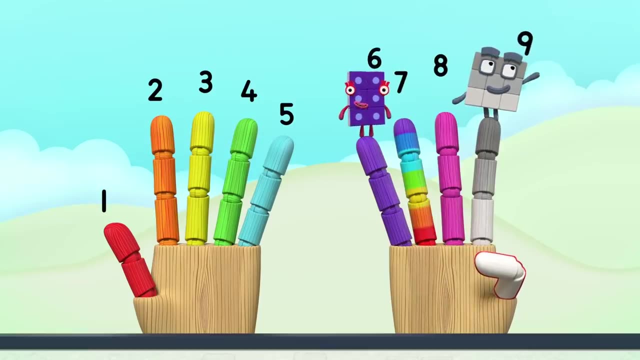 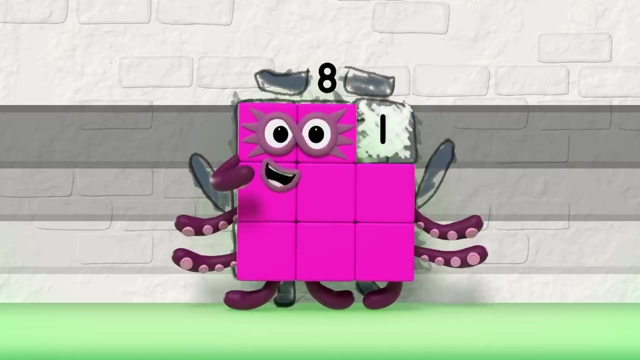 I'd love to be stronger, Like nine is: What have you got That we haven't got? You can count on your hands. Seven, eight, nine, That's the difference. Three, One, two, three. You can fill in the space. That's the difference. 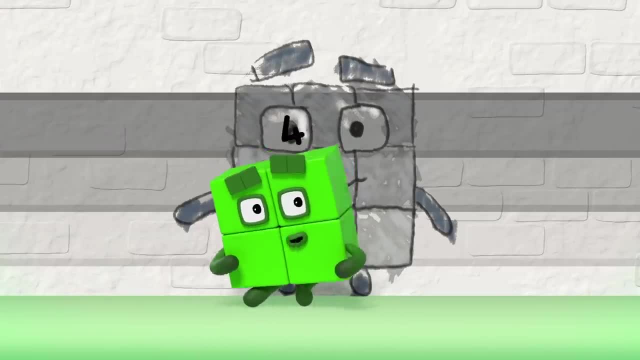 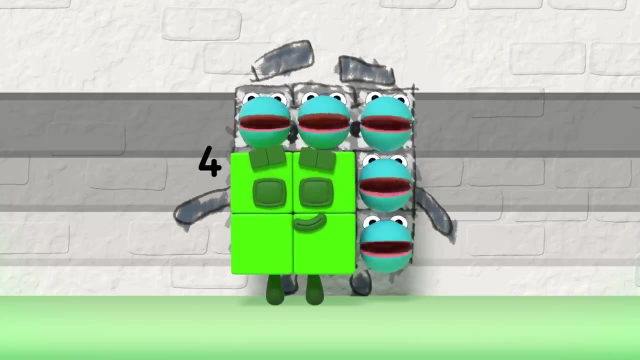 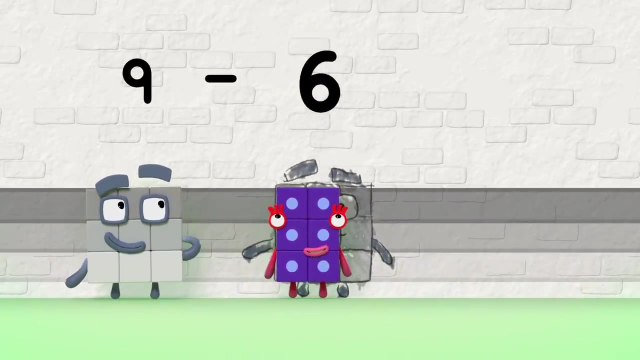 One, And if the difference Won't pop into your head, You can count, No, the gloves In place. One, two, three, four, five, Five. The difference is five. So Watch the difference. Nine minus six Equals three. That's the difference Three, Nine minus me. 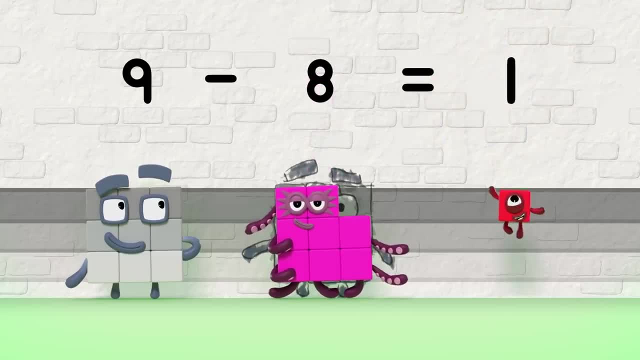 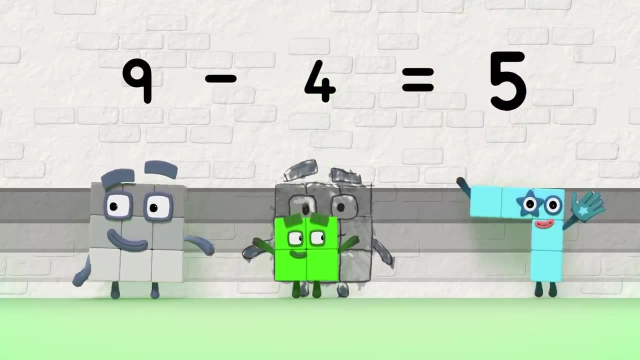 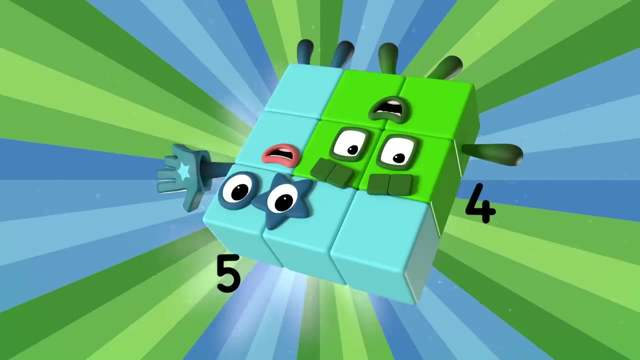 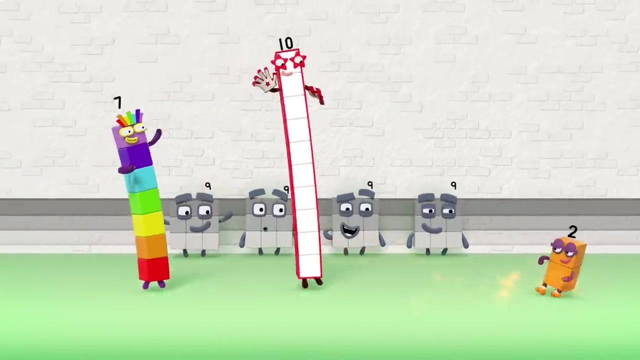 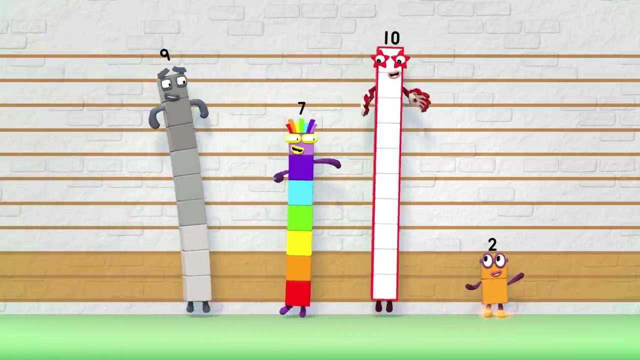 Equals one. That's the difference One. Nine minus four Equals five. That's the difference Five. So make up the difference And everyone will see What the difference is Between you and me. I'd love to be you, But I'm much too big. We need to lose something. 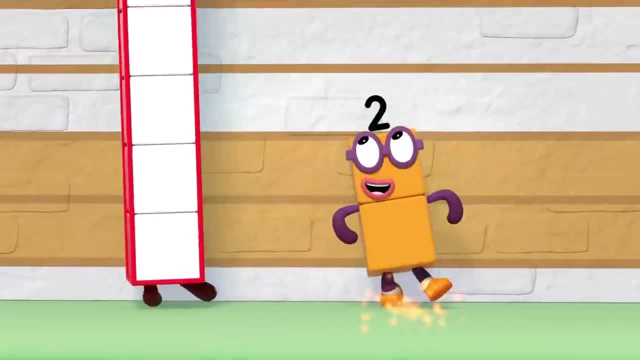 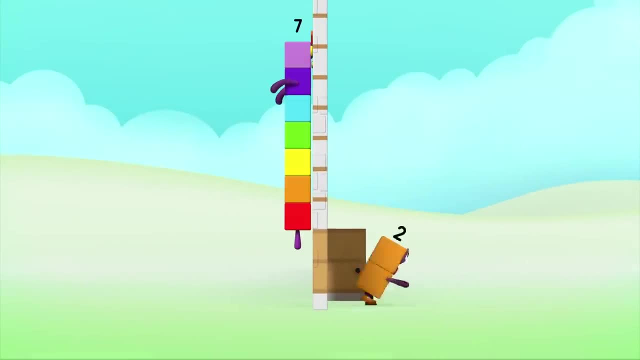 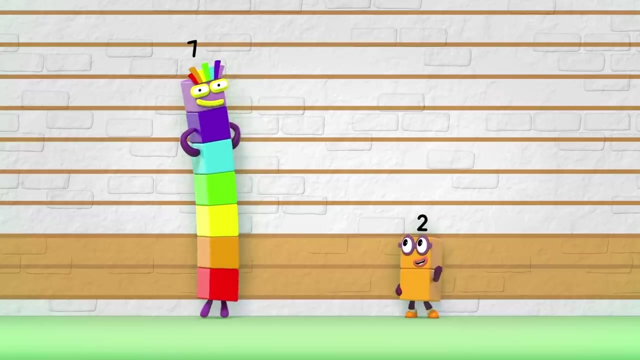 But what I'd love to have some of your talent. One makes you two, And some of we're not. I can walk through a door- Oh, That's the difference. Seven. I could get into bed- Oh, That's the difference. Eight. And if the numbers 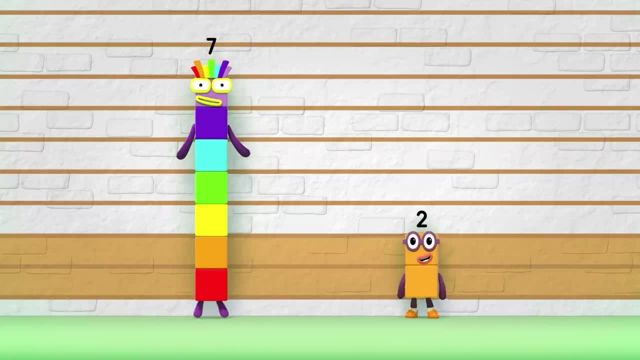 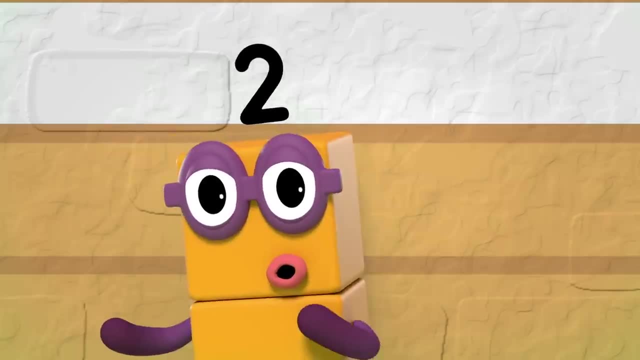 Won't pop into your head. You can count the extra blocks instead: One, two, three, four, five, Five. The difference is Five. So what's the difference? Nine minus two Equals seven. That's the difference. Seven Nine minus two. 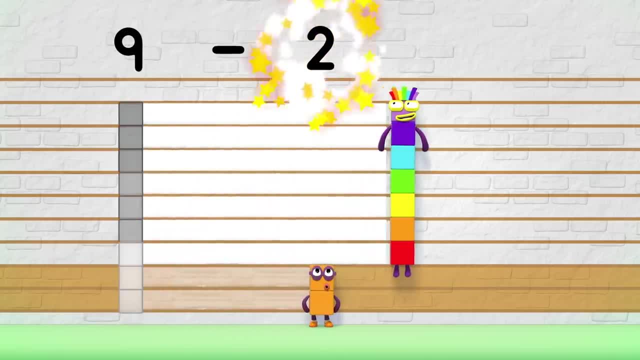 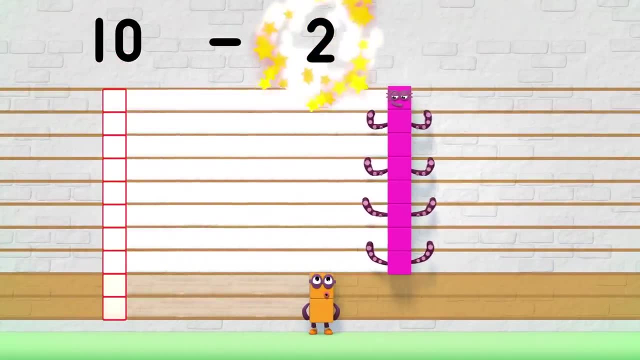 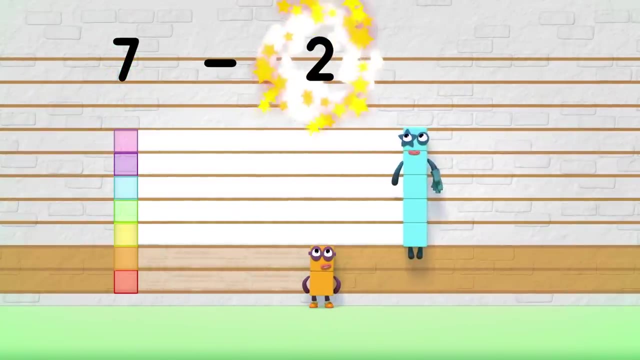 Equals seven. That's the difference. Seven Nine minus two Equals seven. That's the difference Seven. Ten minus two. Ten minus two Equals eight. That's the difference. Eight, That's the difference Eight. Seven Minus two Minus two Equals five. That's the difference. 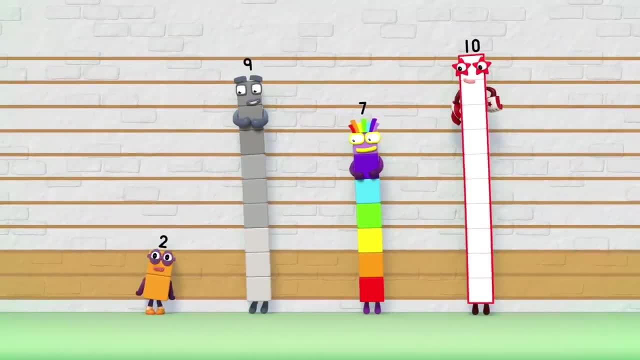 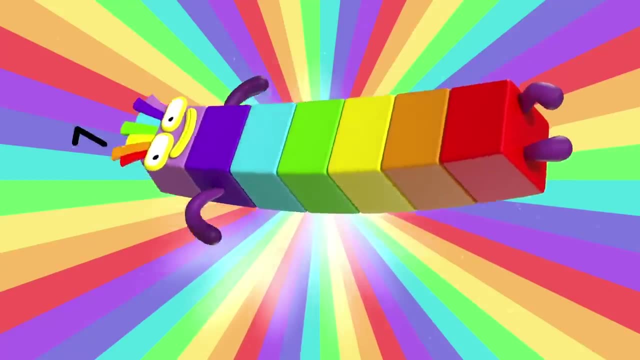 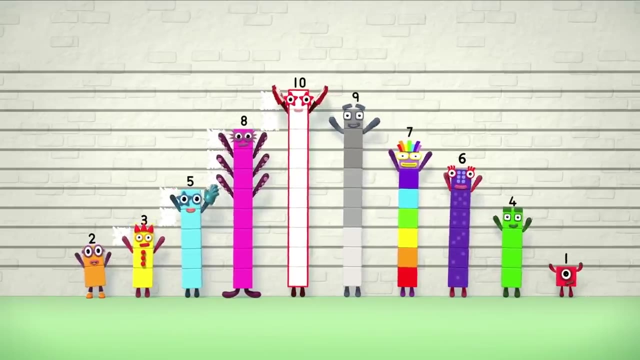 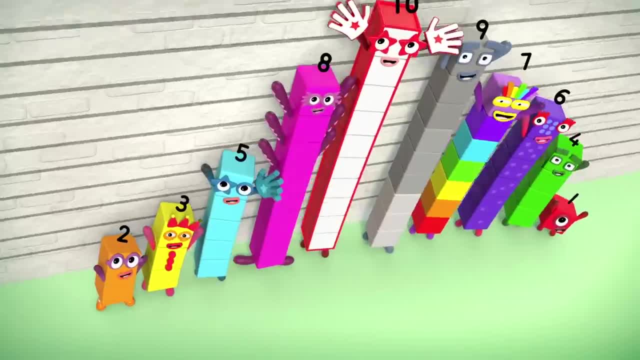 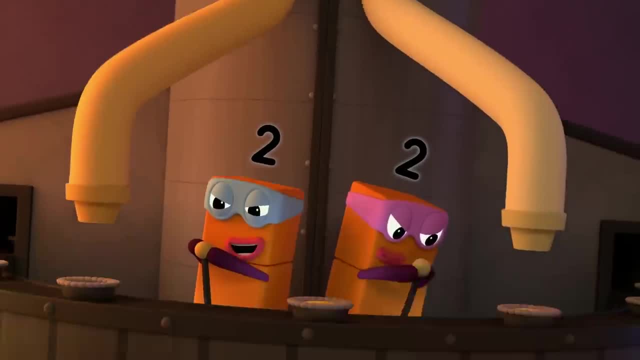 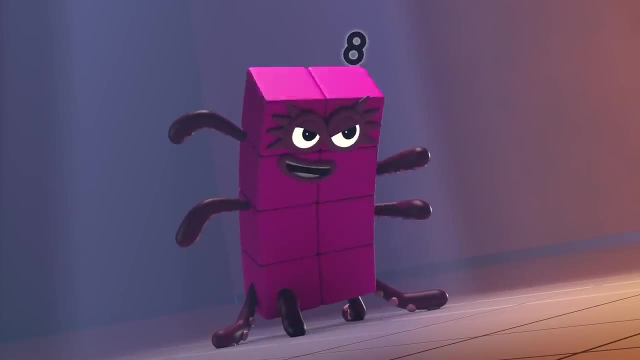 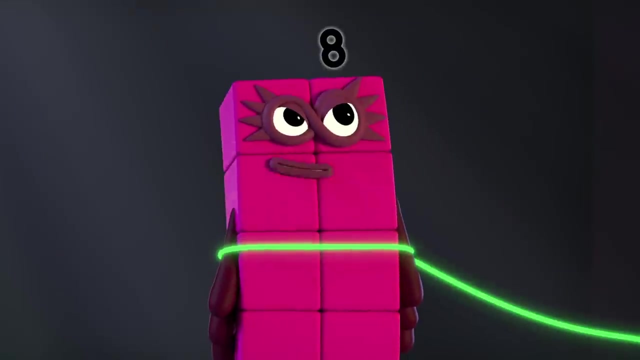 And the differences between us Make us who we are. Surprise, surprise, Custard pies, Your days of naughtiness are numbered terrible. twos, One, two, three Got you Octoblock break rope. That rope is made from pure octonite. 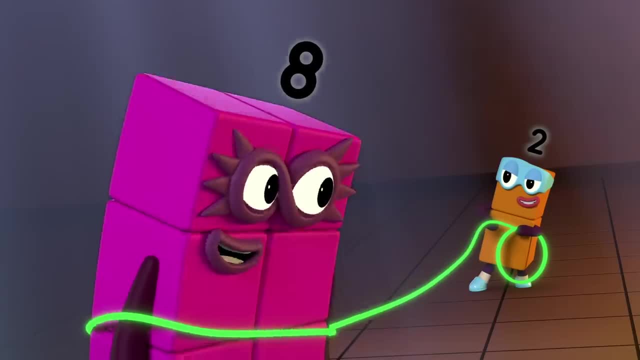 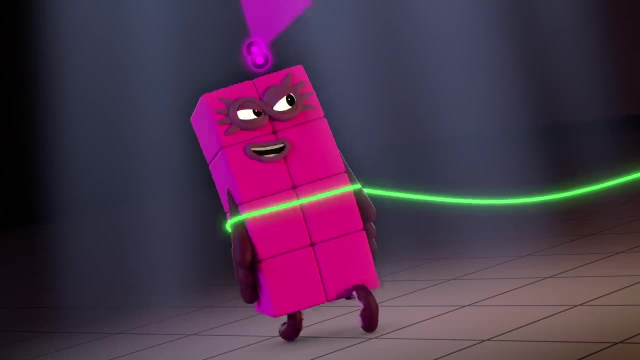 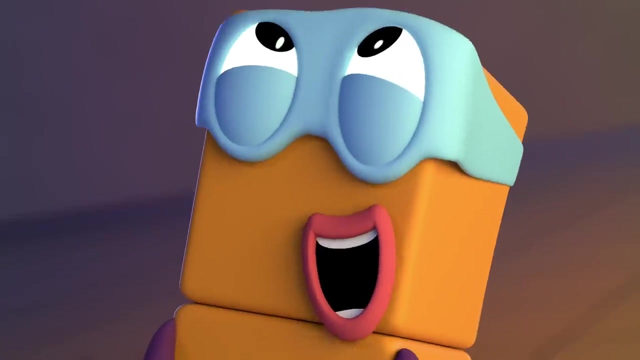 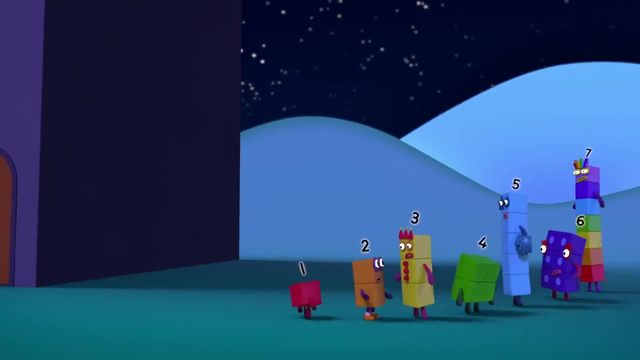 Your powers are useless? Maybe so, but I can still do this. The Octo-Signal: My friends will be here any moment And they will fall straight into our troublesome traps. Don't be so sure. Octoblock leads us Split up. 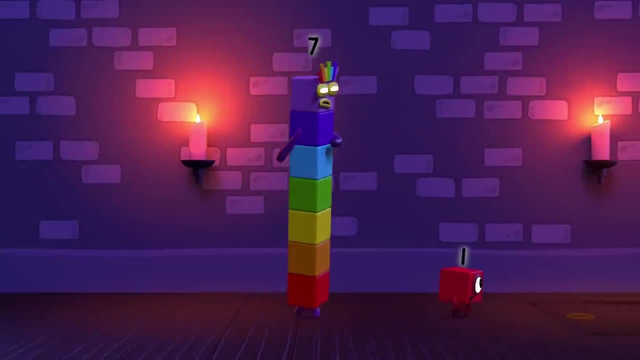 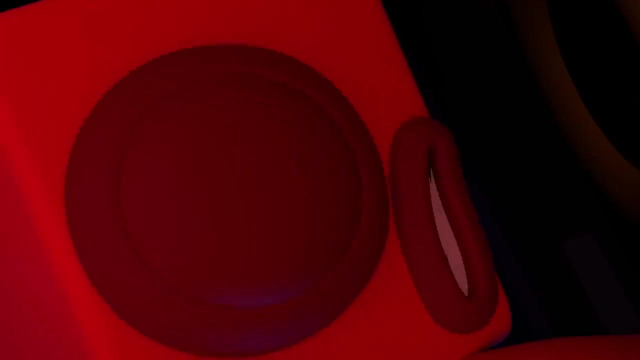 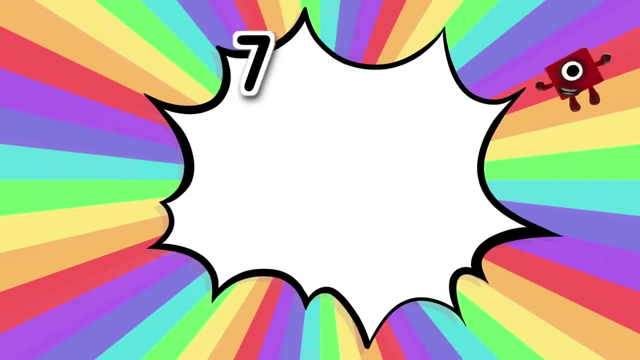 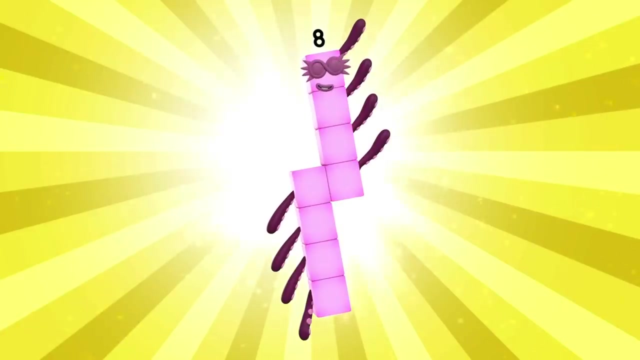 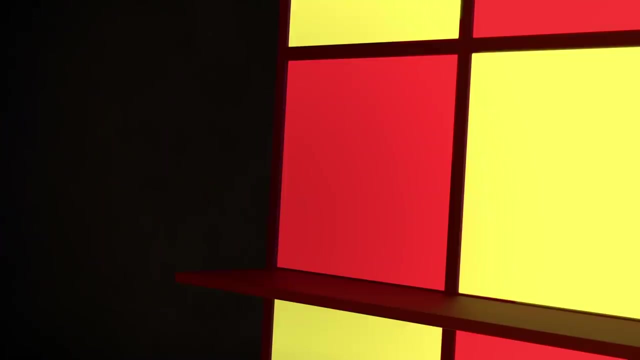 In here. That wasn't very lucky, But that was. Seven plus one equals Eight. Octoblock leap One, two, three, Four, five. Snakes and ladders- My favourite game. Ooh, Let's play together. Two, One, Two. 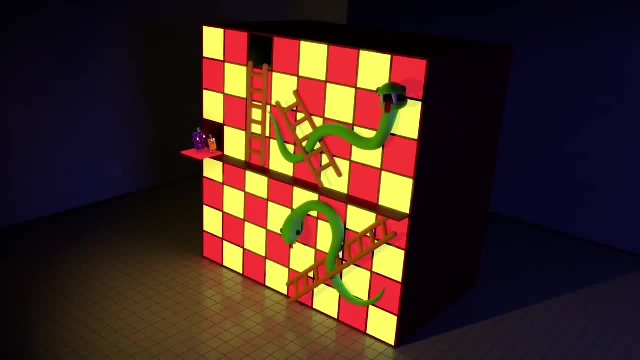 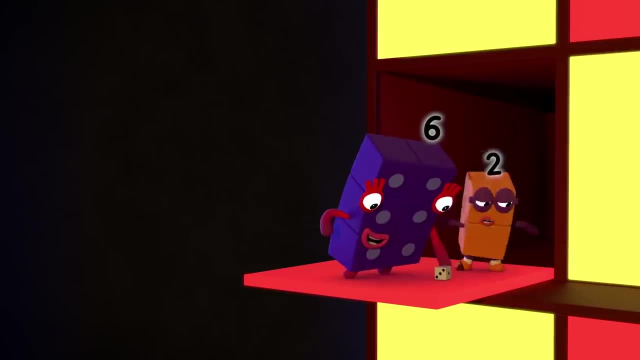 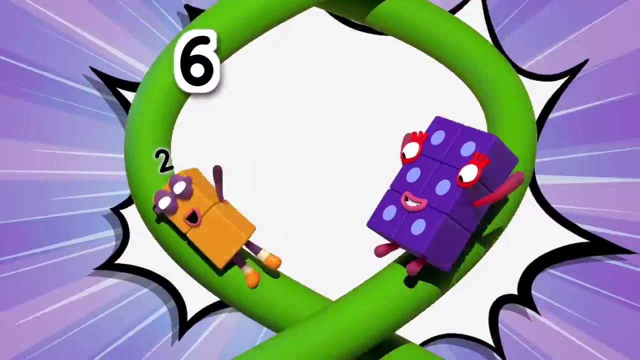 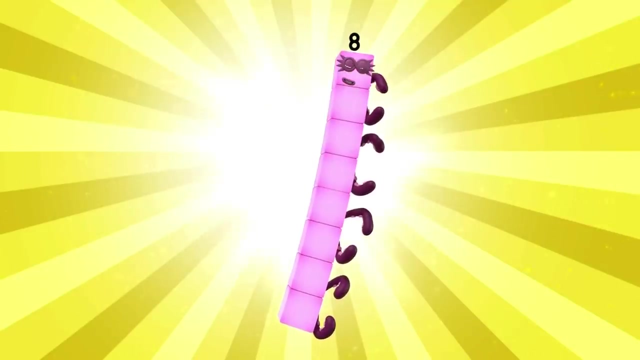 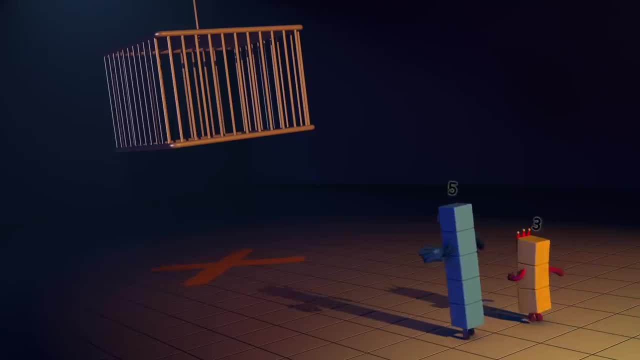 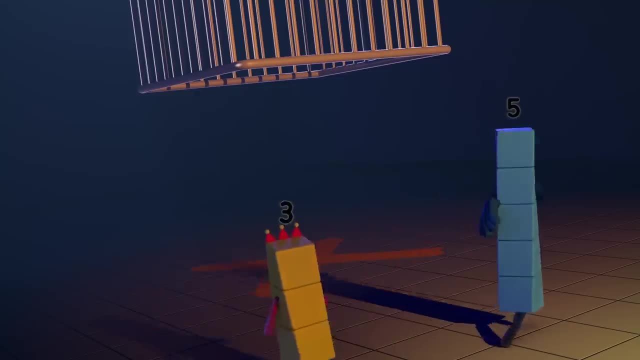 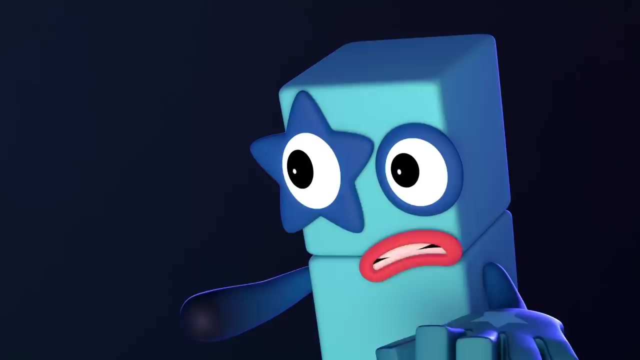 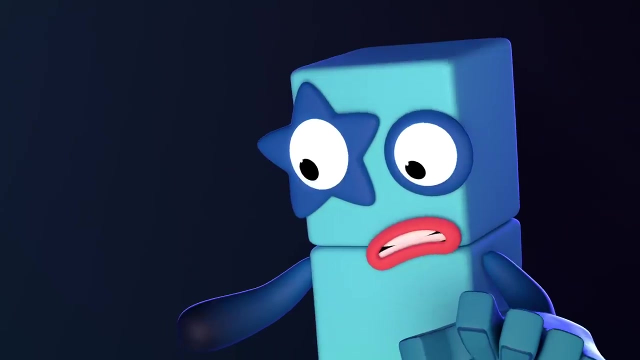 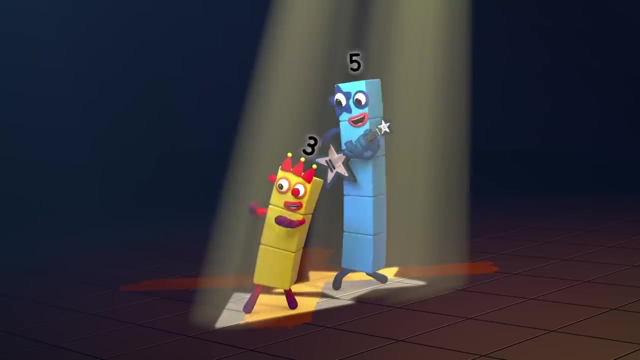 Don't walk under the cage. I could just resist it. I'm not going to let you get away with it. I'm not going to let you get away with it. Resist at three. I'm a star, I'm a star. 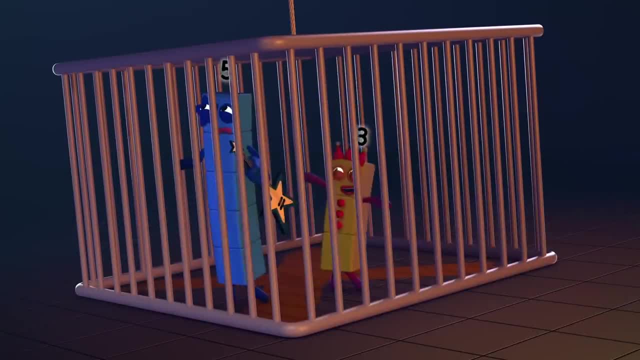 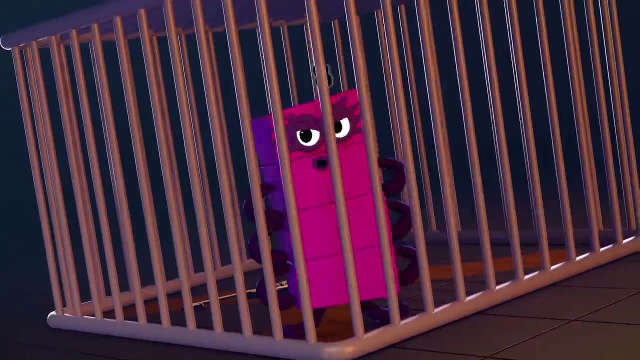 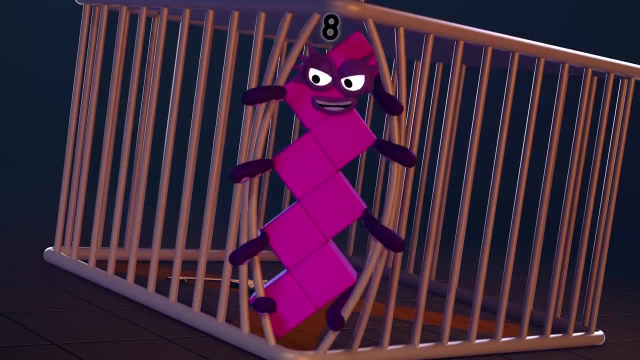 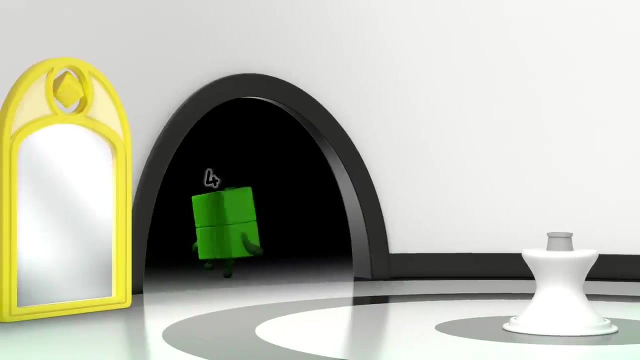 Hey, I wasn't finished. Grand finale. Five plus three equals Eight. Huh, Octoblock ten. One, two, three, four, five, six, seven, eight, Burn, Argh, Ah Oh. 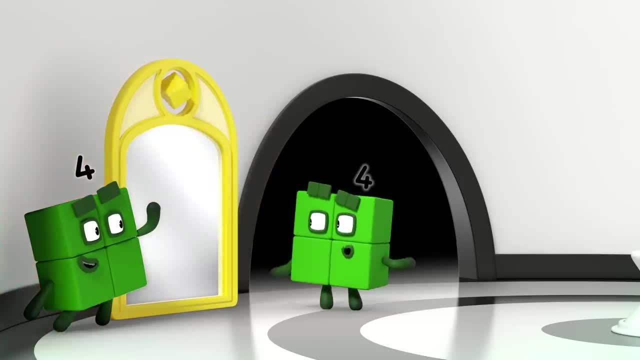 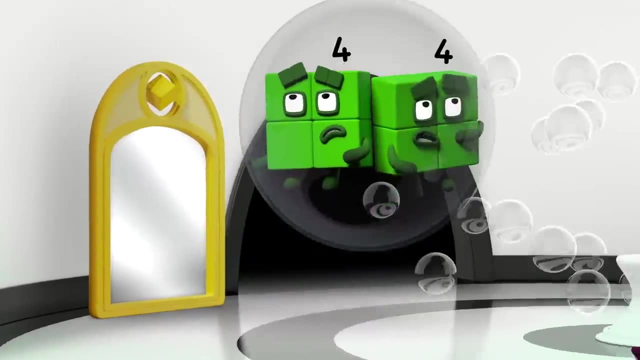 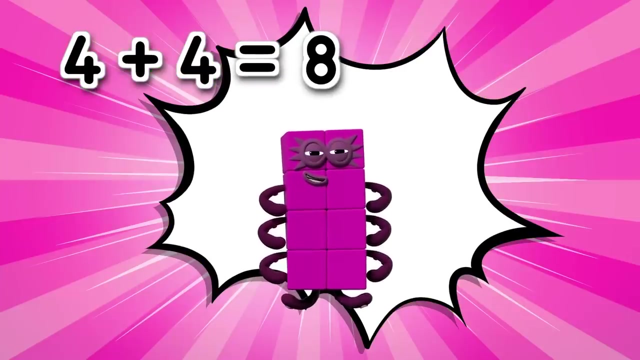 Ooh, Hello, Hello, Ooh, Round things It's got us. Ah, Four plus four equals Eight Octoblock pop. One, two, three, four, five, six, seven, eight Pop. 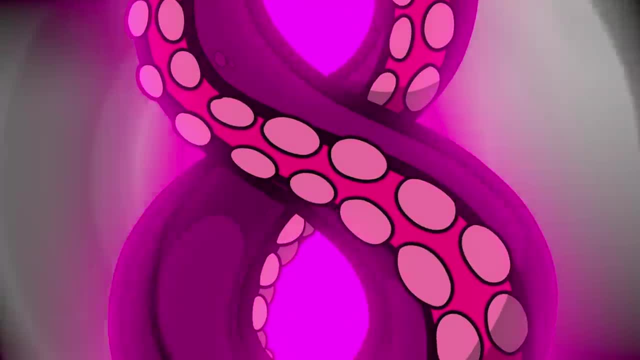 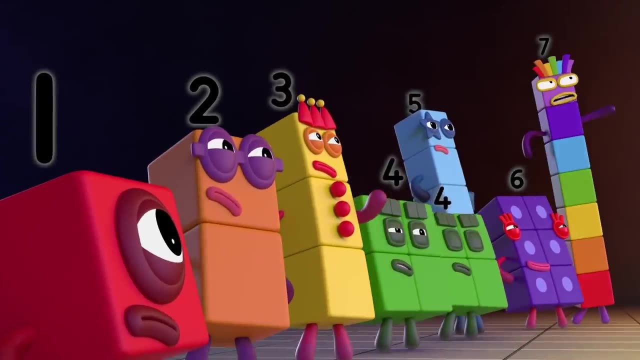 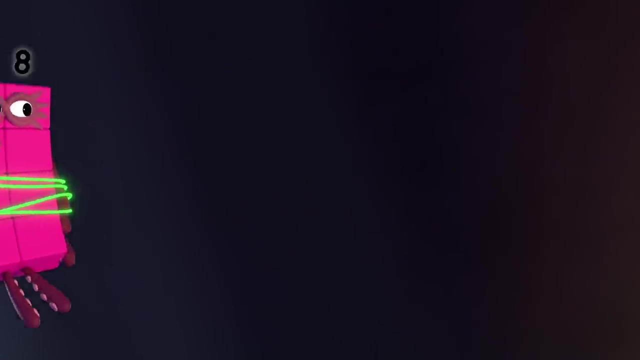 Hup, Prepare to be pied Spiderblock. Ha-ha, Stop right there. We have you outnumbered. Ooh, Ah-ah-ah, Ha-ha, Hup. Maybe so, But we've still got a trick or two. 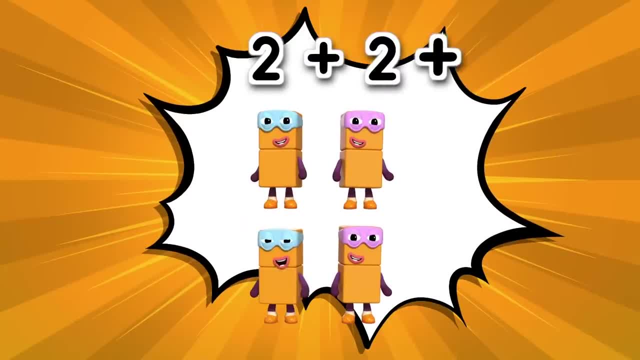 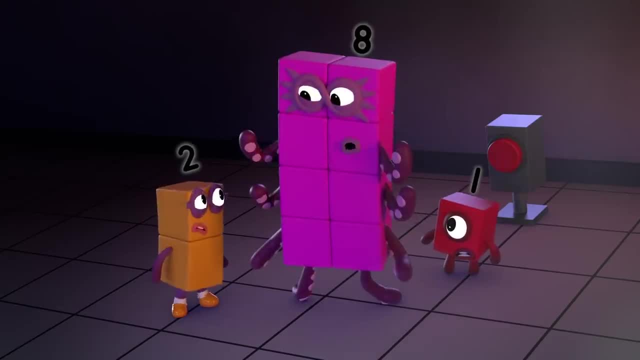 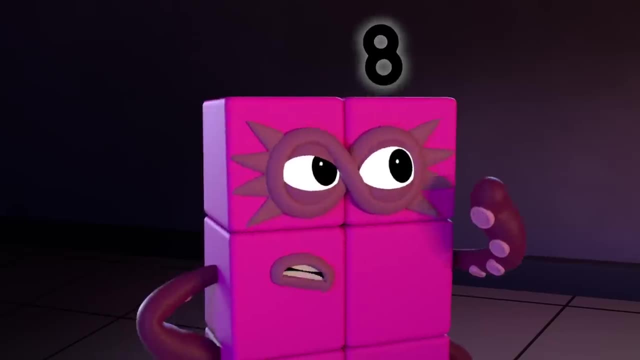 Let's see who's asleep. Two plus two plus two plus two equals eight. Oh, Four terrible twos make one Octonauty. You've met your match. Octoblock. Don't count on it. Octoblocks assemble. 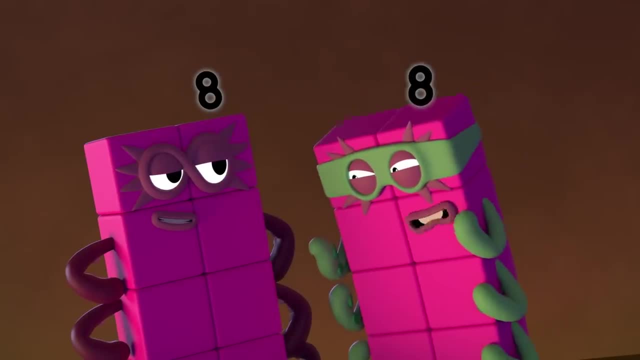 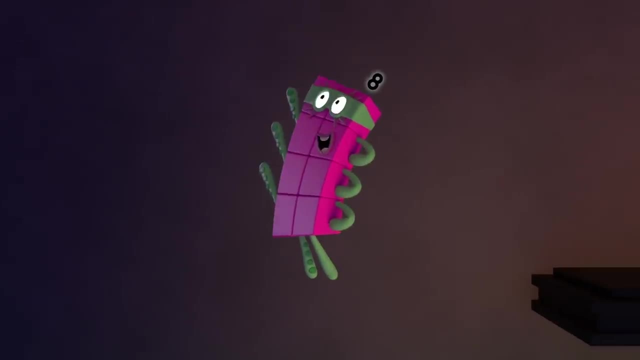 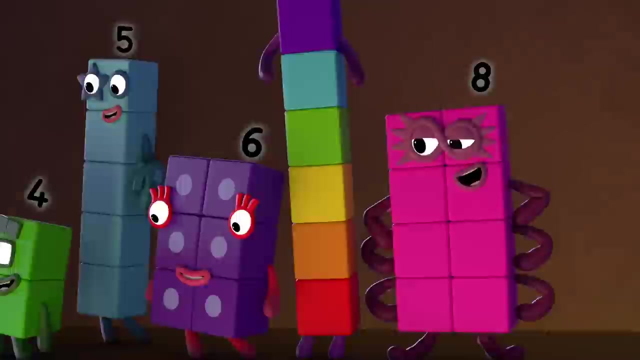 Your number is up, You'll have to catch me first. Octonauty escape, Ha-ha. Eight seven, six, five, four, three, two. one escape. Uh-oh, I spy with my little pie. a very naughty number block. 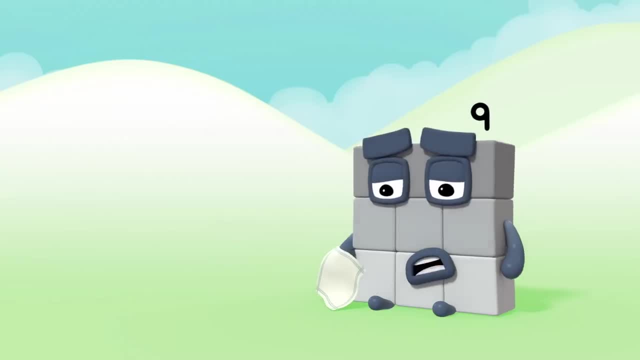 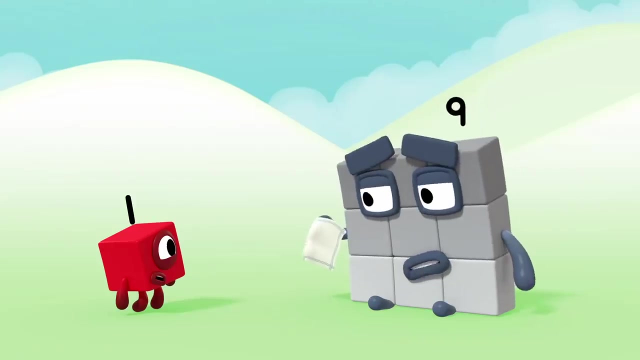 Ha-ha, Oh, Hello, Nine, What's the matter? One smaller, I always get one smaller. Huh, Every time I sneeze, I get one smaller. Achoo, Oh, Oh. 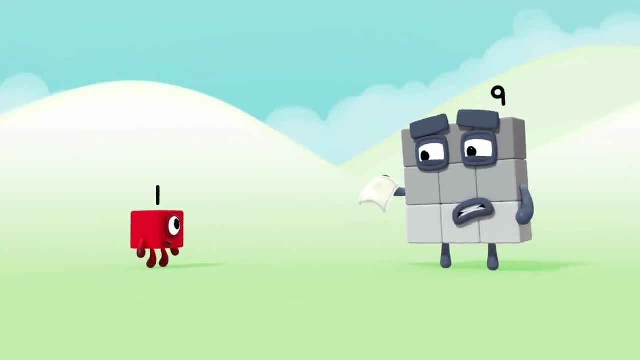 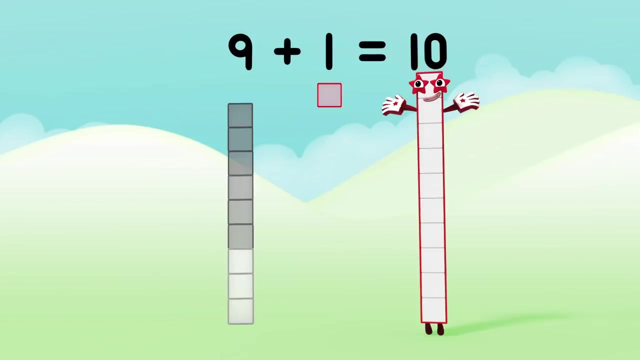 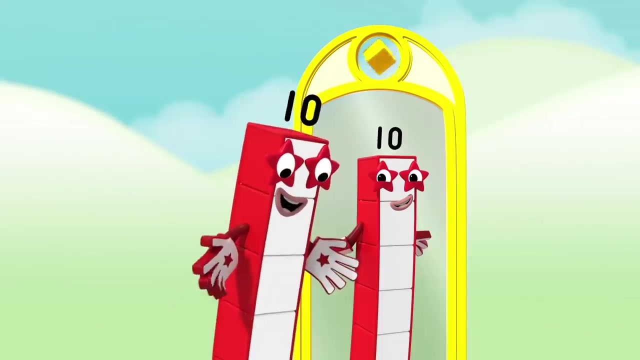 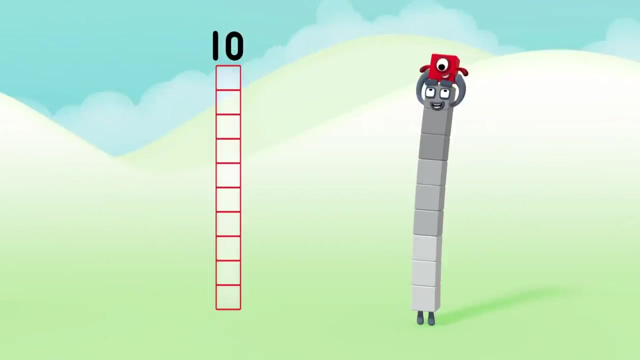 See Why can't I ever get one bigger. Maybe you can Stand tall. Nine Plus one equals ten. I am ten. Say it again: I am ten. Watch this. Ten minus one equals Nine, Oh. 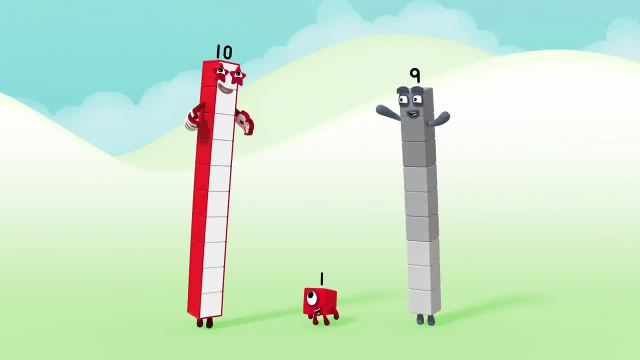 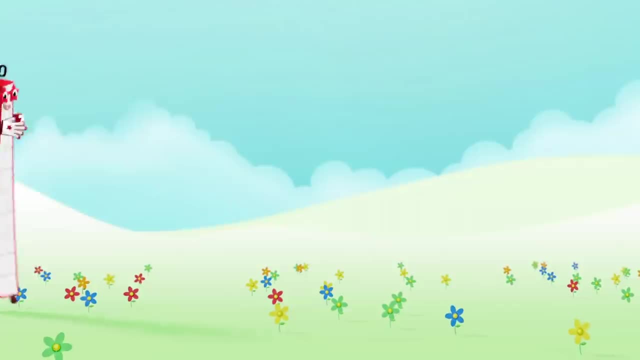 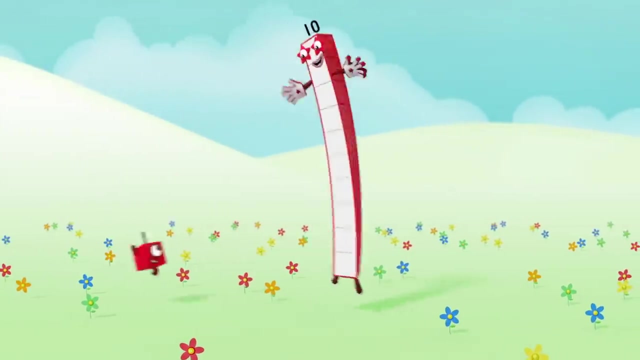 You're amazing. One bigger. You're one bigger. Why do you have a one on top? Huh, If you're wondering why there's a one on top, you'll know the answer when you realise: I'm one big block. I'm one big, perfect ten. 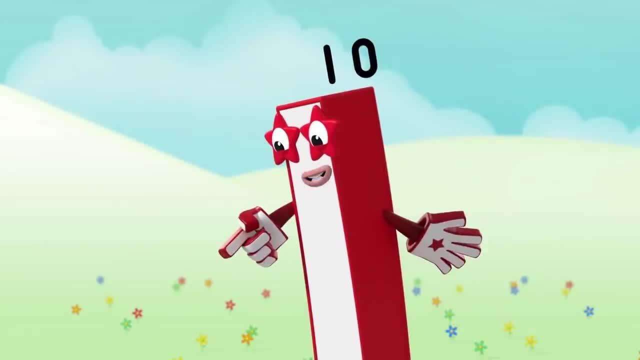 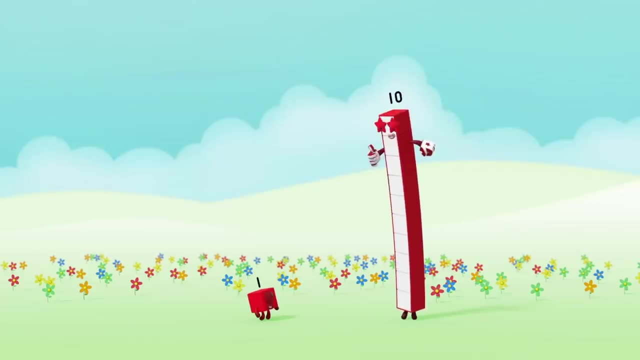 I'm a ten block, I'm a ten block. You might think we're different. think again. We're more alike than you suppose. You're one one And I'm ten And I'm ten ones, which means I'm one ten. 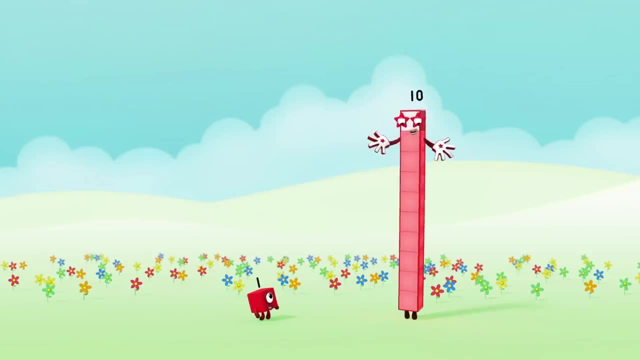 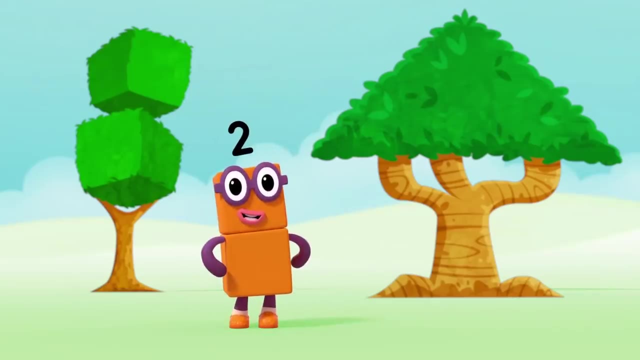 One, two, three, four, five, six, seven, eight, nine ten. Two is made of two blocks. I'll always be your friend. Three will entertain you. On what You can depend, I'm two ones. 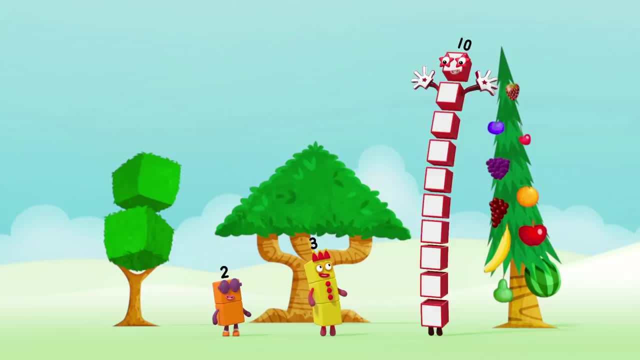 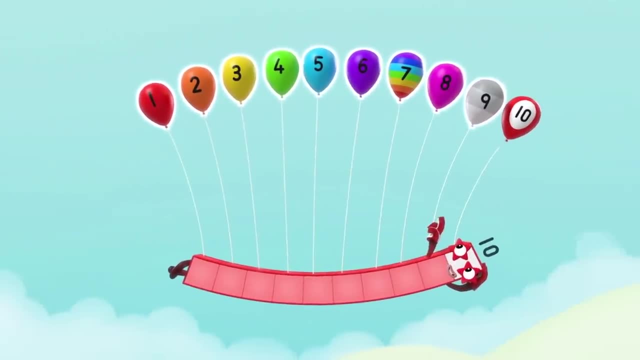 And I'm three ones And I'm ten ones, which means I'm one ten, I'm one ten. One, two, three, four, five, six, seven, eight, nine. ten Four is made of four blocks. 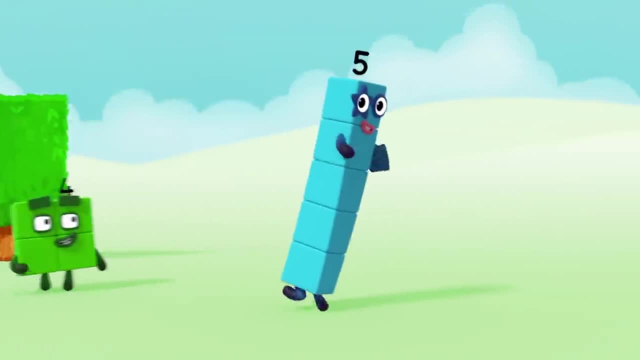 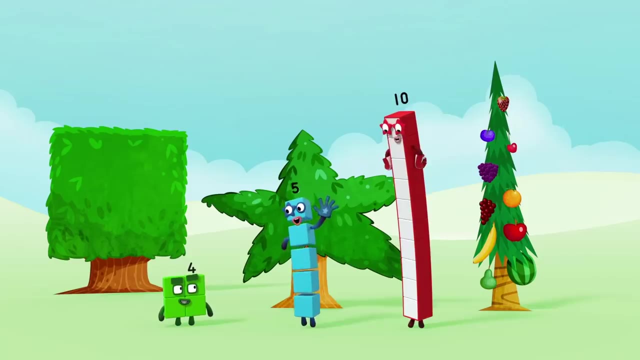 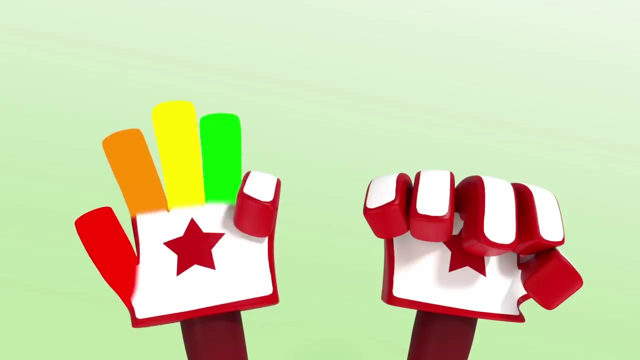 I love to be. a square Five is made of five blocks High five There. I'm there. I'm four ones And I'm five ones And I'm ten ones, which means I'm one, ten, One, two, three, four, five, six, seven, eight, nine, ten. 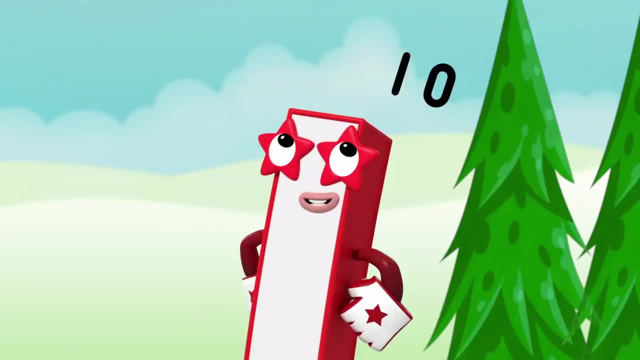 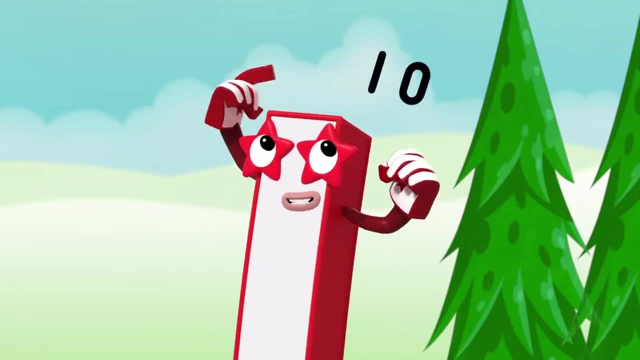 Oh, why have you got that round thing next to your one? It's a zero. I need my zero hovering in space. It's there to keep my one in place And if you're wondering what it's for, it shows you I'm not one. 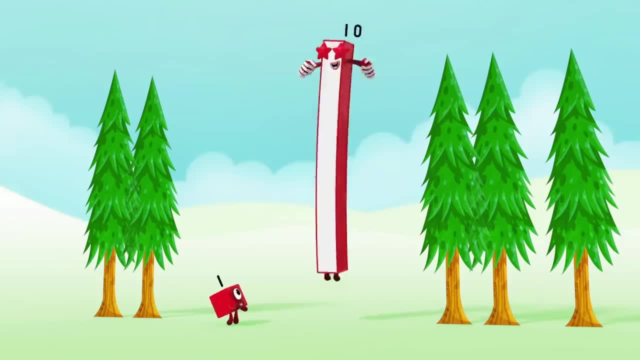 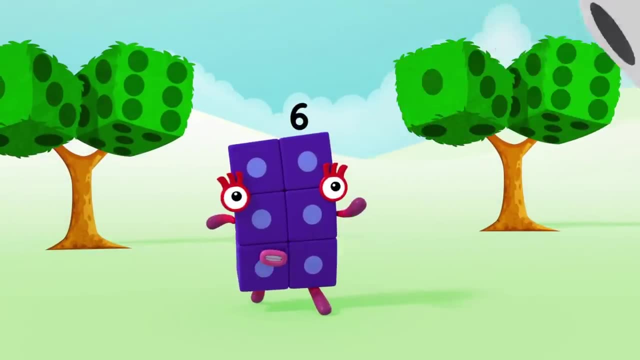 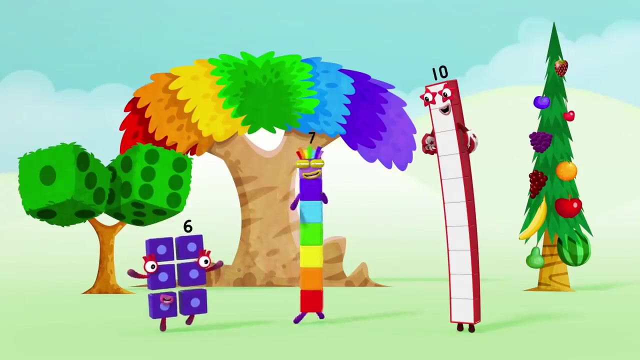 I'm one ten and nothing more. Six is made of six blocks. I like to roll the dice: Seven's made of seven. In a rainbow That looks nice. I'm six ones, I'm seven ones And I'm ten ones, which means 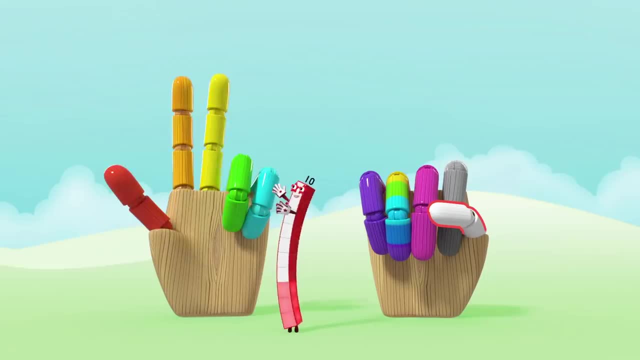 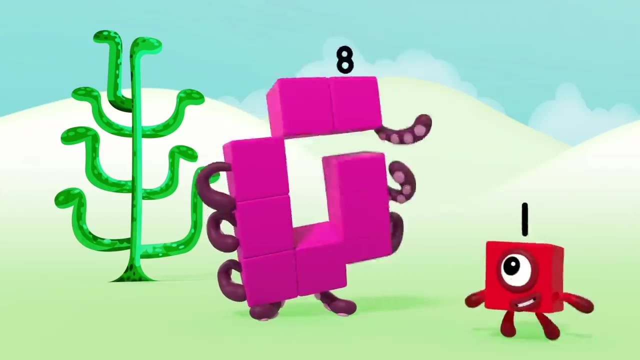 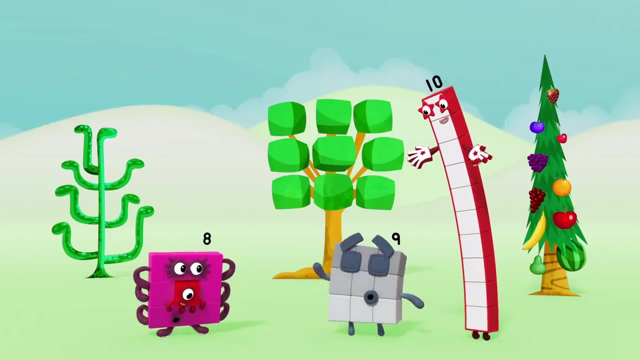 I'm one, ten, One, two, three, four, five, six, seven, eight, nine, ten Eight is made of Octoblocks And if you add one more, Nine is made of nine blocks. I'm a bigger square than four. 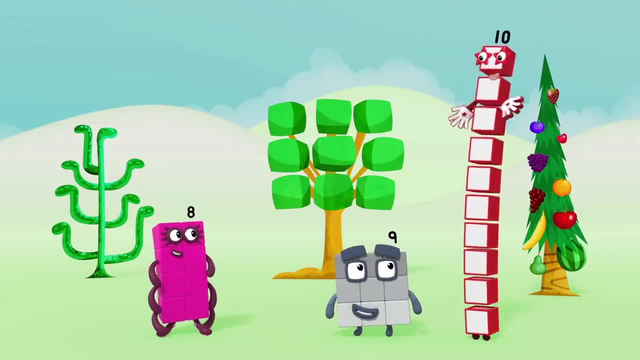 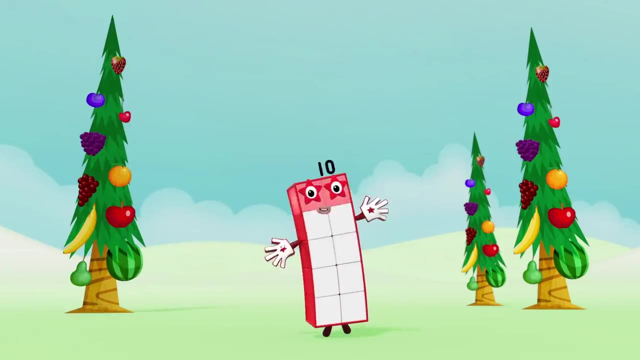 I'm eight ones And I'm nine ones And I'm ten ones, which means I'm one, ten, One, two, three, four, five, six, seven, eight, nine, ten. I can be two lots of five or five lots of two. 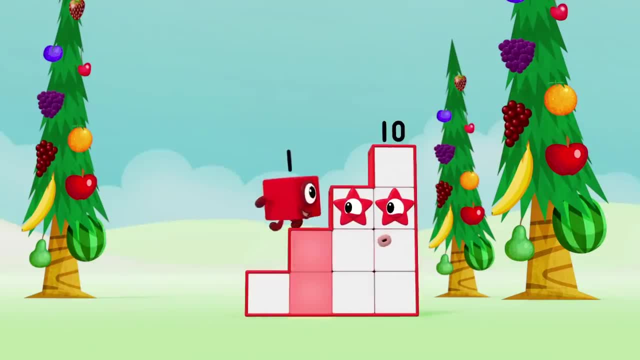 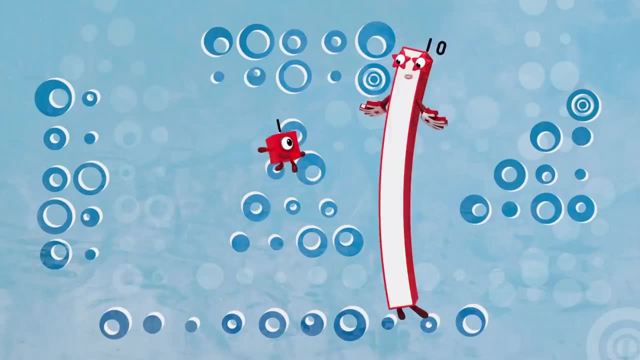 In other words, five pairs. I can be one and two and three and four. when you need to go upstairs, I'm a ten block. I'm a ten block. You might think we're different. Think again. They're all just made of counting blocks. 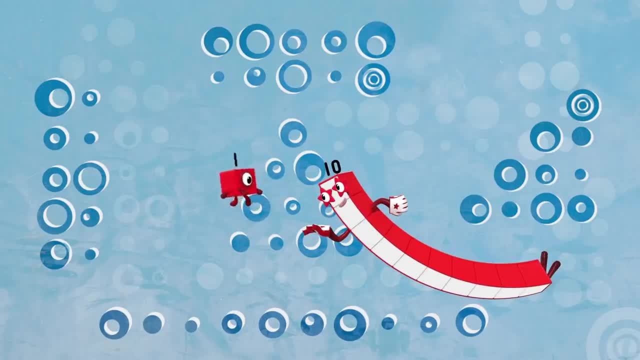 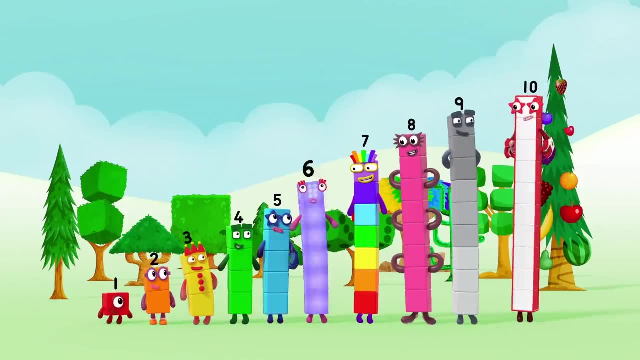 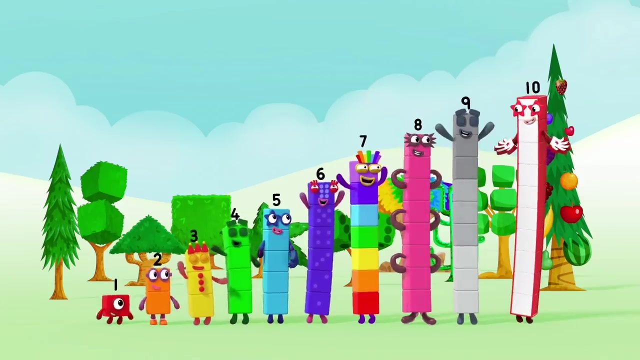 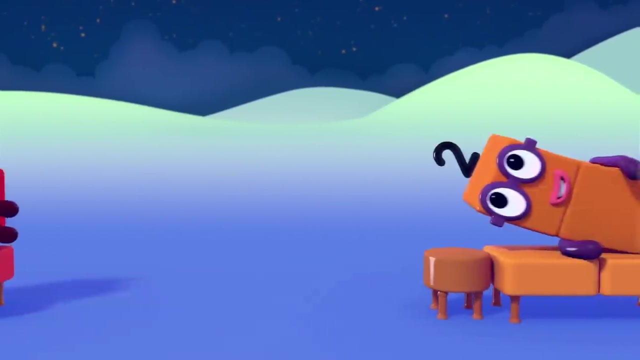 You're one one and you're ten ones, which means I'm one ten One. two, three, four, five, six, seven, eight, nine, ten Yay Hooray, Night-night, Night-night. 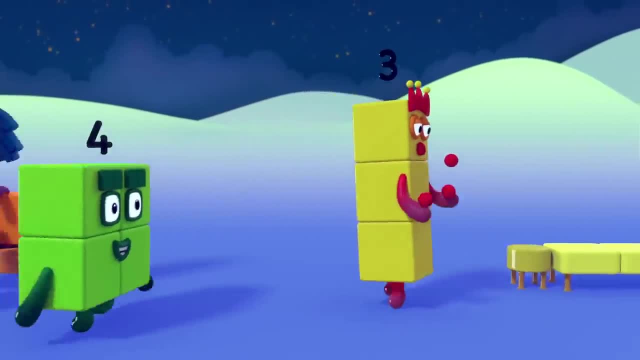 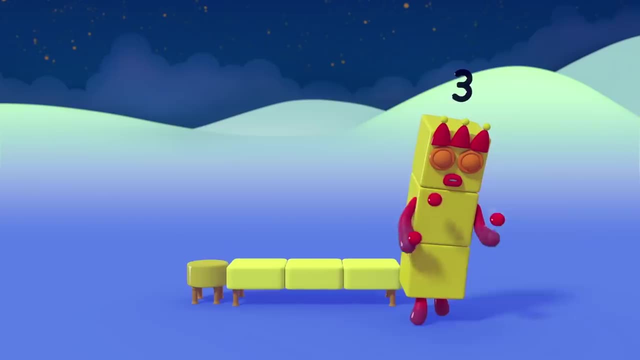 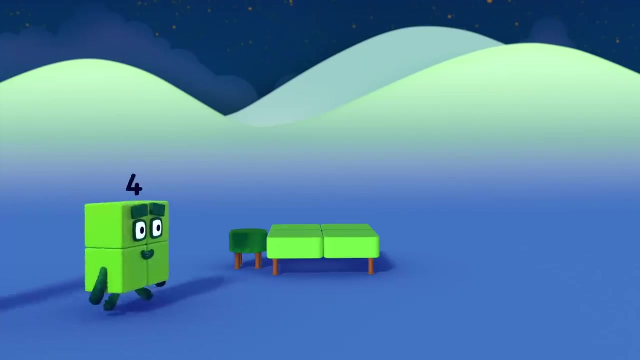 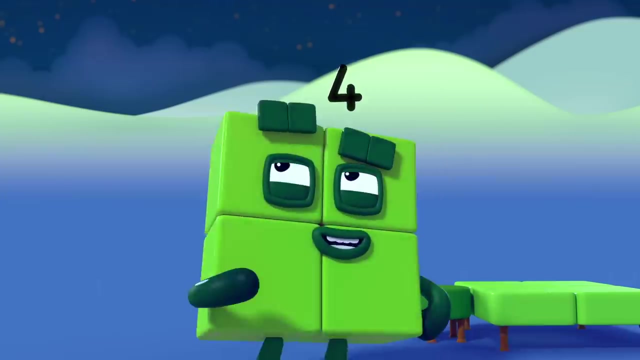 Sigh, Ah, tired, tired, tired, Sigh. It's time for bed, Boar, But I'm not tired. Stay up, go to bed. Make up your own mind, Sigh. Stay up or sleep. Stay up or sleep. 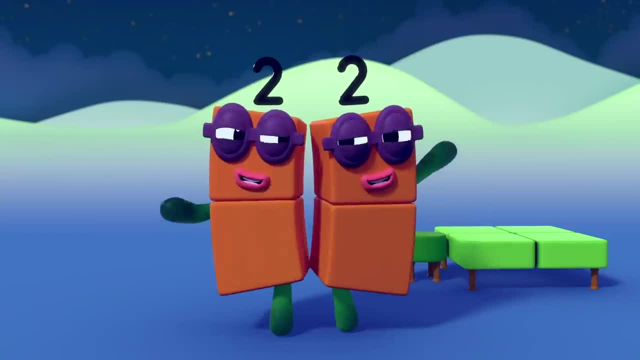 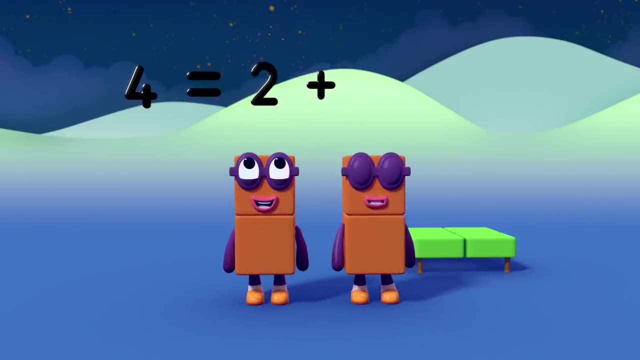 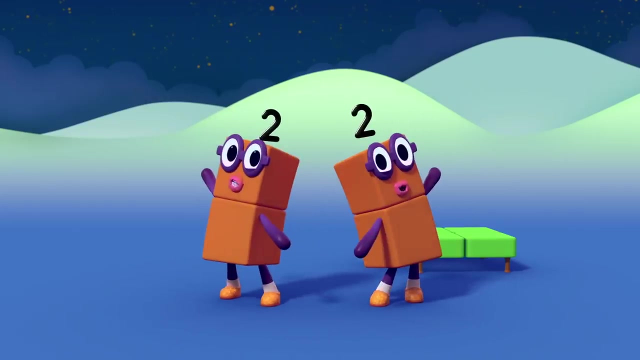 I can't do both. He can. No, no, no, no, Not you two. Four equals two plus two. You look like me, I look like you. We're two of a kind, We're the Terrible Twos. 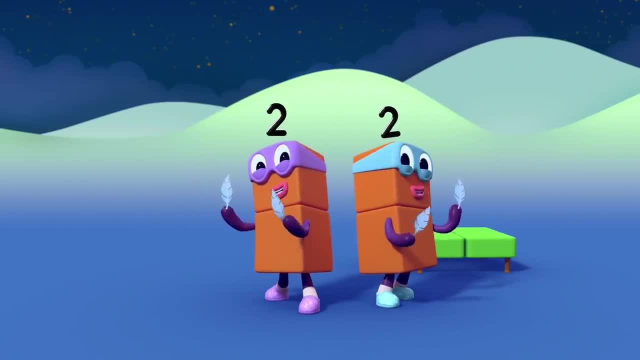 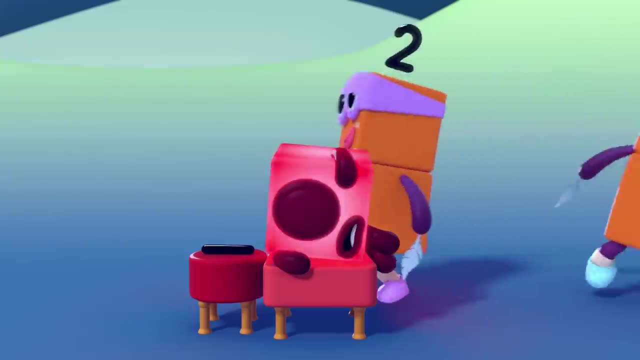 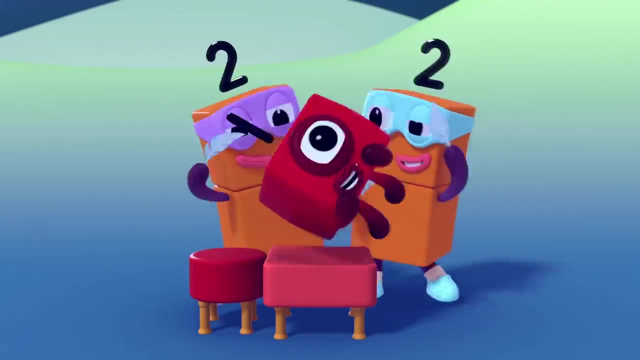 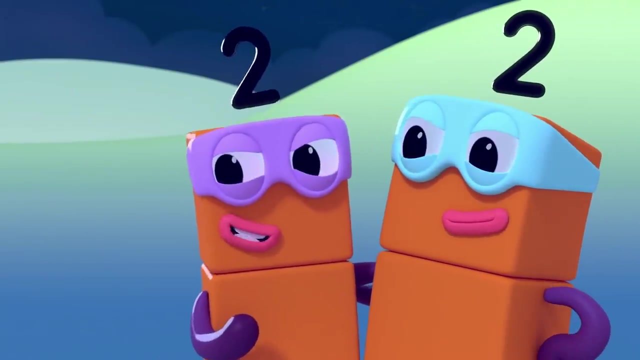 Yeah, Two feathers, It's tickling time. One, two, One, two, Tickle, tickle, Tickle, tickle. Oh, is someone there? Not someone, Some twos, And we're both here to say: 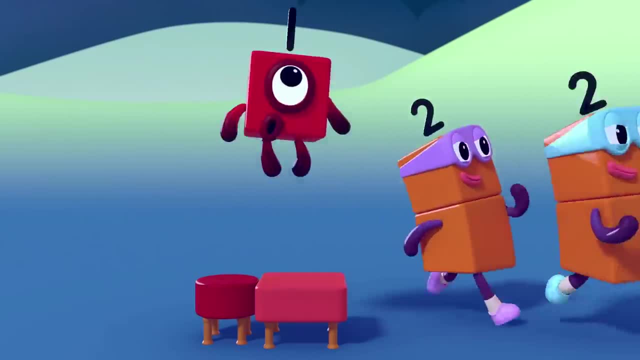 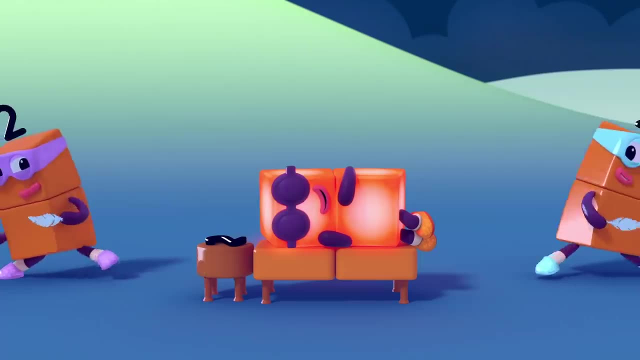 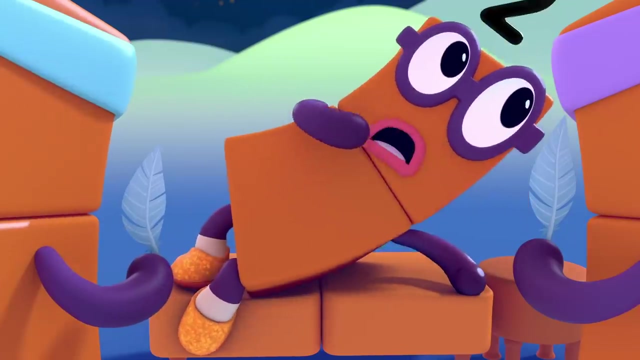 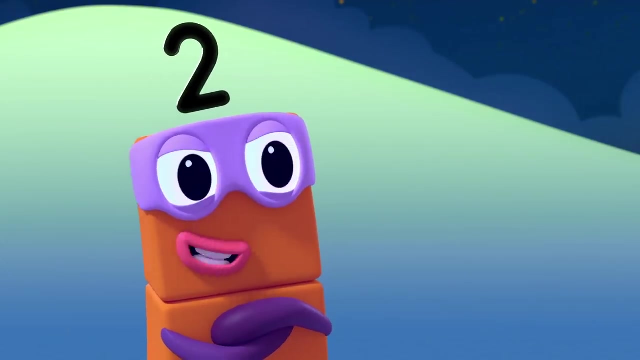 That was fun, Yeah Yeah, He reminds me of someone. Amigo, Can't think who. Amigo, Tickle, tickle, Tickle tickle. Another me, Doubler, Another another me, Him, me, and you are too many twos. 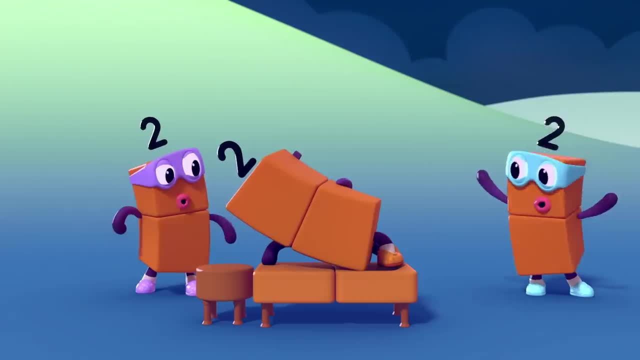 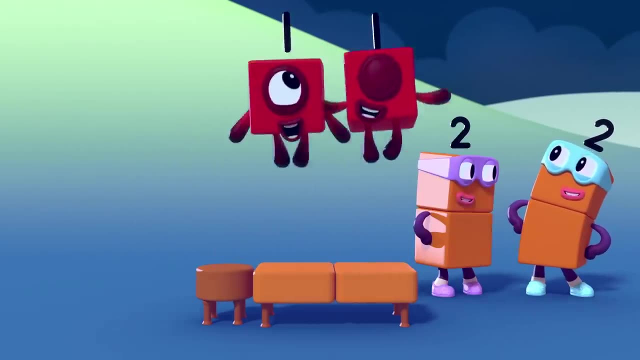 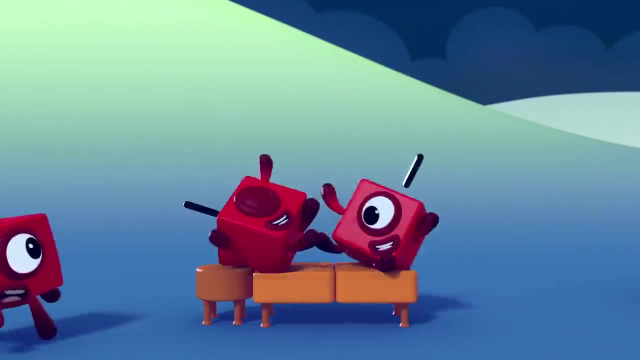 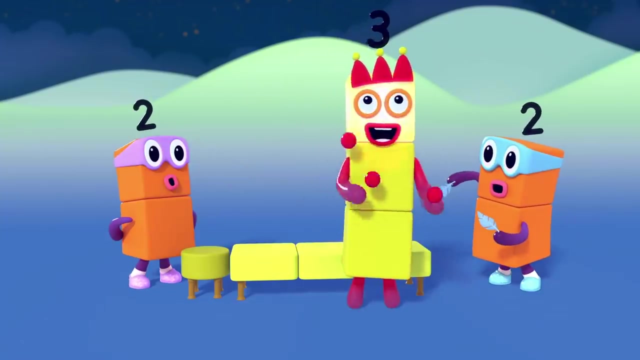 So it's time for the both of us to say: Boo, Ah, Boo, Two, twos, two ones. It's time to be gone. Yeah, Boo, Boo, Boo, One, two, Three. Looks like fun, Let's try it too. 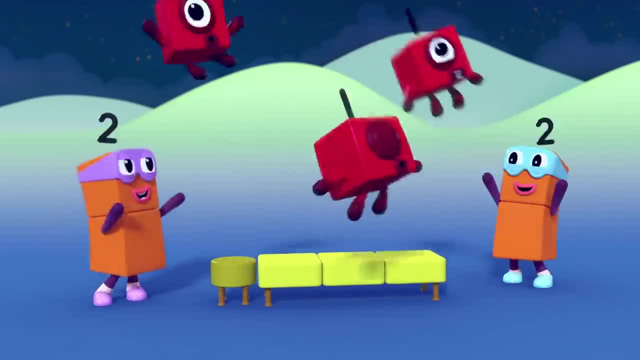 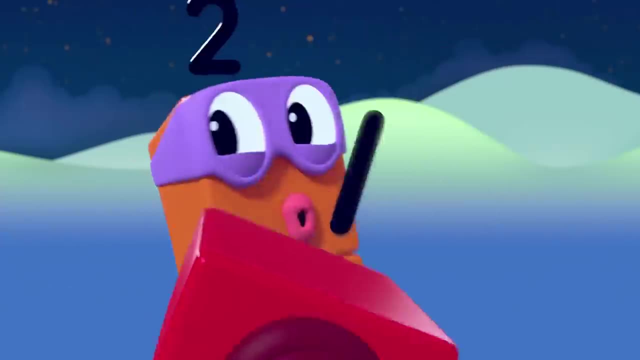 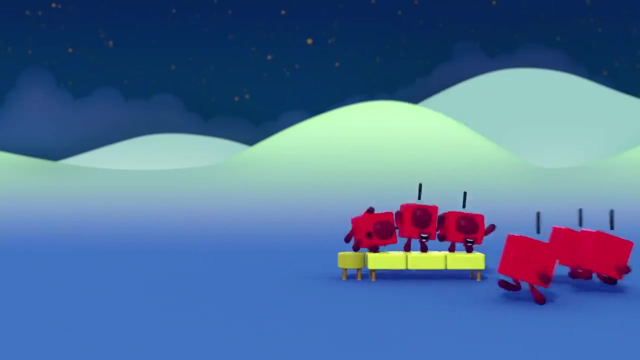 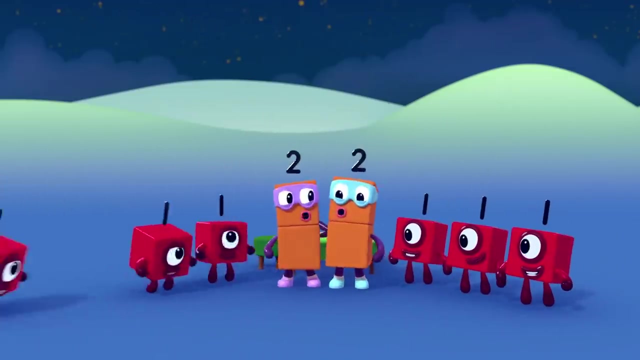 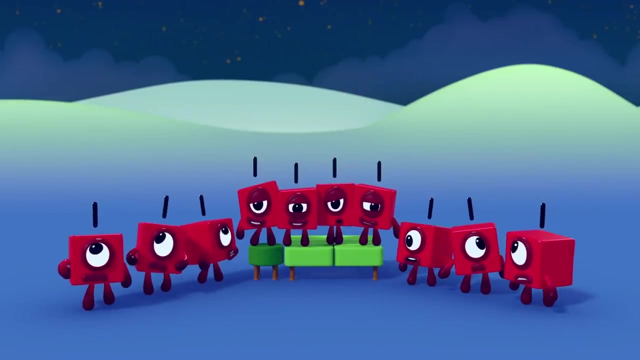 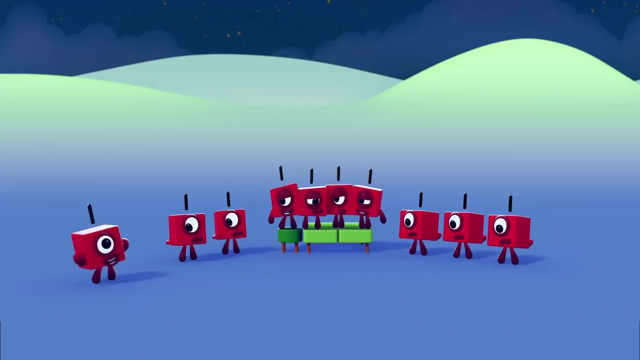 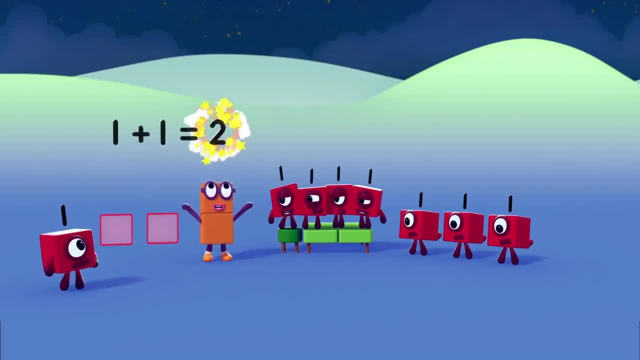 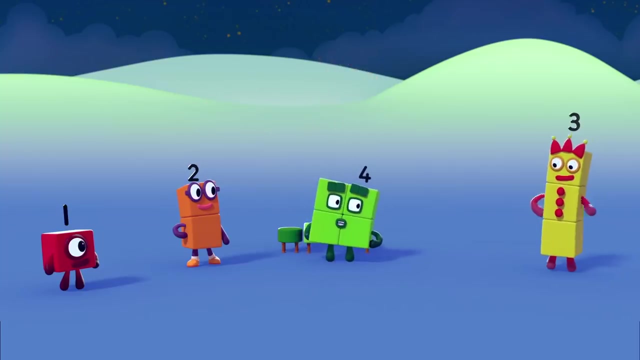 One plus one equals two. Two is two ones. One plus one plus one equals three. Three is three ones. One plus one plus one plus one equals four. Four is four ones. Where are they? Where did those terrible twos go? 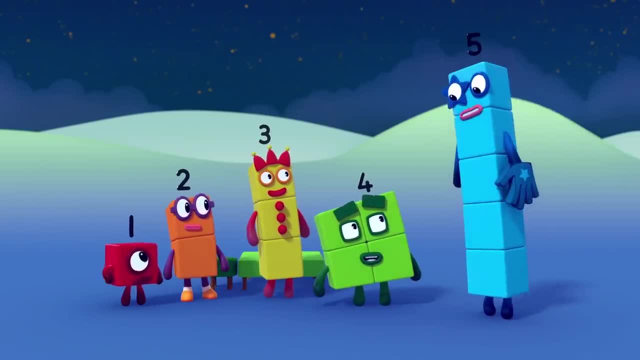 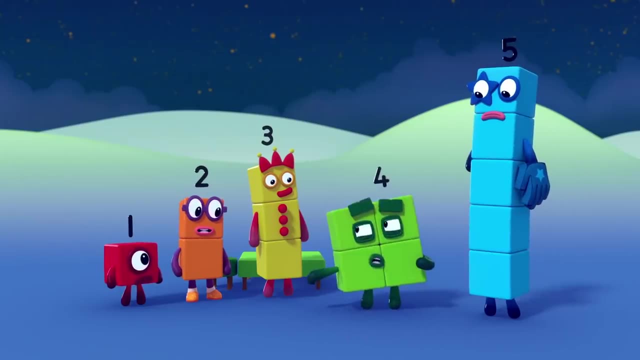 Don't look at me. What's all of the noise? The terrible twos are playing tricks on us, And where are they now? I have to be square with you. They made me. What did they make you? You can tell us, Spore. 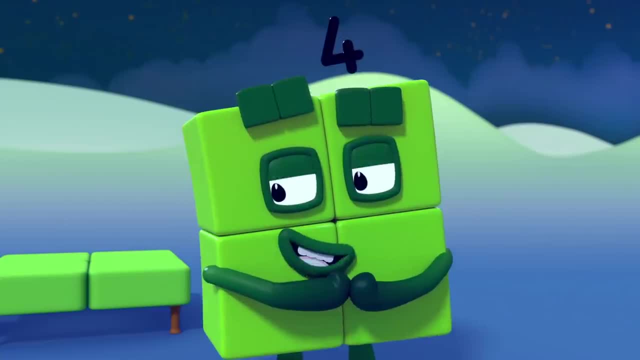 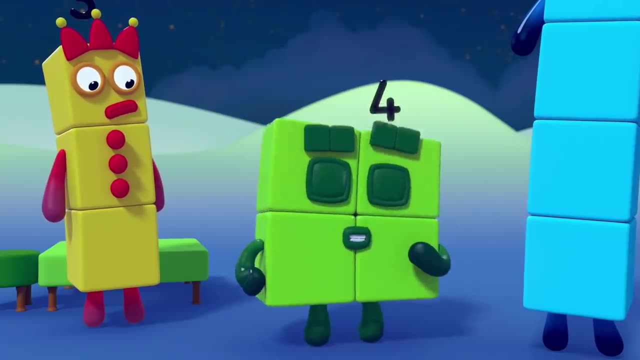 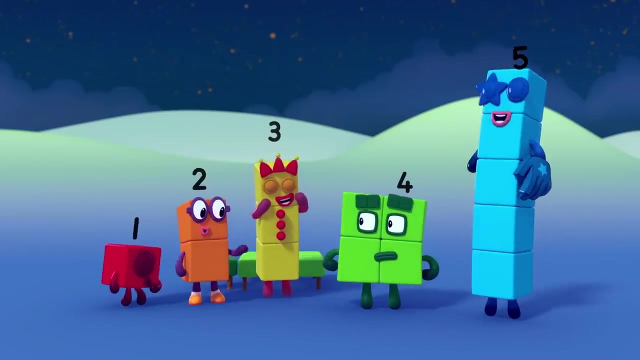 No, they made me. Well, I made them. Then they made me. I'm the terrible twos. I'm four lots of one, but I'm also two lots of two. You're funny, Don't be silly. That's very funny, Gemma. 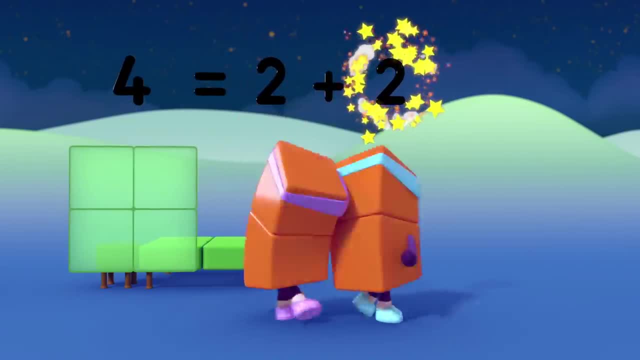 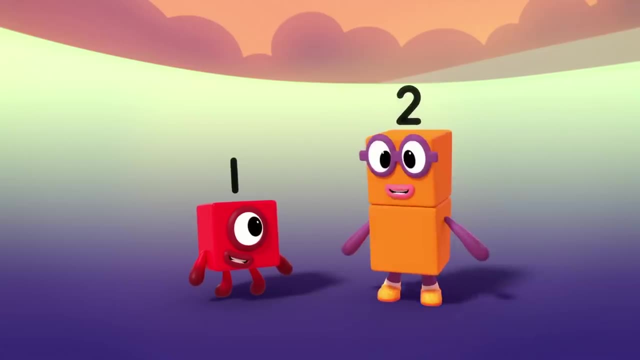 Four equals two plus twos. The terrible twos, Shh One, two And again One two. Your turn One. I can't do it. What was that That way? Come on, Wait, Looks familiar. 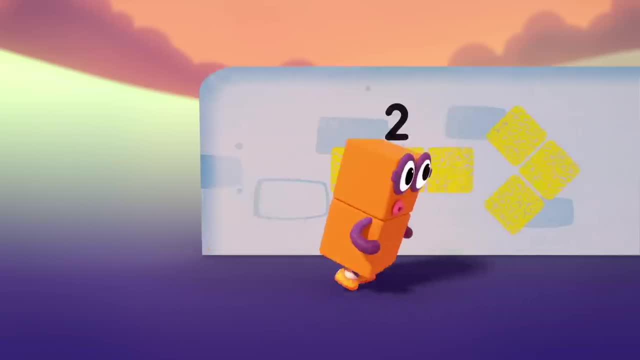 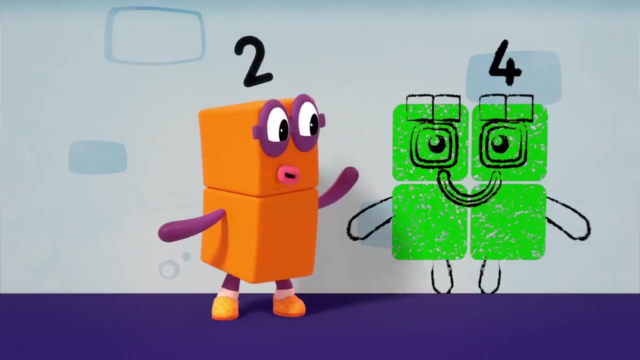 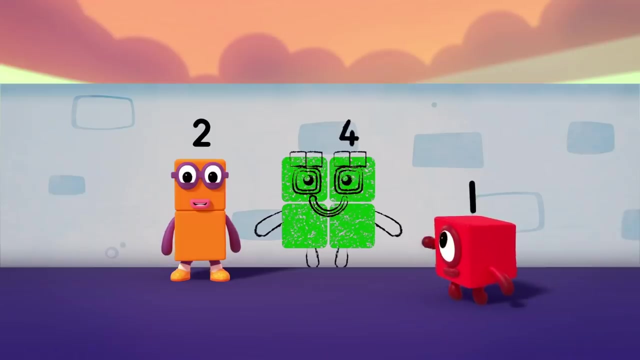 It's pointing to the sounds: Quick, Weeeeeee. Hey, it's four, Four, Four. Are we playing musical statues? Heh, A painting, A painting of four. I knew that, But what's that, Weeeeeee? 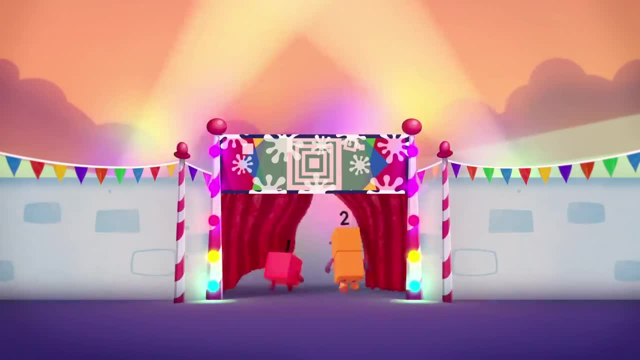 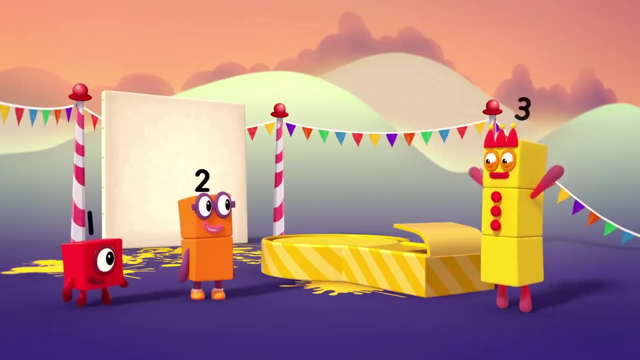 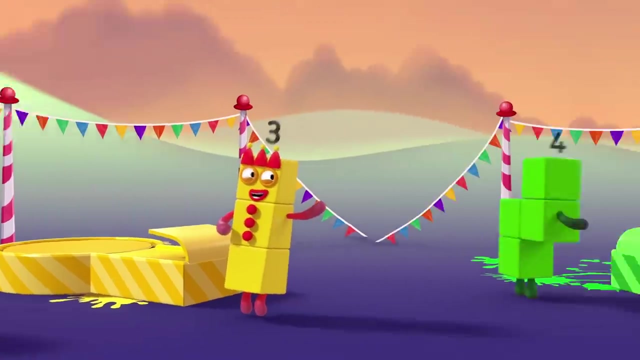 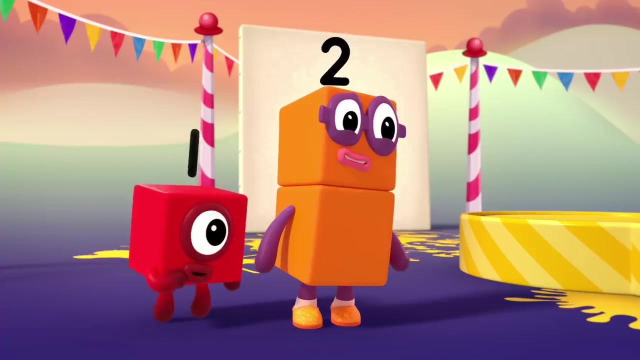 Weeeeeee Welcome, Welcome, Welcome to my new stampoline park. Don't you mean trampoline? No, no, no, Look Whee, Ooh, that was fun. Four Is that you? Of course it is One, two, three, four. 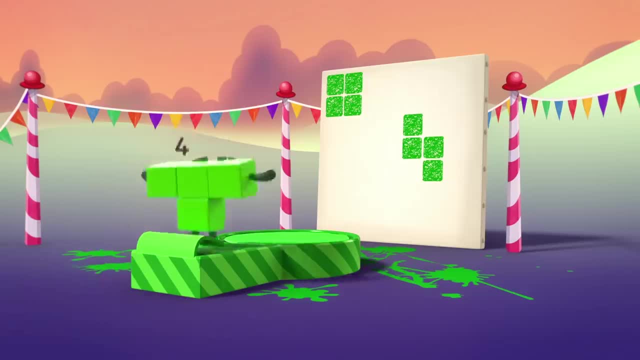 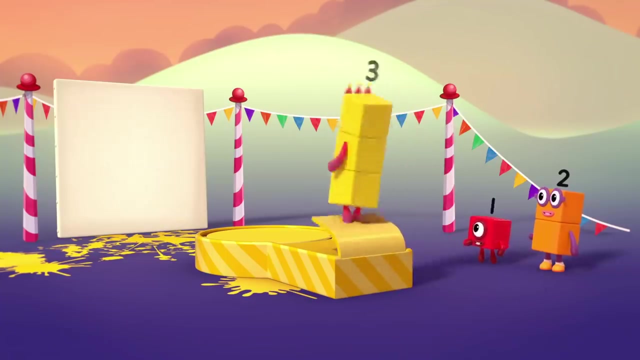 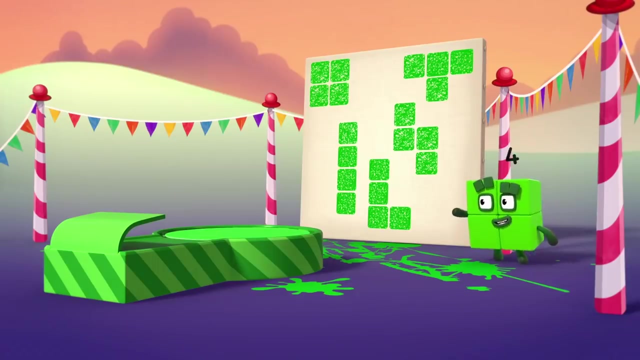 Four blocks. See Whee, Whatever way round I go, I'm still four. Whee, Look at me. Whee, I'm still three. Whee, Bum, bum, bum. Ooh, not bad, You think that's amazing? You should see. five: 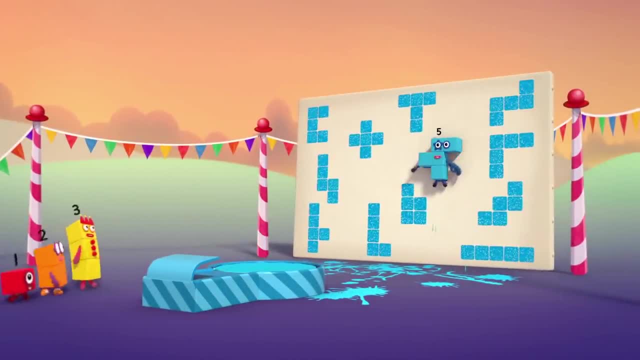 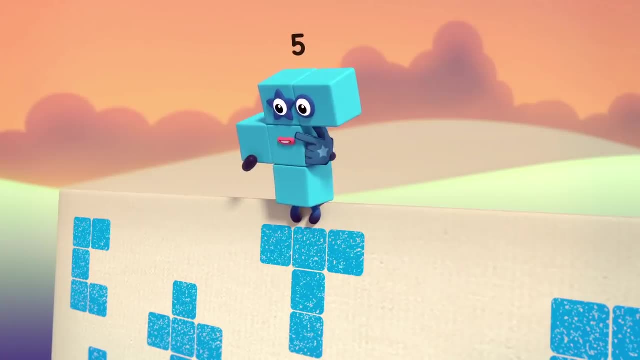 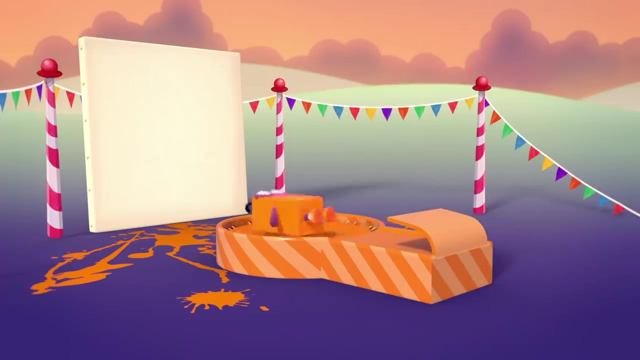 Five: Did you make all these shapes? I did so. The more blocks you have, the more shapes you can make. Oh, My turn. Not bad two, Of course. they're not really different shapes, are they? It's the same shape, one going up and one going down. 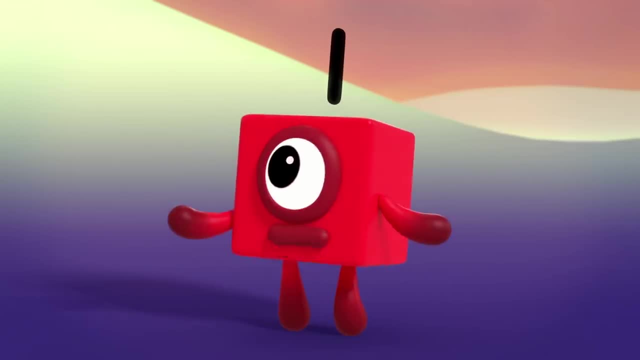 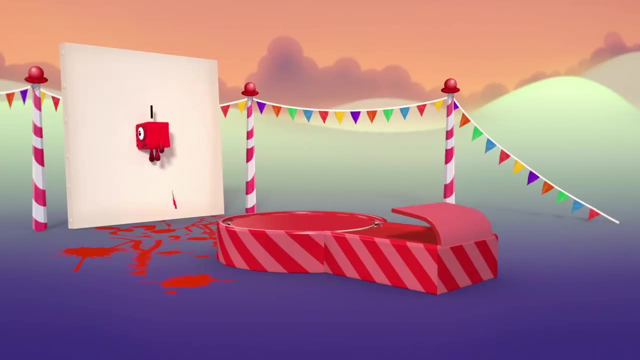 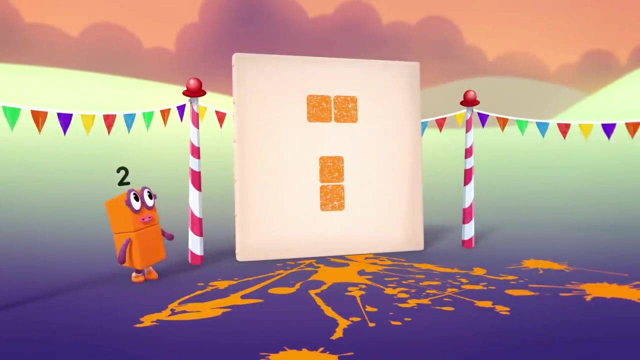 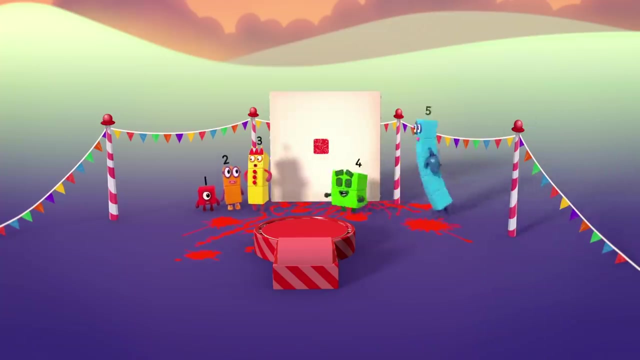 And one going across. Oh, it's still better than me. Look, That's all. One shape, Not very exciting compared to all of you Now. now, now You're forgetting something. One, two, three, Four. 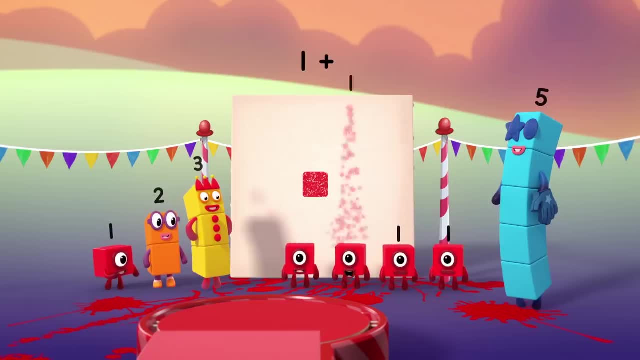 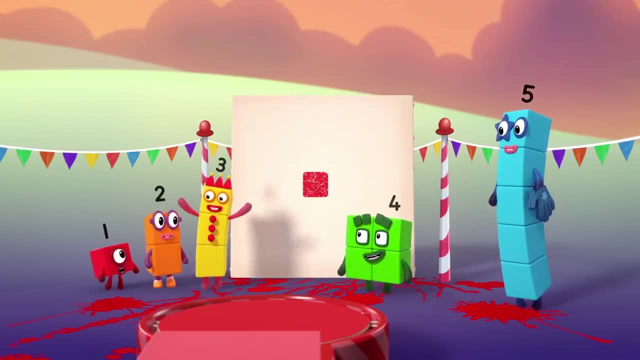 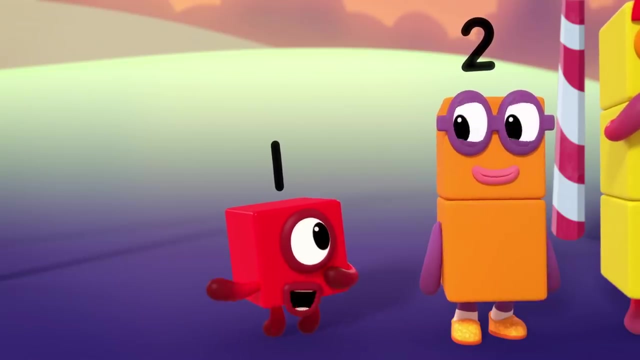 Whoa, whoa, whoa. Hey, One plus one plus one plus one equals four. Every big shape is made up of lots of little ones, So lots of little ones can make every big shape. Look what I can do, Whee. 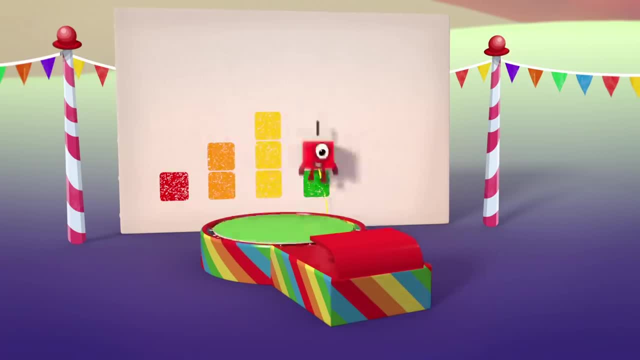 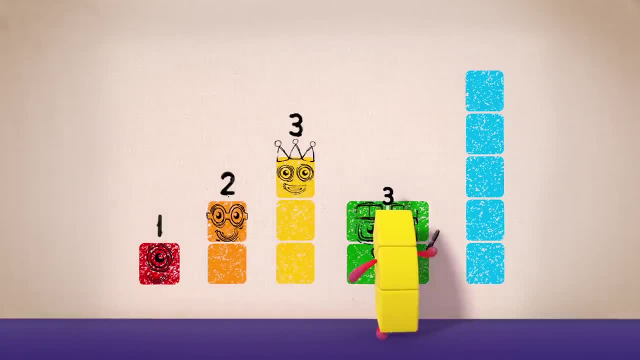 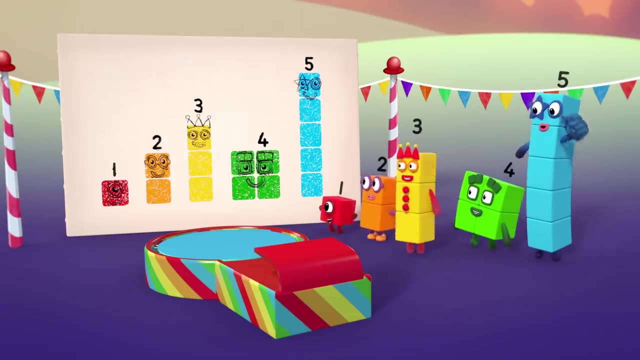 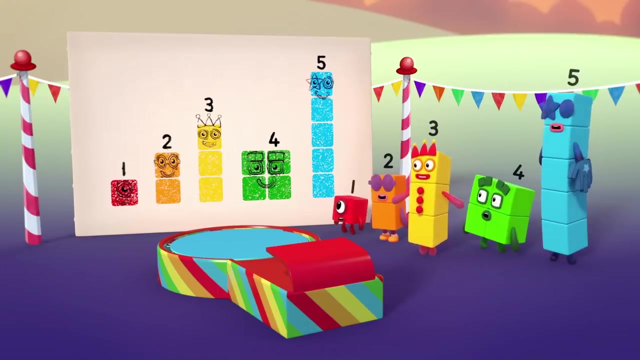 Whee, Whee. Oh, You made all of us. Well done, And just in time for the grand finale. What better way to celebrate opening my new park than with fireworks? Oh, May I present the Sky Act, Nut Yeah. 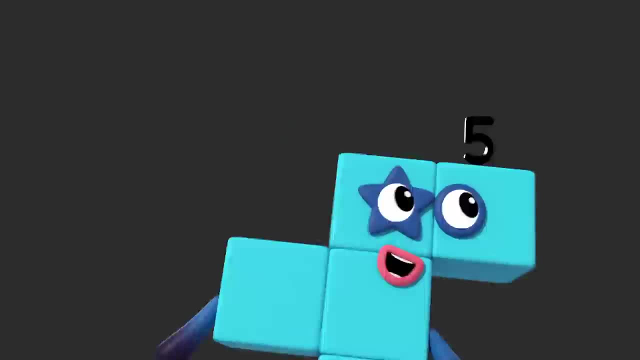 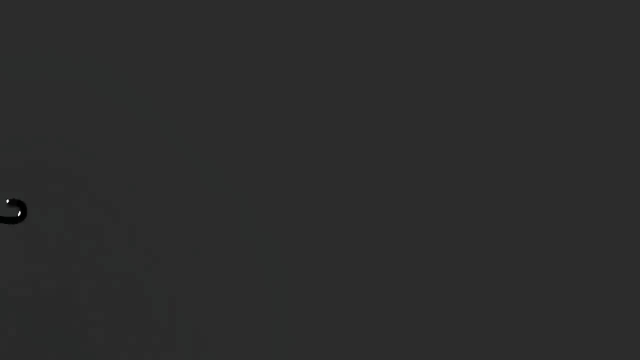 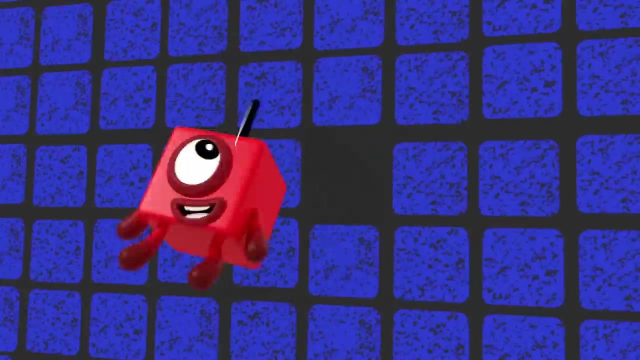 Whee, Yay, Yay, Yay, Yay, Yay, Yay, Whoo-hoo, Whoo-hoo Yeah, Whoo-hoo, Whoo-hoo Yeah, Whoo-hoo Yeah. 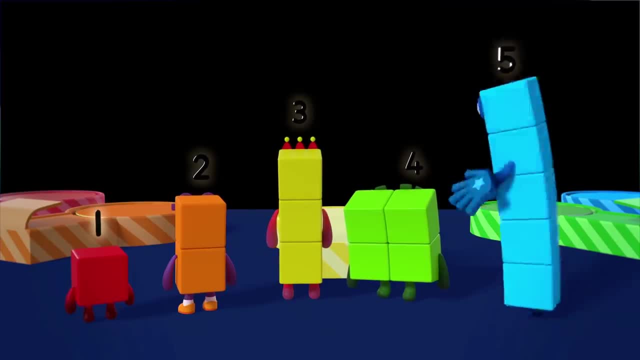 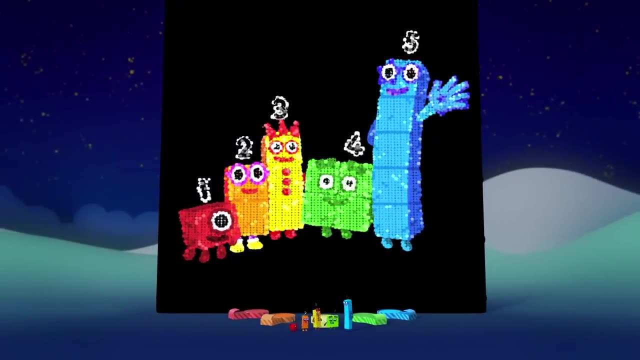 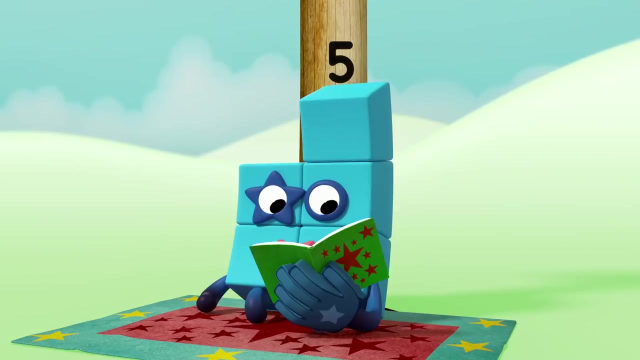 Whoo-hoo, You see one. When we all work together, the sky's the limit. Whoo-hoo, Whoo-hoo, Whoo-hoo, Whoo-hoo, Whoo-hoo. Hey, Found you. 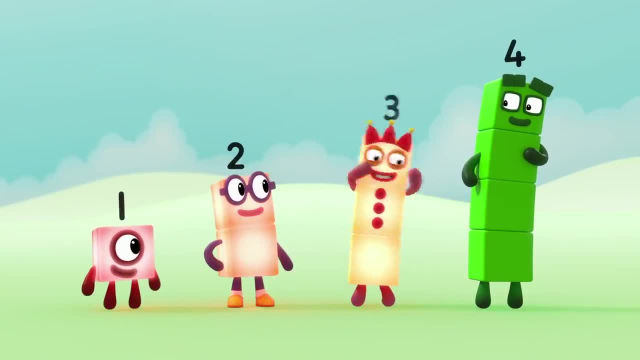 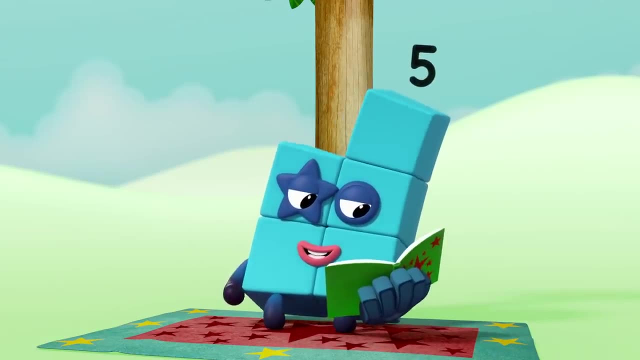 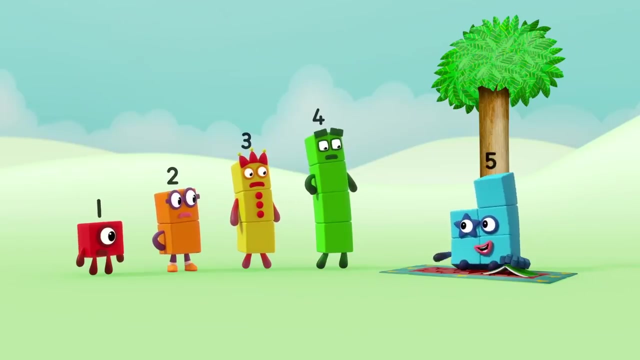 There she is. Hello, We're playing hide and seek. Want to join in? I would absolutely love to You hide, and I'll seek. Huh, You won't find us sat there. Oh, will I not now? I'm good at this game. 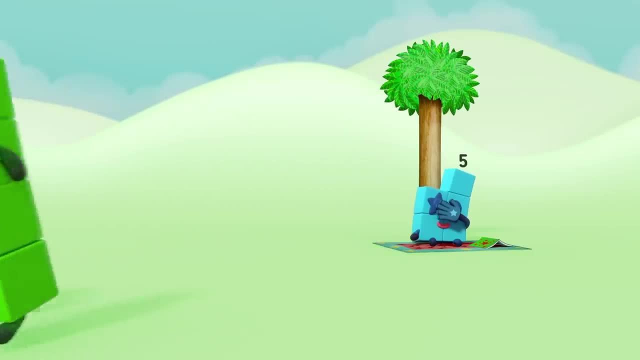 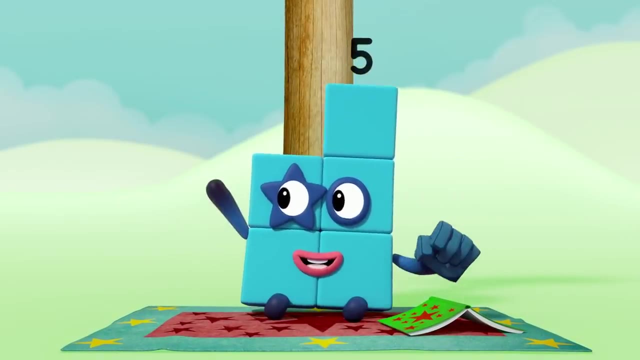 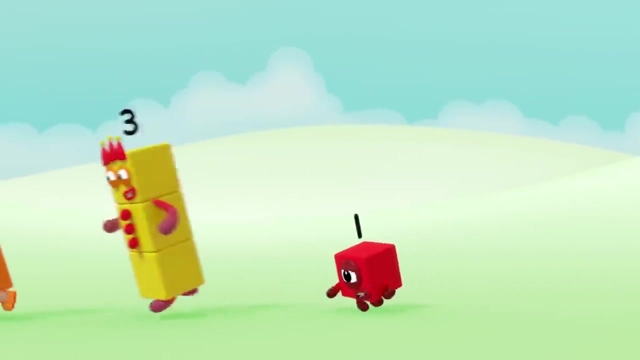 I'll get you out Whoo-hoo One, two, three, four, five, Ready or not, here I Get on with my book: Whoo-hoo, Whoo-hoo, Whoo-hoo, Whoo-hoo. 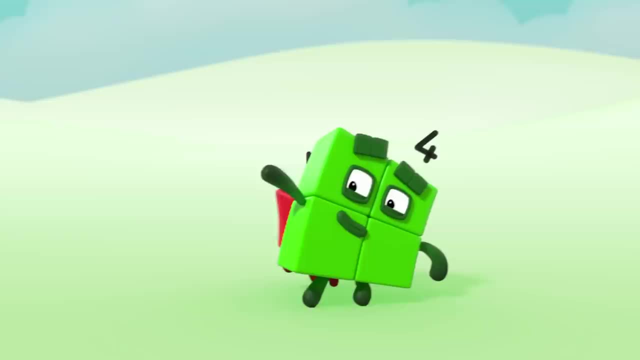 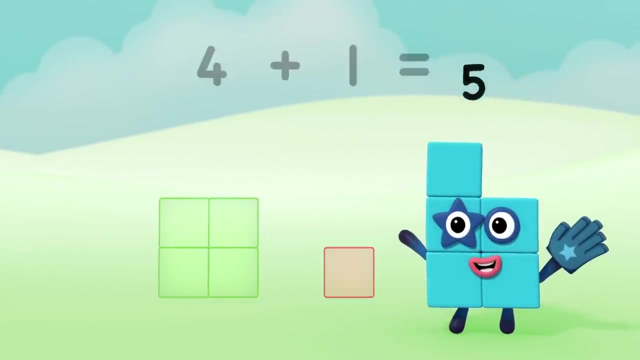 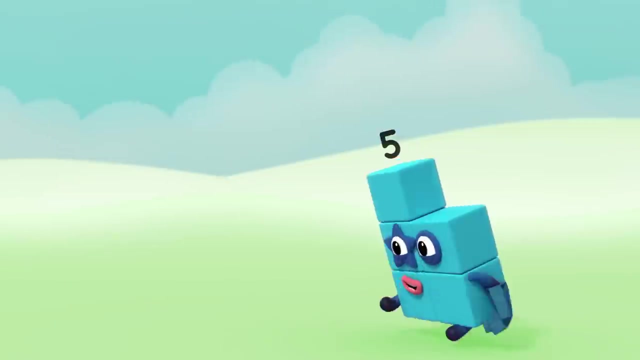 Whoo-hoo, Hey, Hide behind me. Where can I hide? No, behind you Four, Oops. Four Plus one equals Five. Ready or not, here I come. Find you four, find you one. Five minus one. 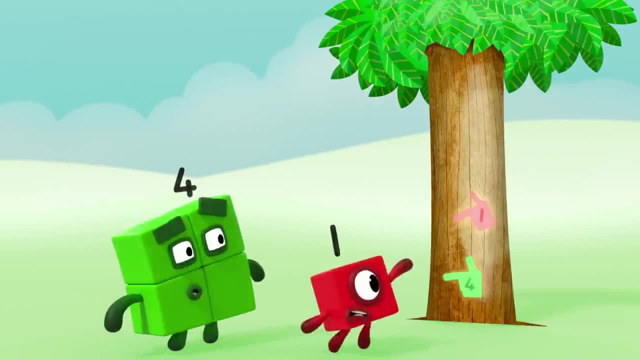 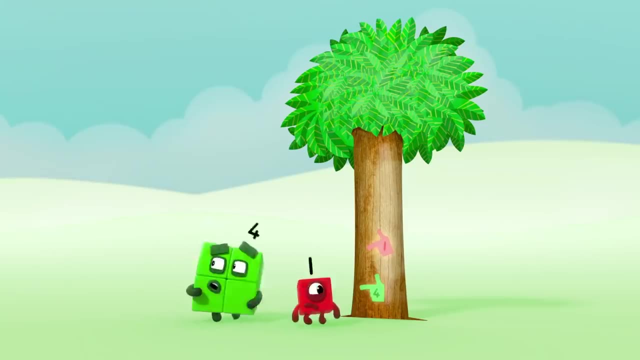 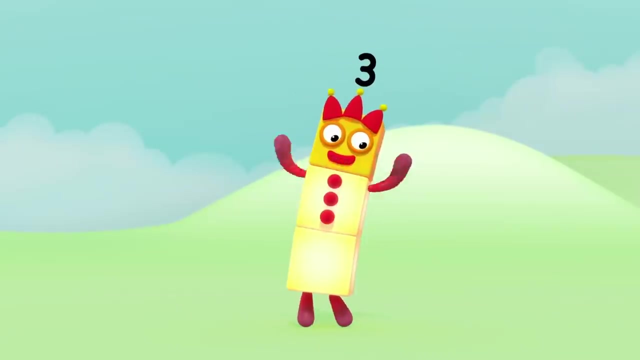 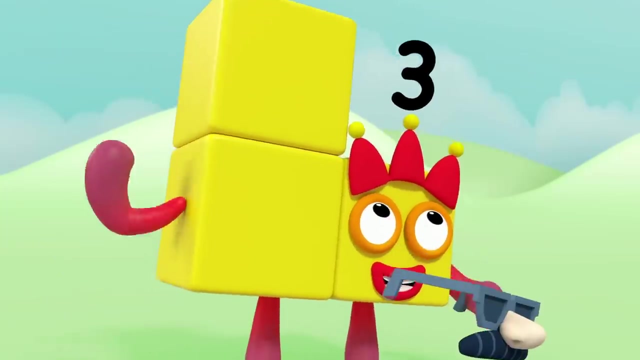 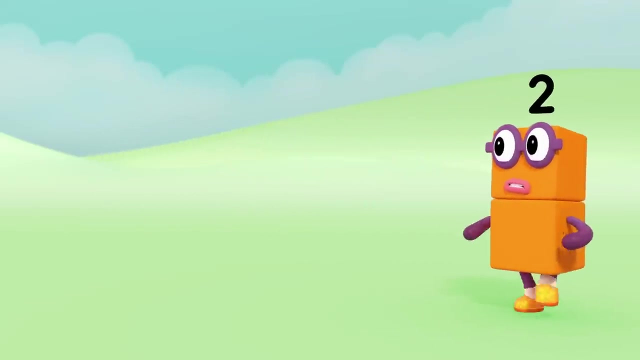 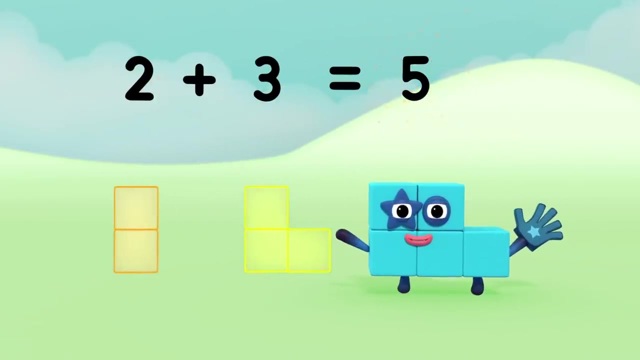 Equals four. Look Five, said she'd point us out. Five was right here. How? Two And Three, Two, Three, Two And Two, Two, Two, Two, Three, Two, Three, Two. Ready or not, here I be. 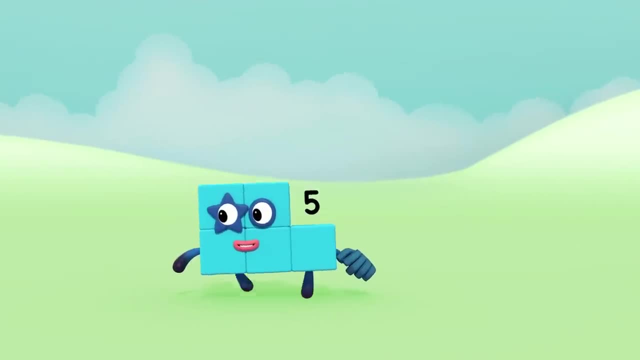 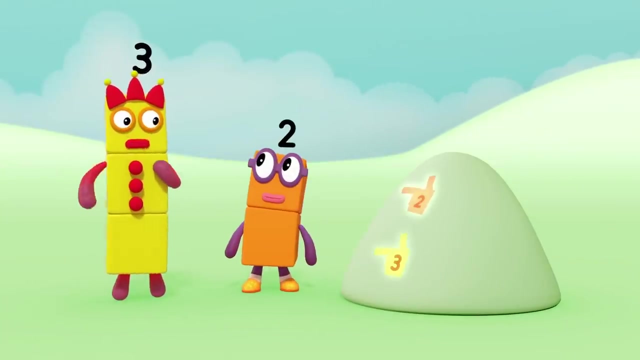 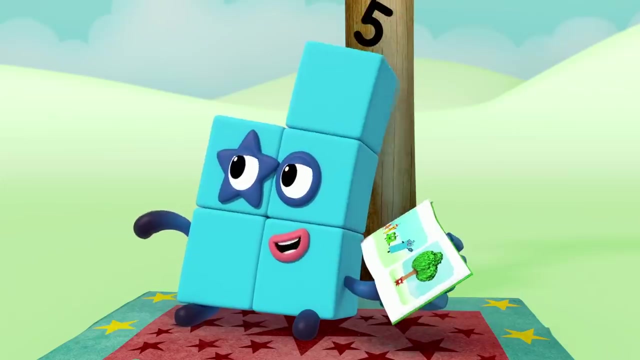 Find you two, find you three. Five minus three Equals two. A pair of pointing prints. Five found us, But but how, Uh Five You're here. How did you Told you I was good? Now my turn to hide. 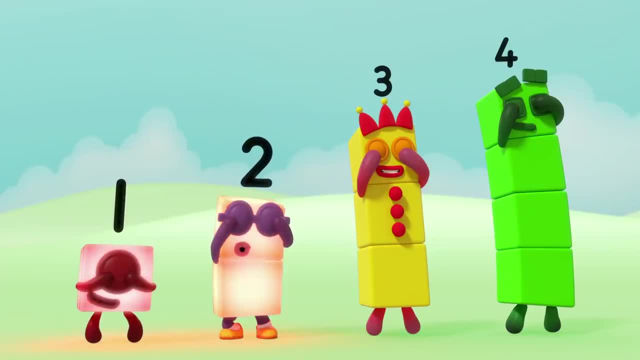 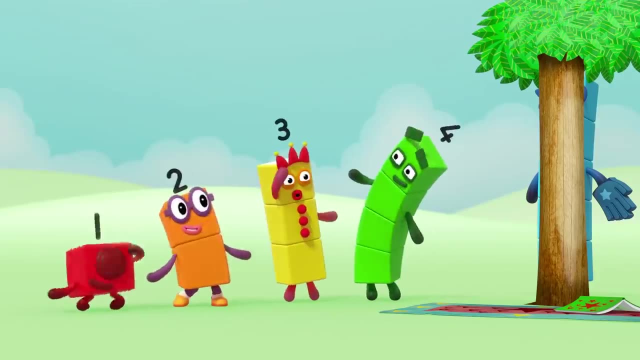 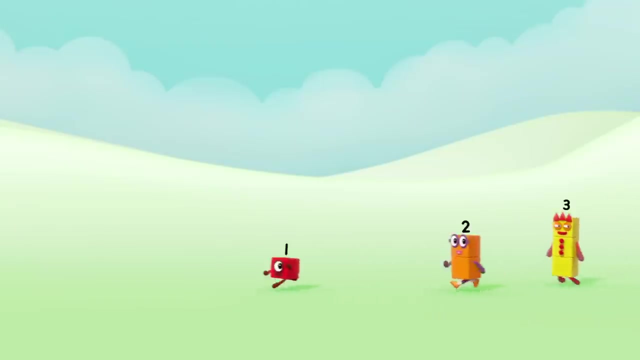 We're done. One, two, three, four. Ready or not, five here we come Rock. One plus four equals Five. Found you Amazing? Can you find me again? Five minus four Equals one, Come on. 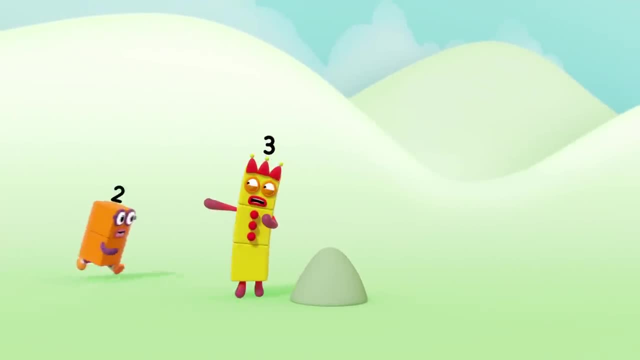 Rock. Uh-oh, Ah, Uh-oh, Uh-oh, Come on. Three Plus two Equals Five Found you. Fantastic, Can you find me again? Five Minus two Equals three Found you. 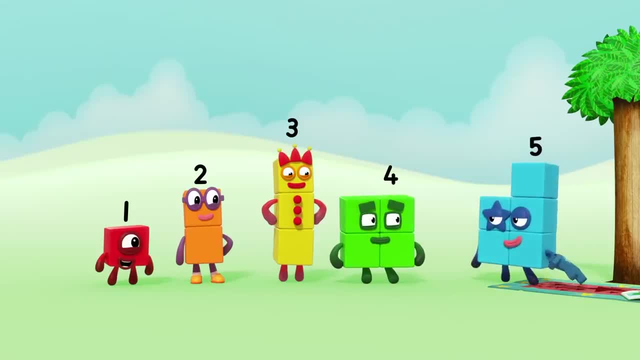 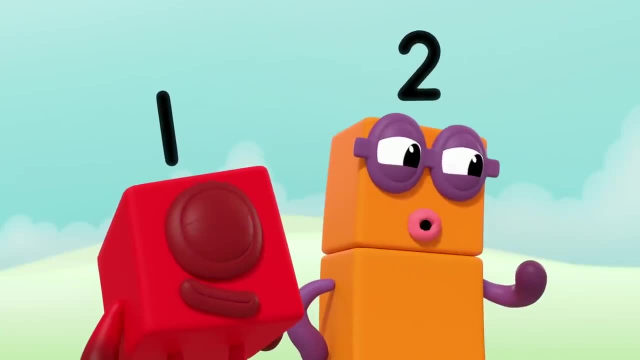 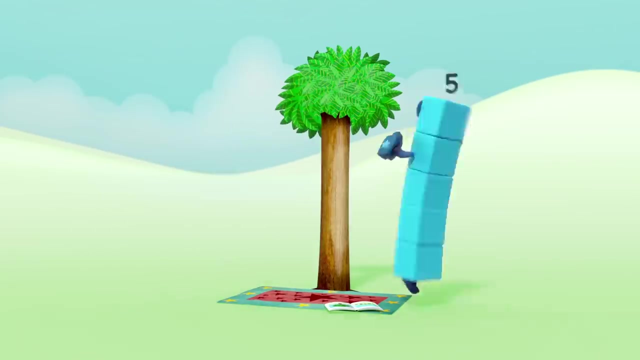 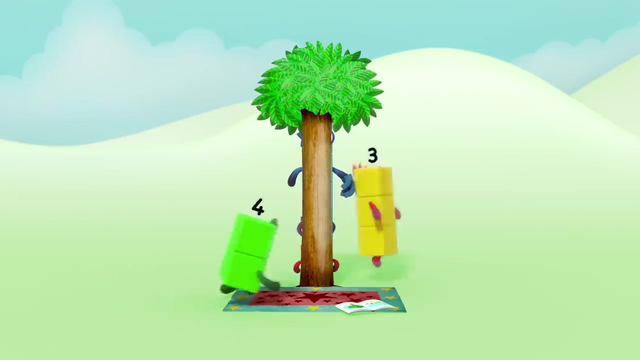 You stars, Uh-oh, Uh-oh. Can you teach us to be as good at hide-and-seek as you? Sure I can Try this. Oh, Four, Oops. What a great game of hide-and-sheep. but now it's time for Sheep to sleep. 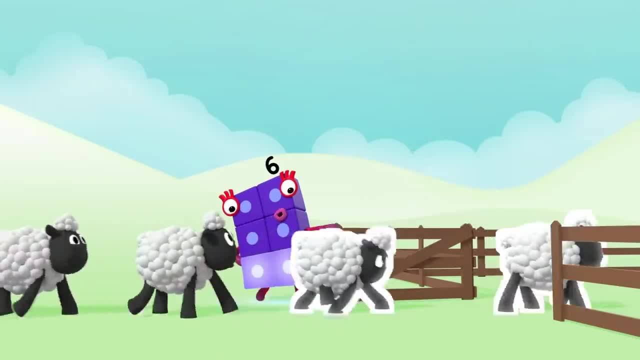 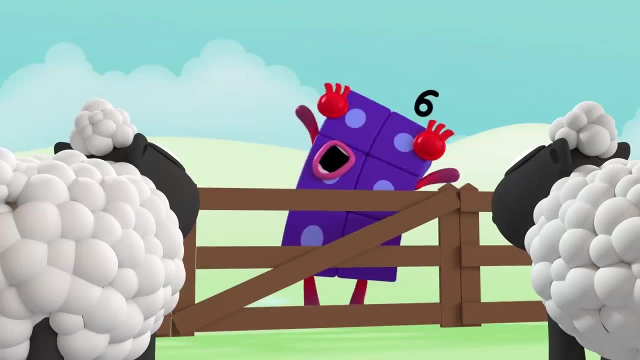 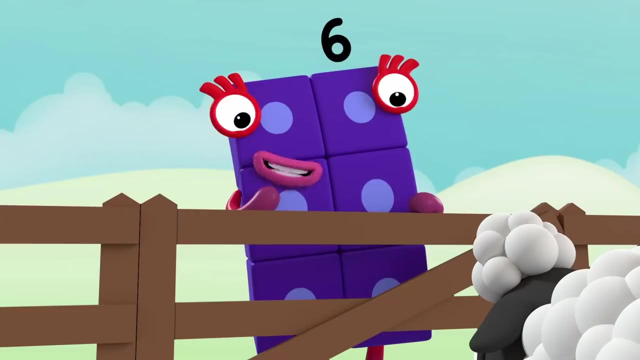 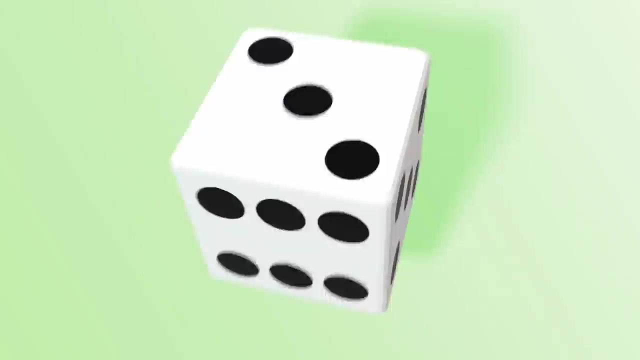 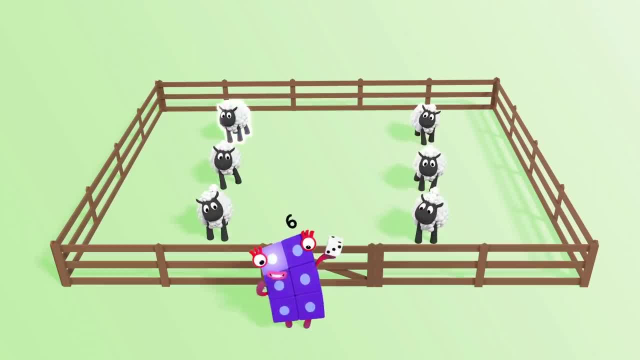 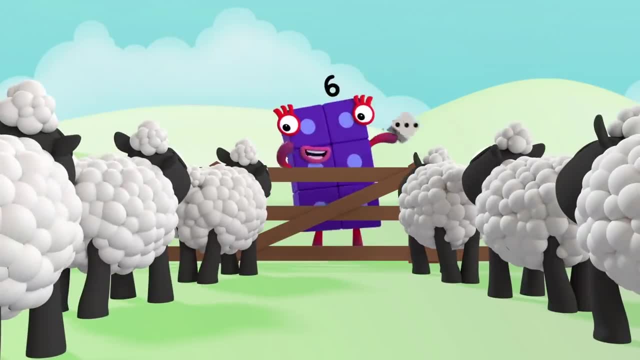 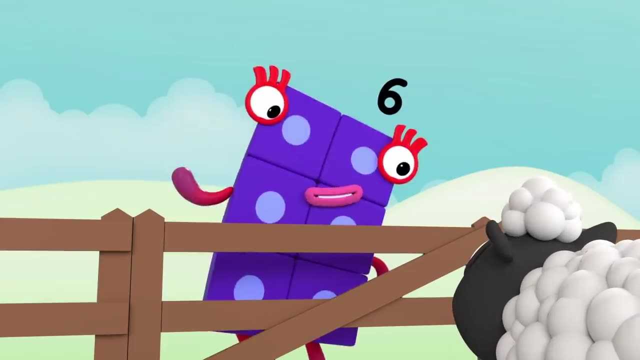 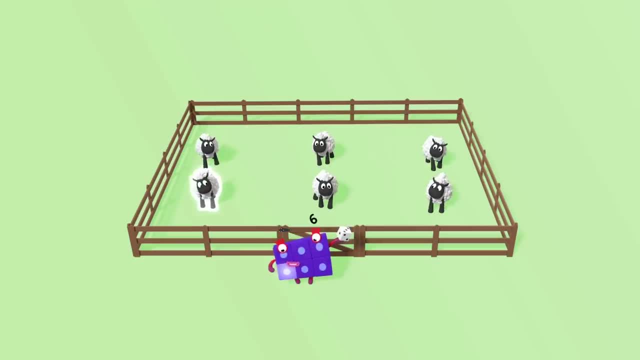 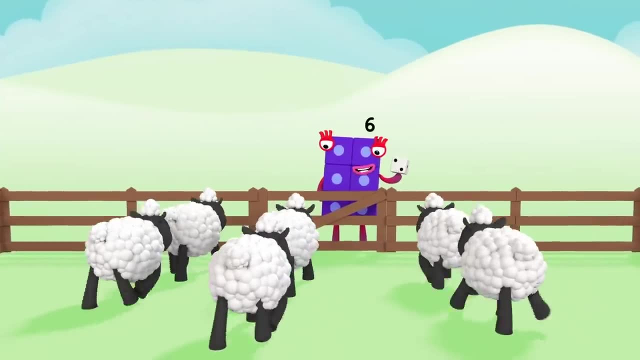 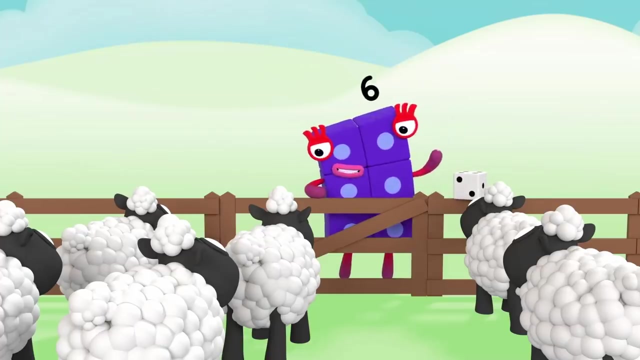 Arrange yourselves in groups of two, One, Two, One, Two, Oh, Six is the same as three. lots of two. I know that now, thanks to you. Listen, now I can't count more sheep. It's time for you to get some sleep. 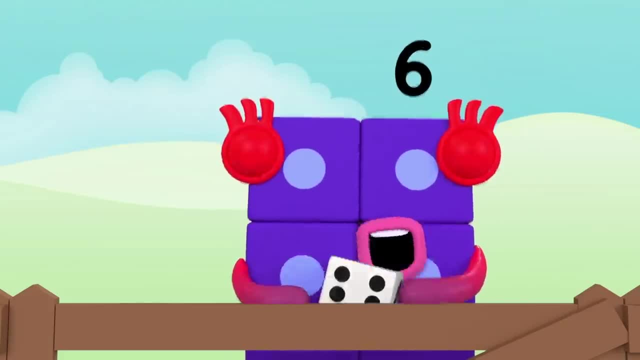 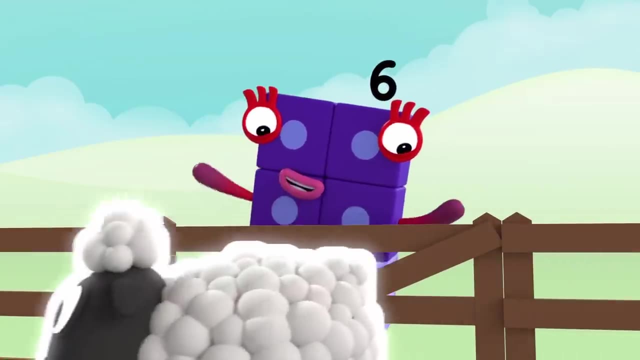 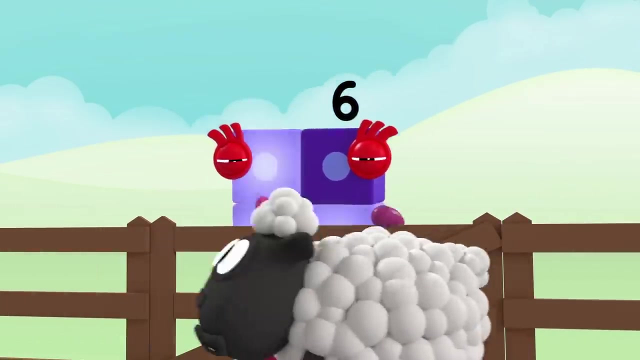 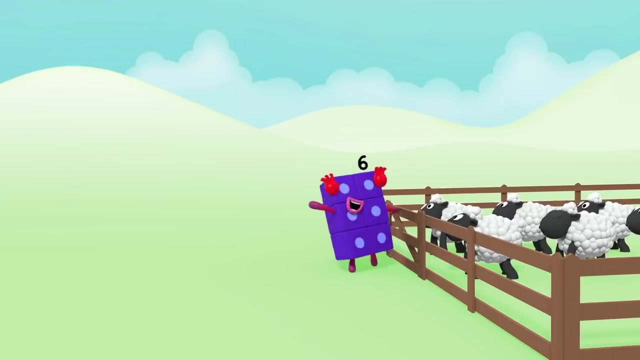 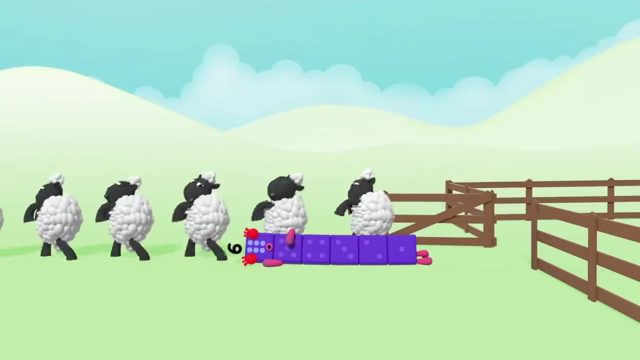 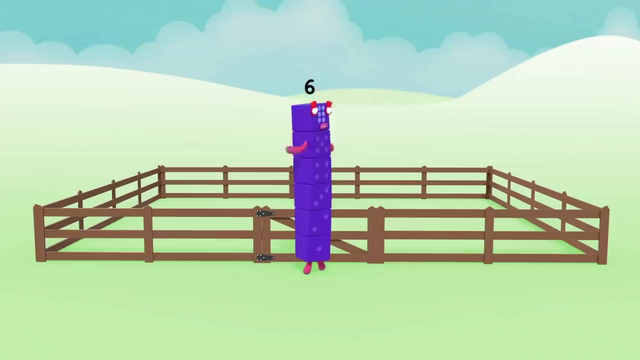 Oh, I see Time for tricks. Arrange yourselves in a group of six: One little sheep, Two little sheep And three little sheep, Four little sheep, Five little sheep And six little sheep. Wait a moment, Was that the gate? 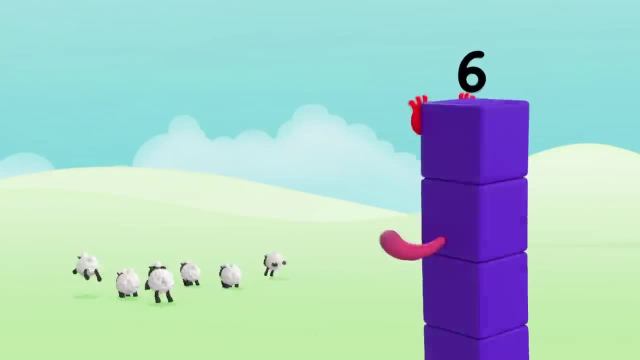 It was. They're gone. I'm too late, I'm off. Oh no, I'm off. Look at that. Two lots of three. That's one too many for just one- me, Is it? Look at that. Two lots of three. 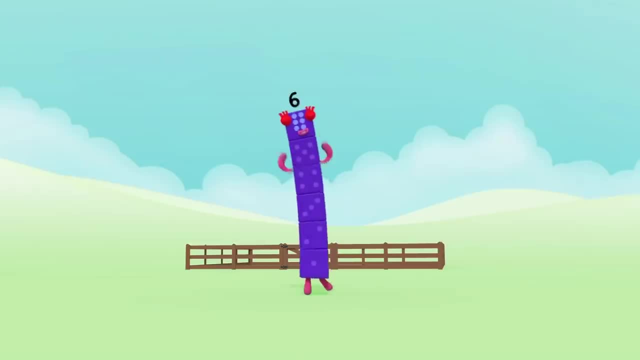 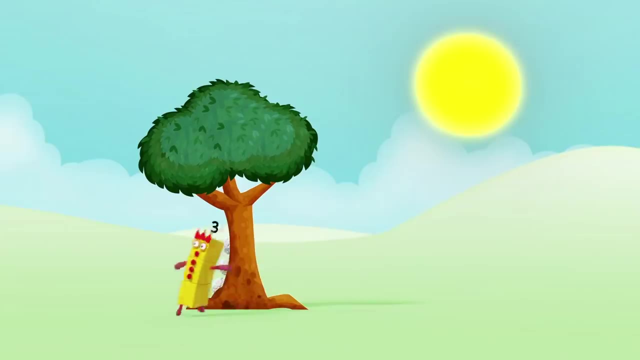 That's one too many for just one- me, Is it? Look Ah Baa Baa, baa baa baa baa On the left. On the left Baa Ah, Found you Sheep One, Two and Three. 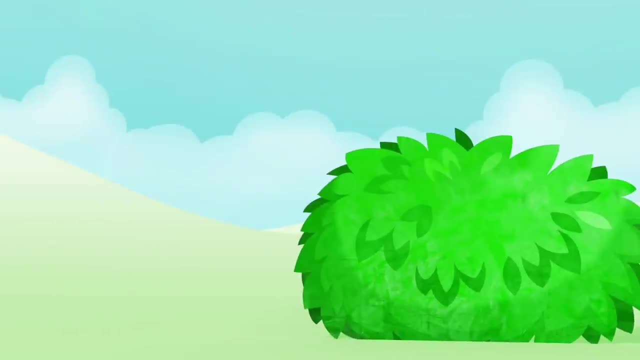 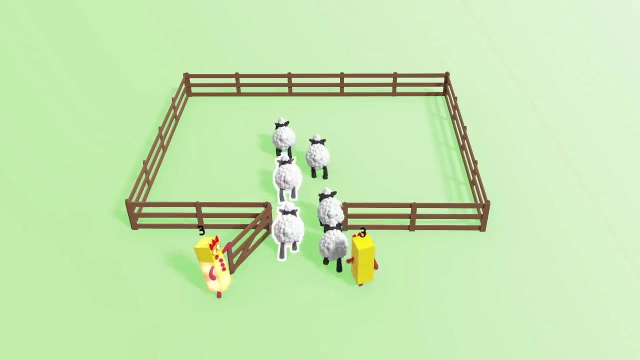 There you are Behind that tree, Baaa, Baaa, I found another one: One, two, three. You gotta be smart to hide from me. One, two, three, That's three from me. One, two, three And three from me. 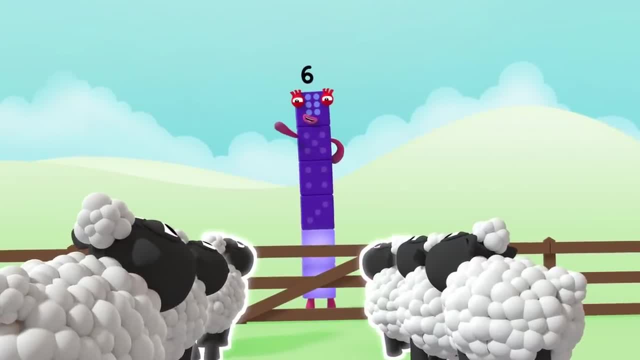 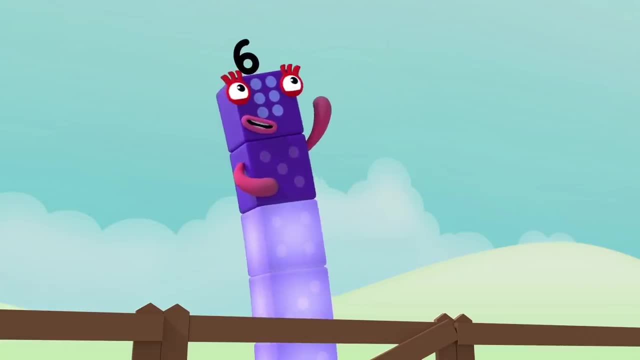 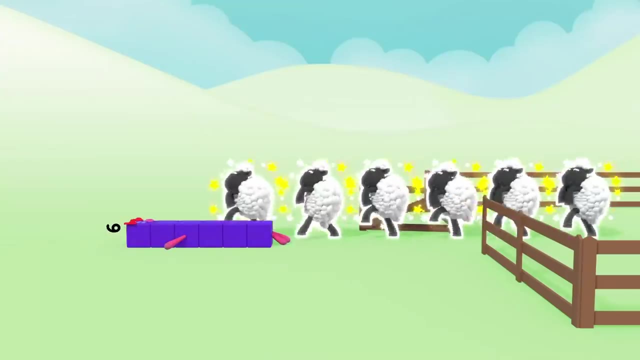 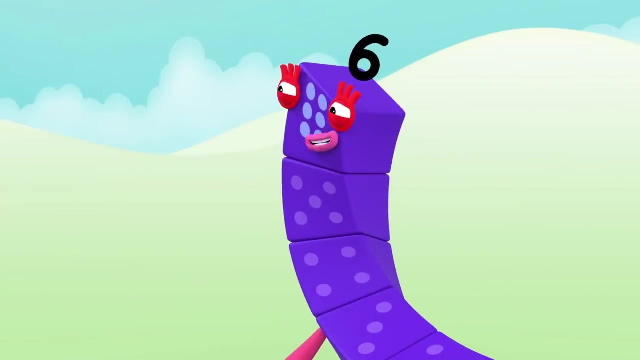 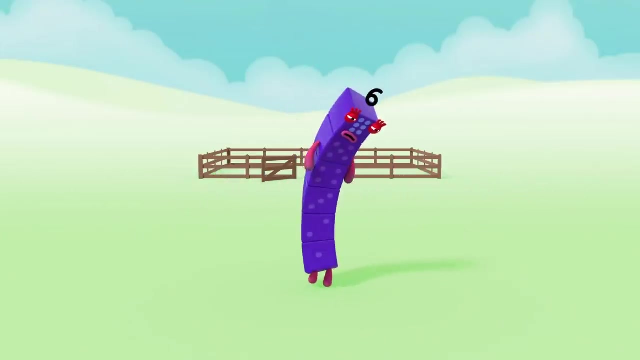 One little sheep, Two little sheep And three little sheep, Four little sheep, Five little sheep And six. Not again, You naughty sheep, Come back here. It's time to sleep. Oh no, They found three ways to run. 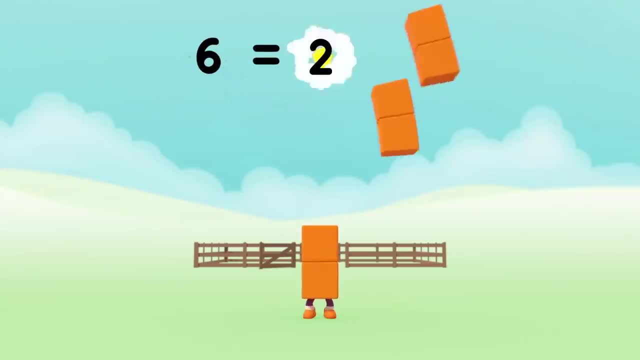 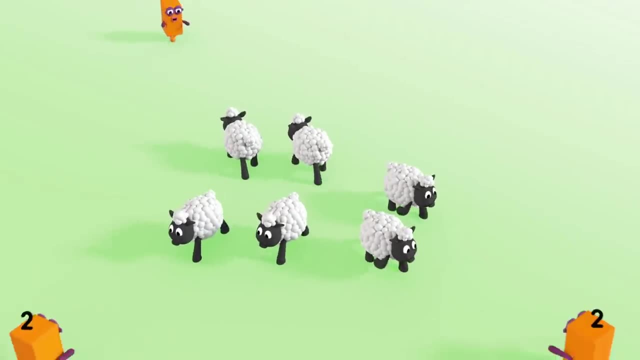 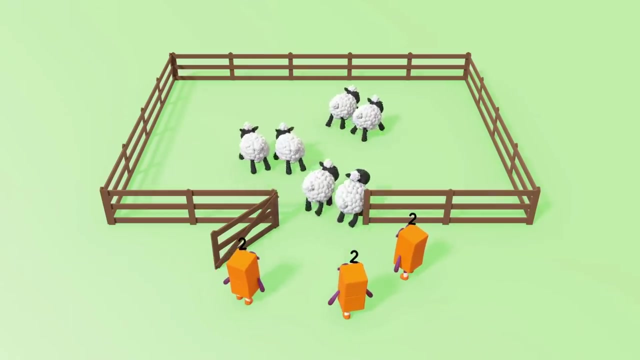 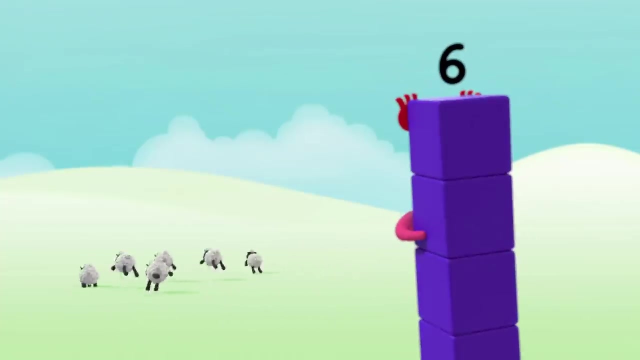 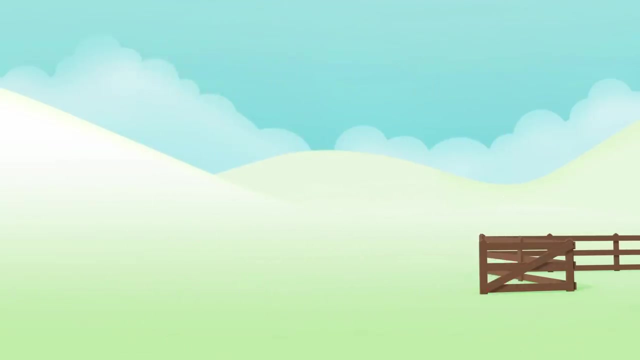 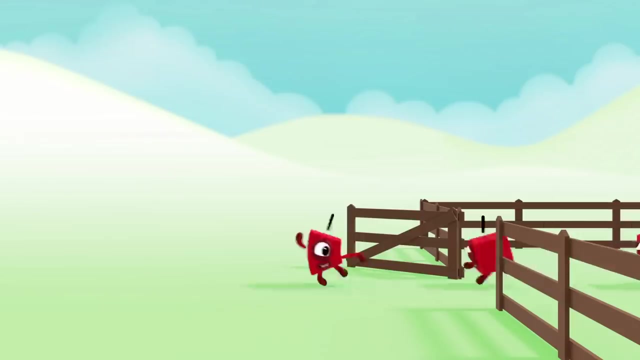 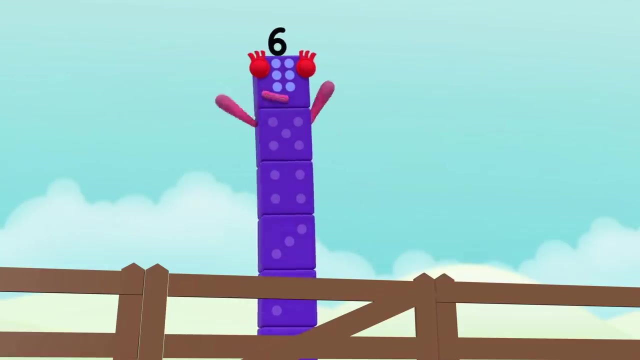 And I thought counting sheep was fun. Quick march: One, two, one, two, one, two. If that's the way you want it to be, six naughty sheep need six of me. Yeah, Now listen, You naughty sheep. it's definitely positively time to sleep. 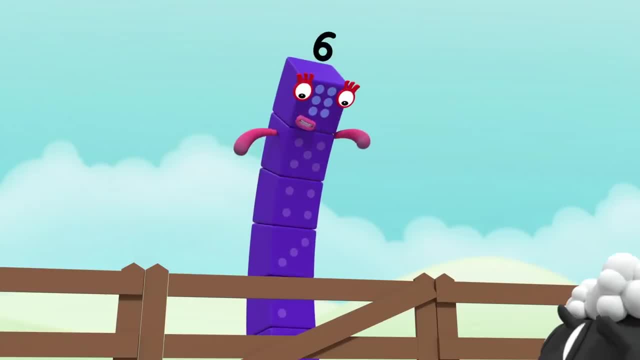 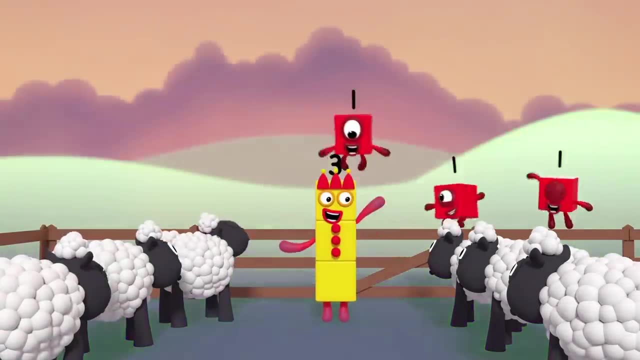 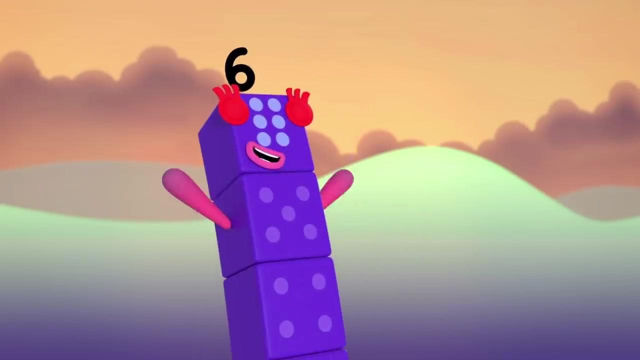 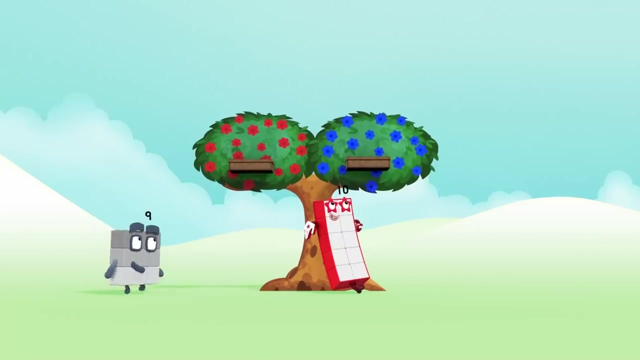 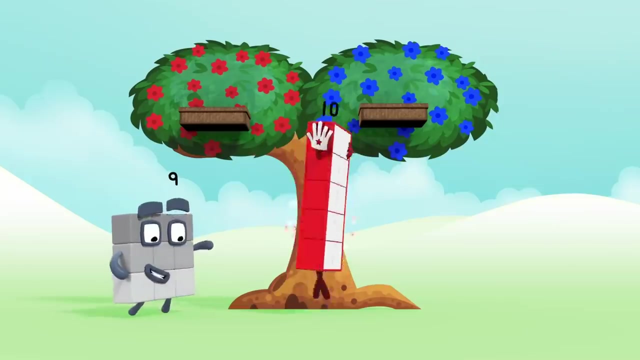 If counting sheep sends me to sleep, counting blocks might work for sheep. Finally, bedtime. At the same time, it's time to pick your own grabbed things. I'm going, I'll go with you. You're so cute, You're so cute. 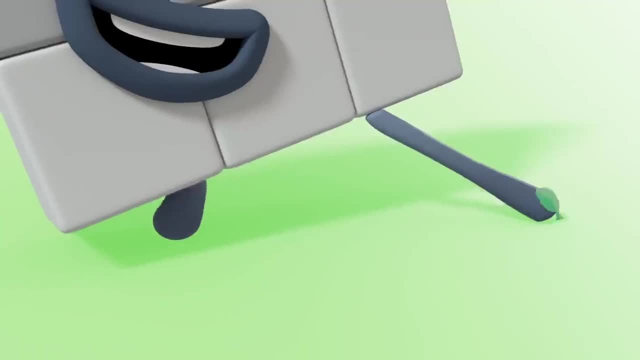 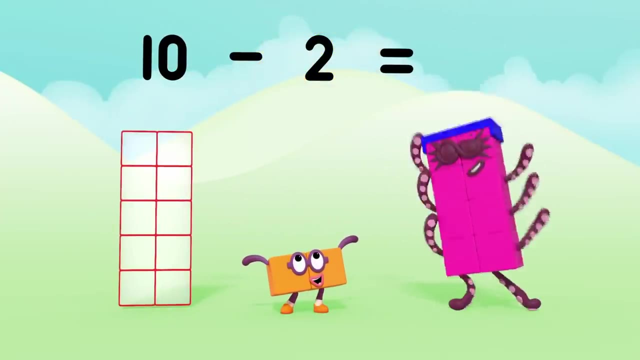 Done. What about this? You know I've got this. Go on and try it. Why won't you try it? Come on, Go and hit me, Here we go, I'll try it. Oh, no way, I'll do it myself. 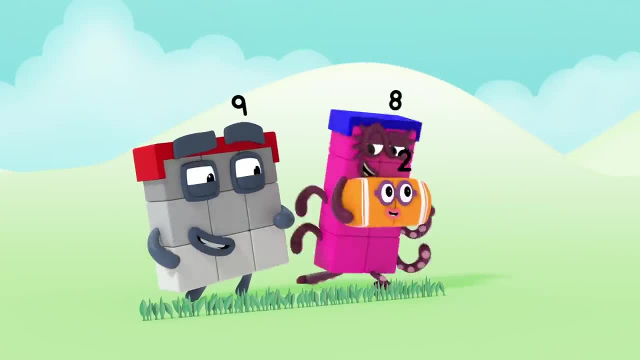 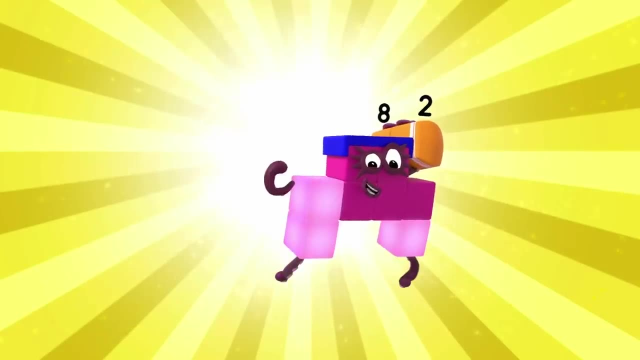 What's it gonna be like without me? You need to hit me, you fool. Oh, you mean this. Oh, no, That's enough, I'll do it. Play One, two, three, four, five, six, seven, eight play. 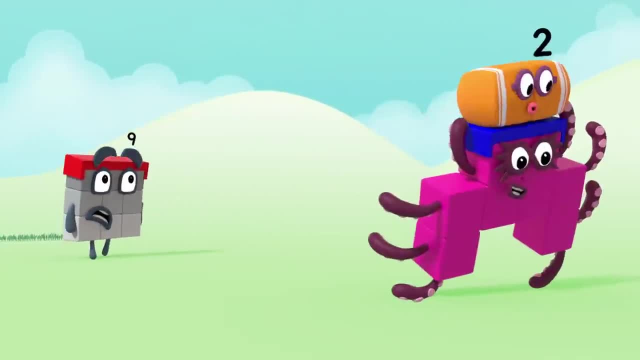 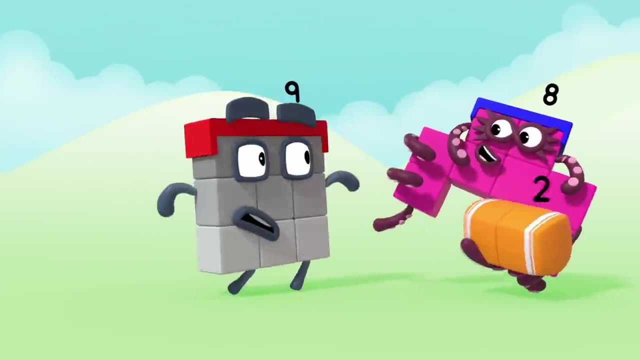 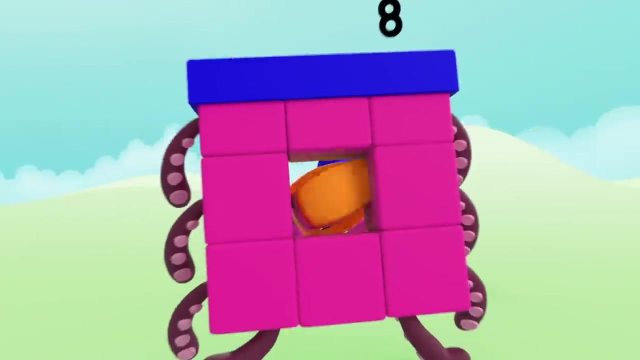 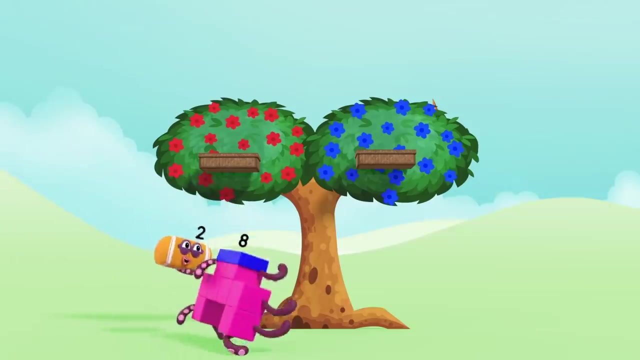 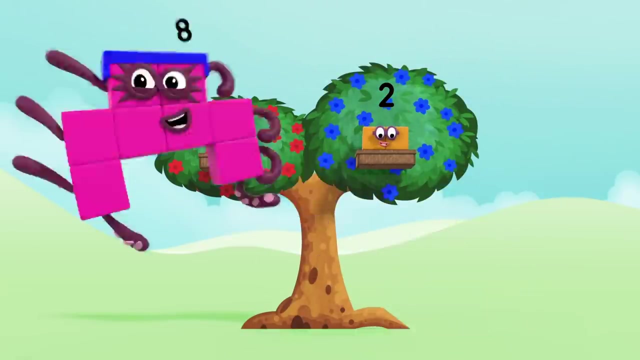 He's on the left And now the right. He's on my head Now, out of sight. Up high, Down low, Too slow Action, Octoblock jump: Score Two points to Blues. I'm bigger now, so it's my turn. 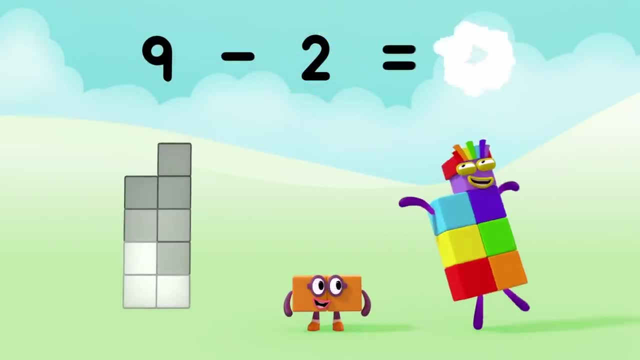 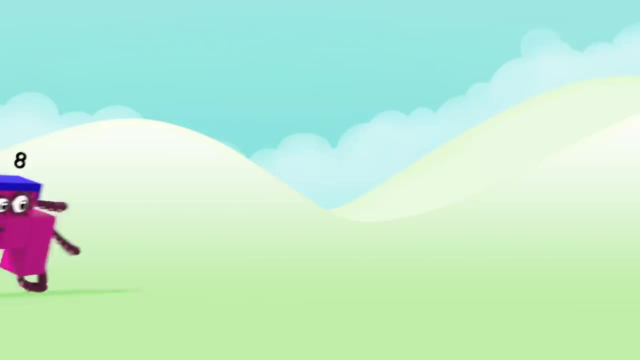 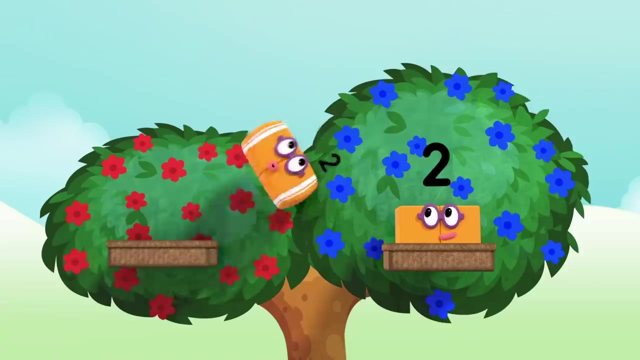 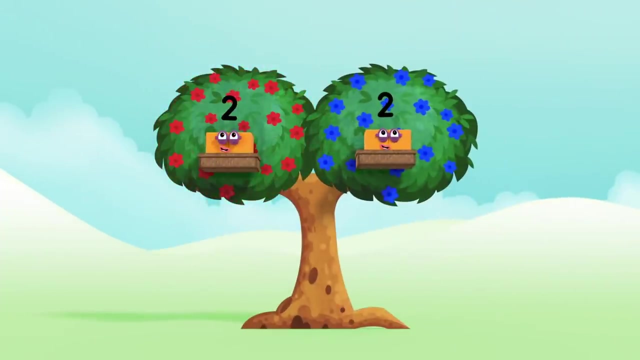 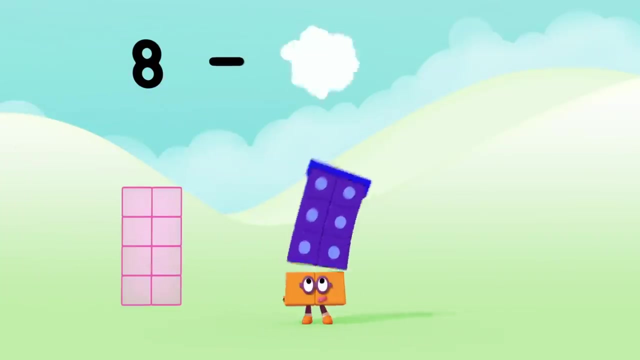 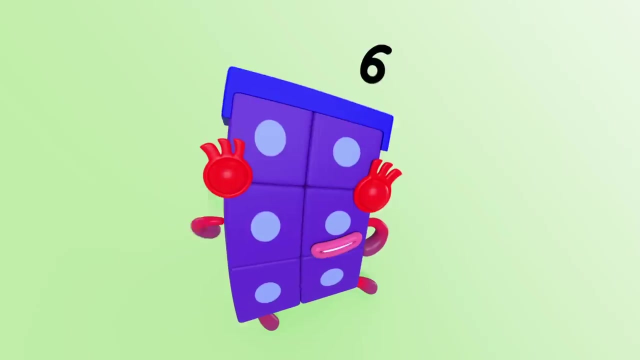 Nine minus two equals seven. Ready Go, Whee, Woohoo, Whee. Two points each. Beginners. luck, You're bigger You start. Eight minus two equals six. This game is nice, Let's roll the dice. 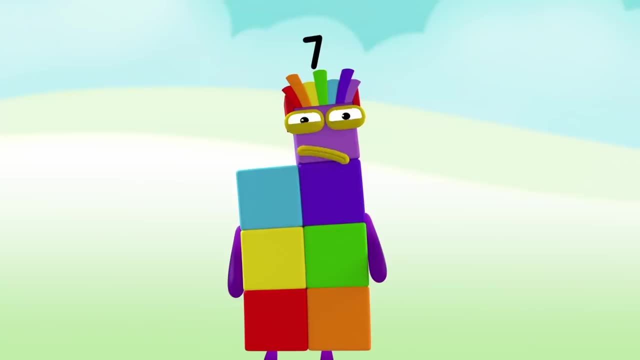 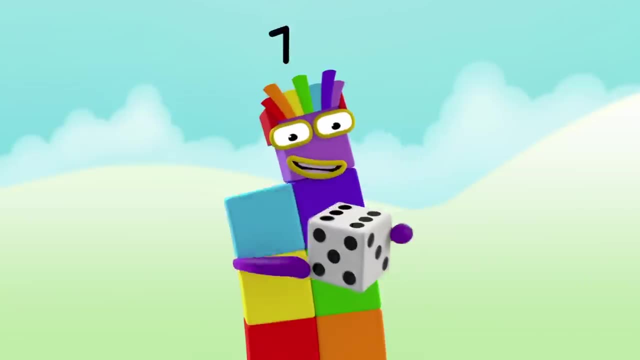 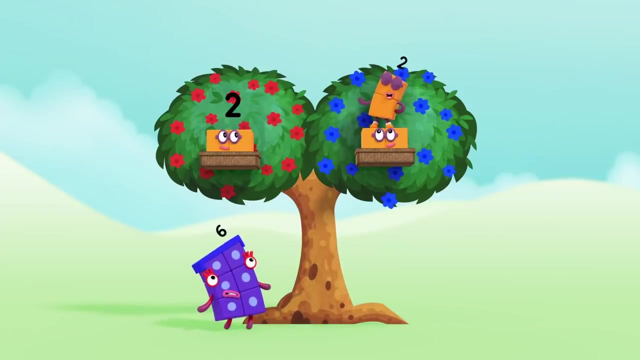 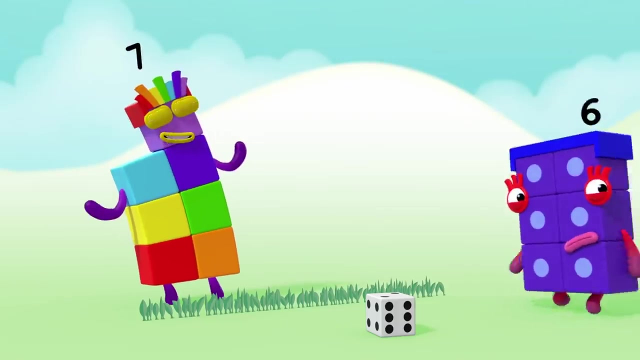 When it leaves my hand. how will it land? Um on six? Oh, lucky me, Lucky me. Penalty, Unfair distraction, Which means Four-two. Better luck next time, Here we go. Seven minus two equals five. 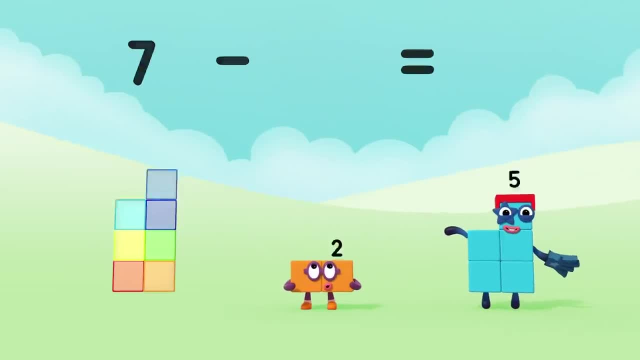 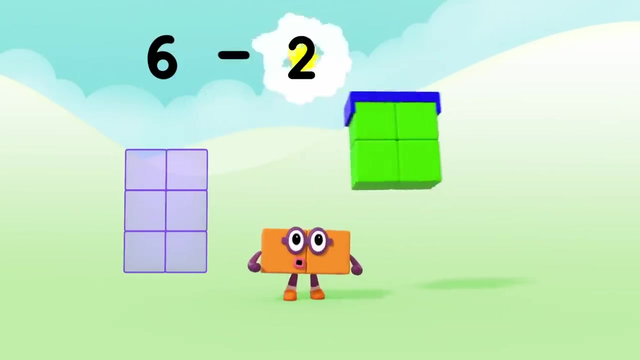 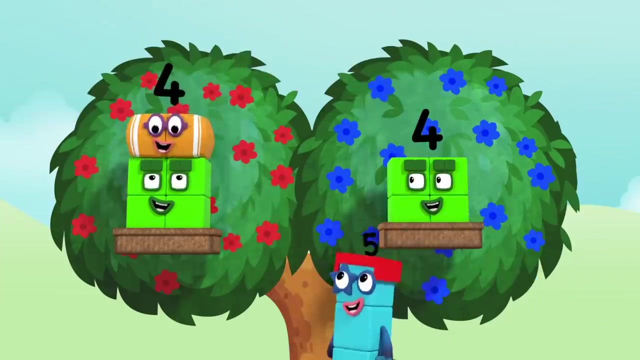 Seven minus two equals five. Hehe Oh, Four points each Six Minus two equals four. Four points each Six minus two equals four. овали, Uh Huh, Three, Six, Four. Five minus two equals three. 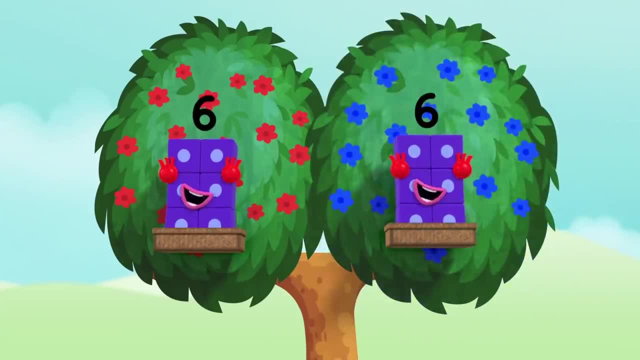 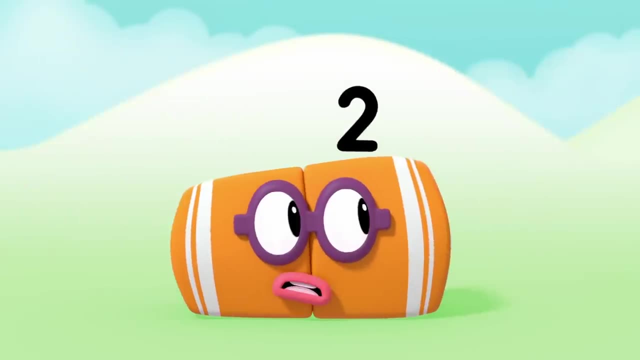 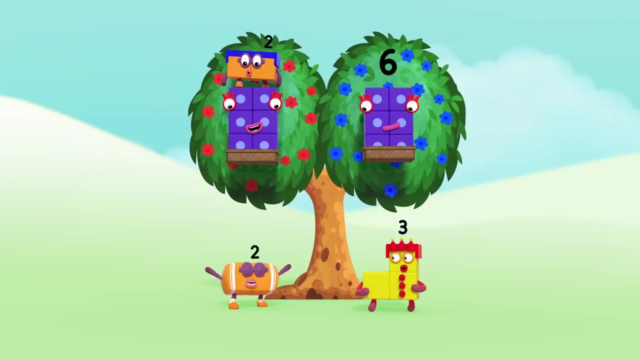 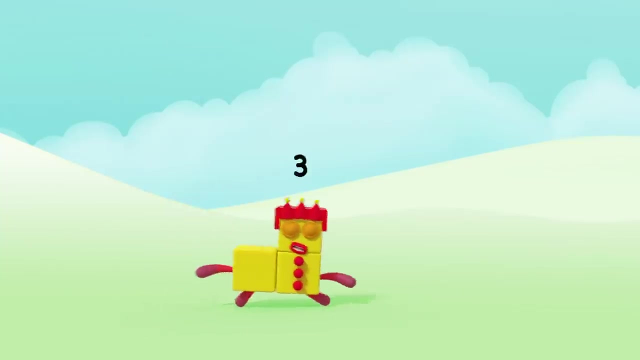 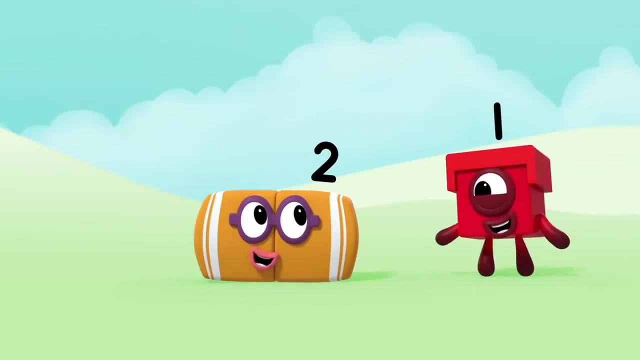 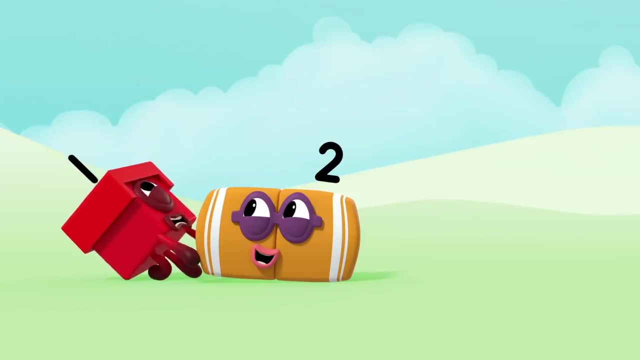 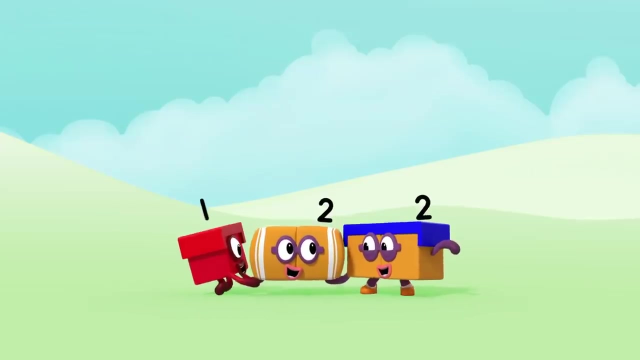 Six points each. Four minus two equals two. Hey, Not me. Penalty round two, Oh Eight. Three minus two equals one. Final round, Ready Go, Oh Bother. Let me lend a hand Or two. Thanks, Two Up there, please. 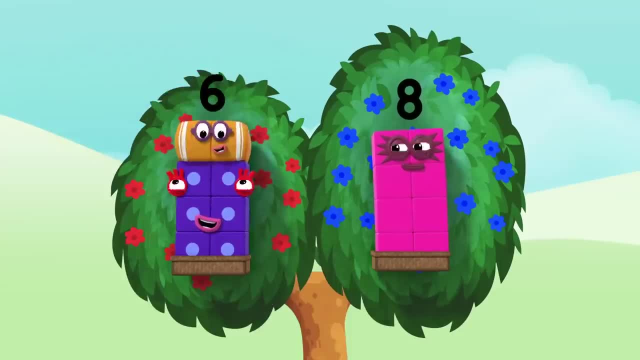 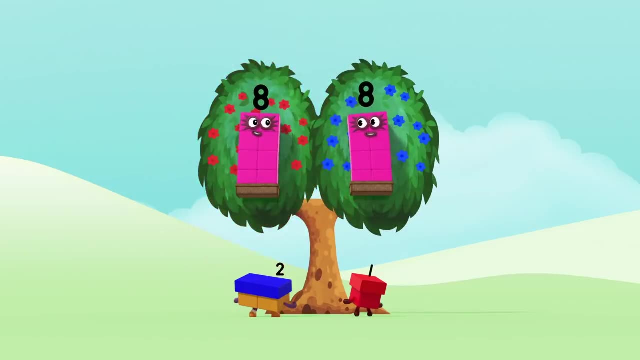 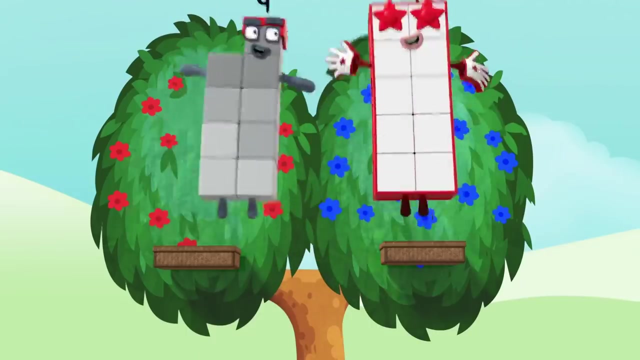 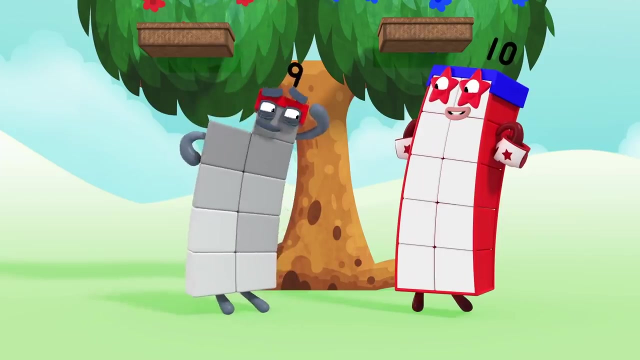 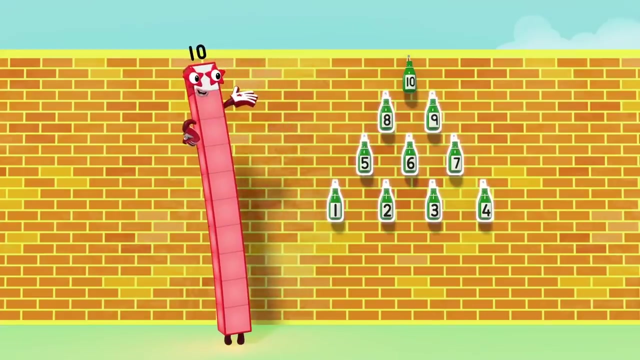 One, Two, Yay, There Hang on Eight points each. It's a draw. Woo Ugh Ugh. That was fun. Same time tomorrow. Game on: Ha ha. One, two, three, four, five, six, seven, eight, nine, ten. 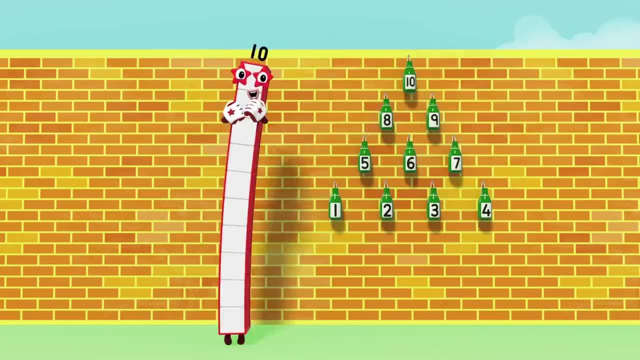 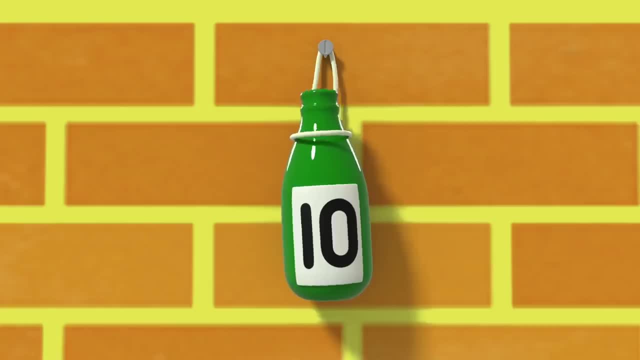 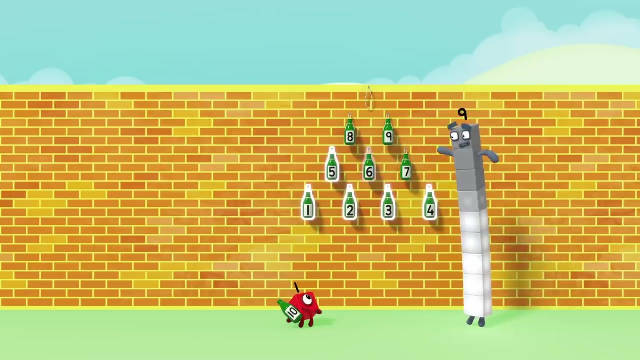 Ten green bottles, Huh. Ten green bottles hanging on the wall. Ten green bottles hanging on the wall- Huh, But one green bottle should accidently fail. There'll be one, two, three, four, five, six, seven, eight, nine. 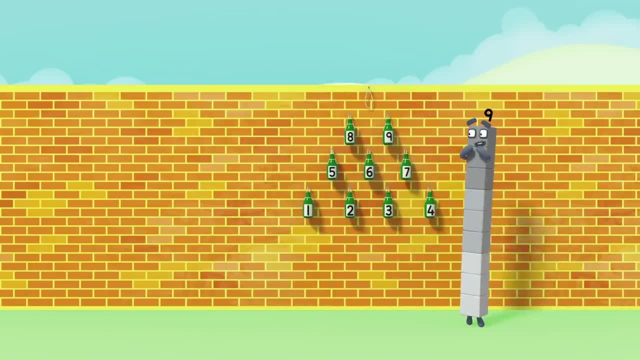 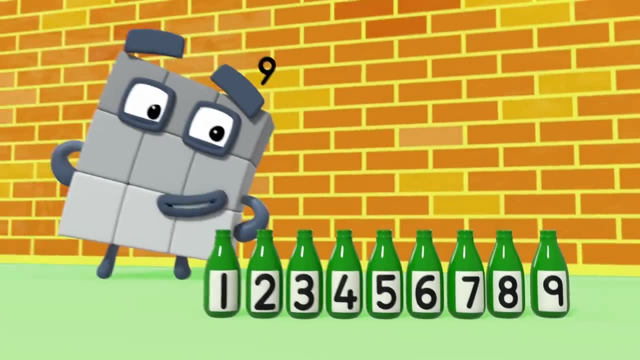 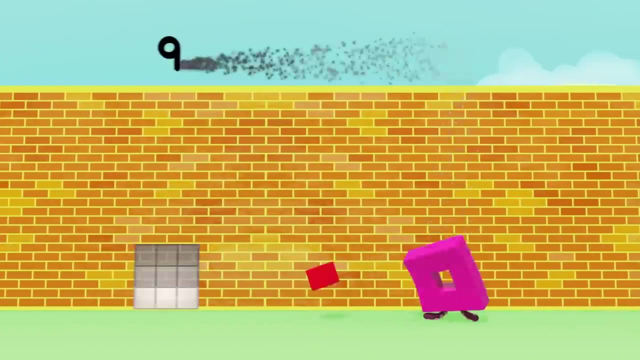 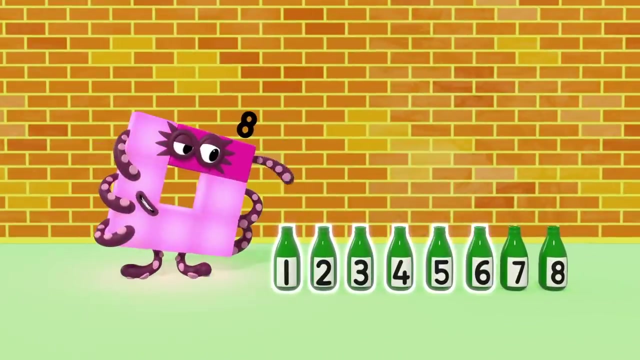 Nine green bottles hanging on the wall. Better move these nine before they fall. They're not safe up there. Nine green bottles safely on the floor. Nine green bottles safely on the floor, But if one green bottle becomes a dinosaur, There'll be one, two, three, four, five, six, seven, eight. 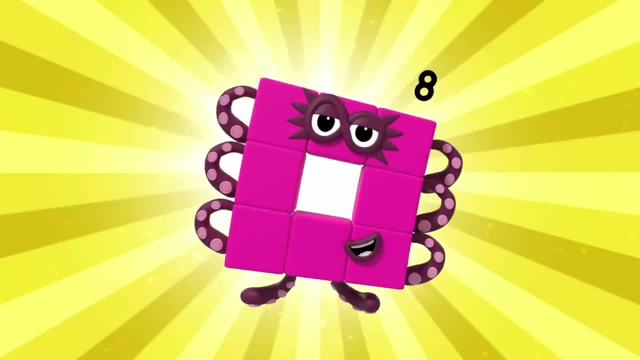 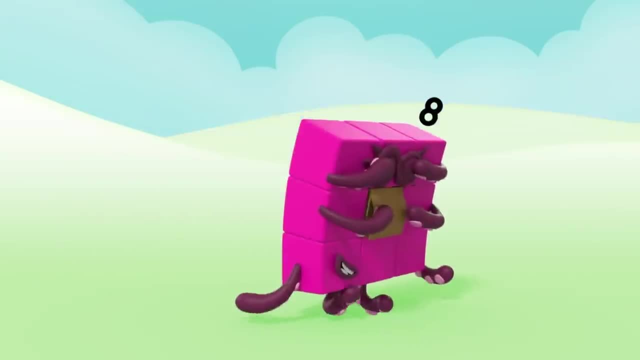 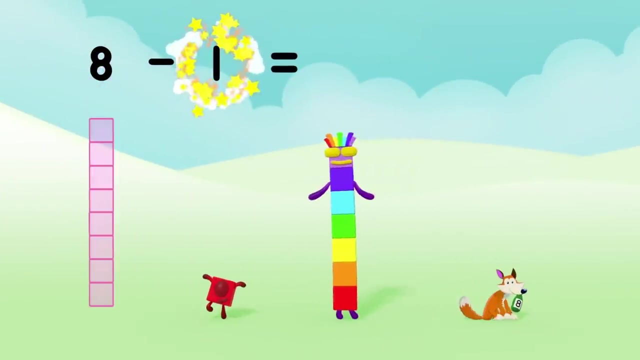 Eight green bottles not safe on the floor. Octoblock hide One, two, three, four, five, six, seven, eight. hide Eight green bottles hiding in a box. Eight green bottles hiding in a box. But if one green bottle is stolen by a fox? 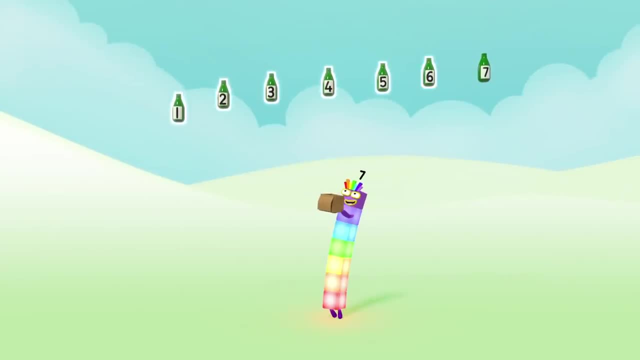 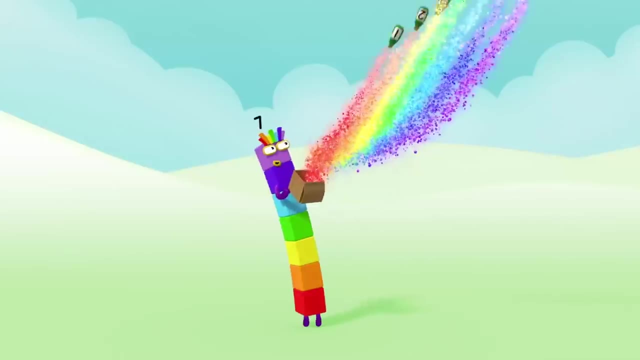 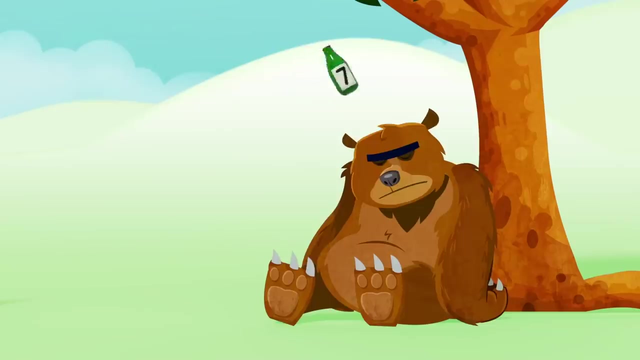 Hey, There'll be one, two, three, four, five, six, seven, Seven green bottles hiding in a box. That was lucky. Seven green bottles flying through the air. Seven green bottles flying through the air, But if one green bottle should wake a grizzly bear. 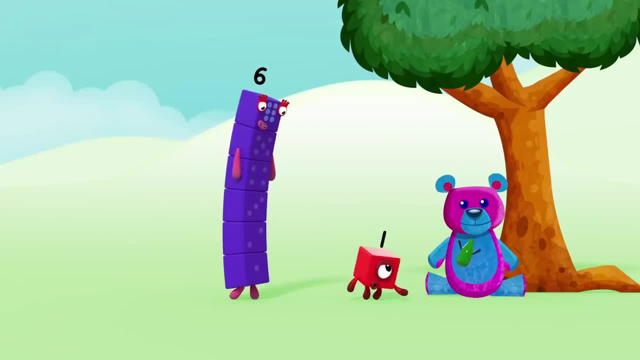 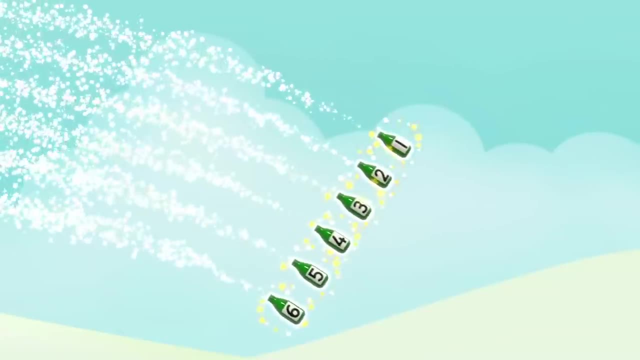 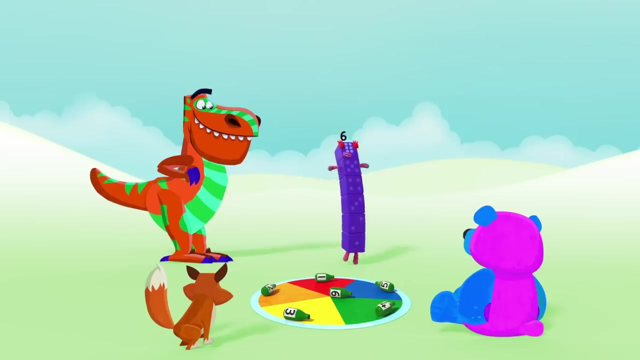 What I mean. hug a teddy bear. Phew, There'll be one, two, three, four, five, six, Six green bottles falling through the air. Six is my name. let's play a game, And this game goes like this: 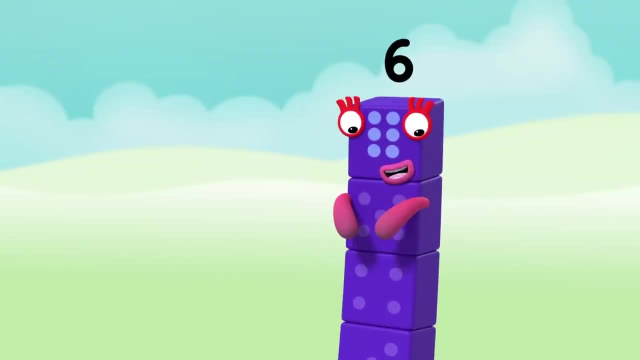 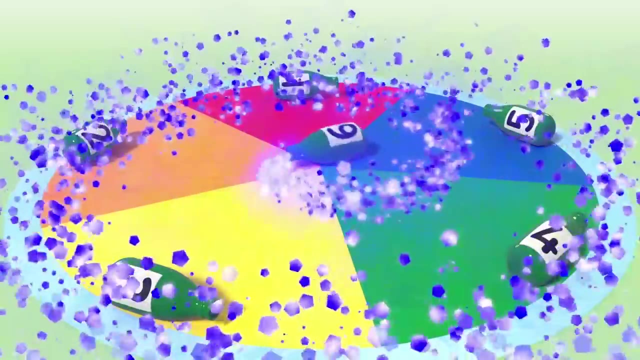 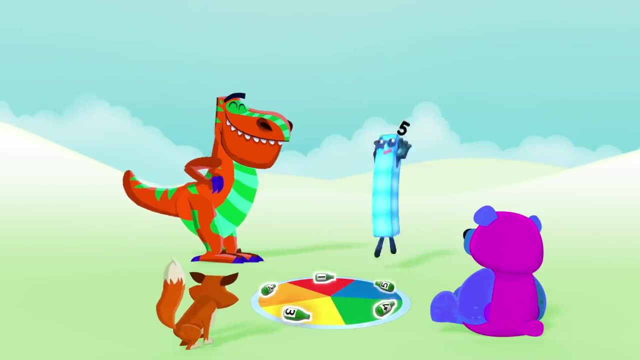 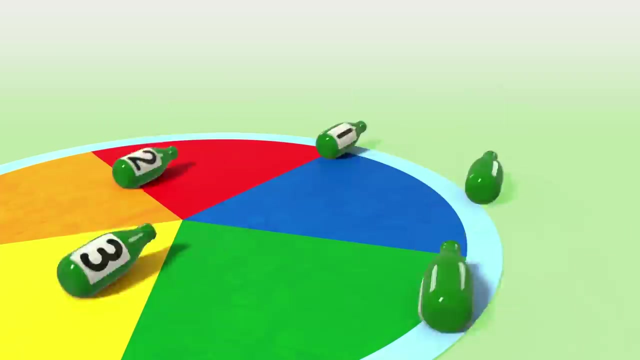 Six green bottles lying on the ground. Six green bottles lying on the ground, And if one green bottle spins around, You win. There'll be one, two, three, four, five, Five green bottles lying on the ground. Yeah, Five green bottles rolling down the hill. 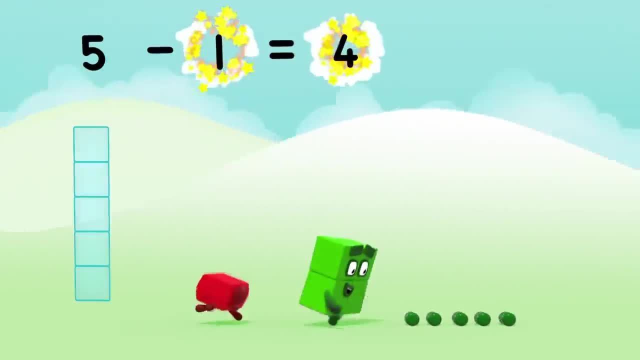 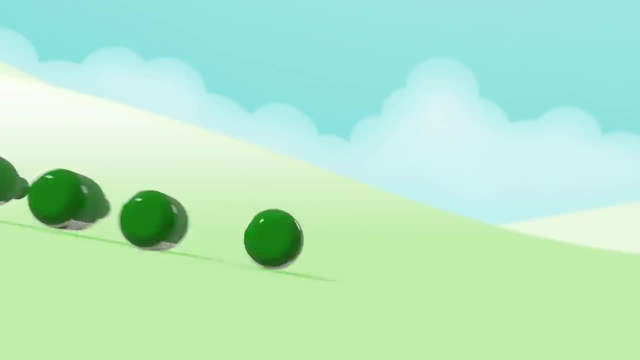 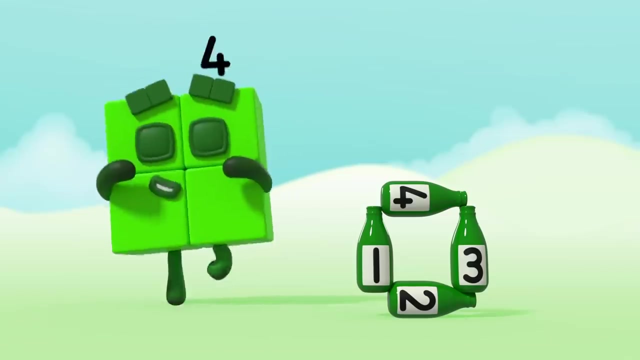 Five green bottles rolling down the hill, But if one green bottle should grow a daffodil, There'll be one, two, three, four, five green bottles Rolling down the hill. Four green bottles standing in a square. Four green bottles standing in a square. 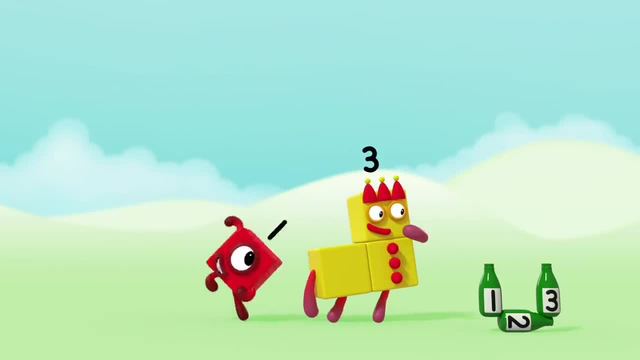 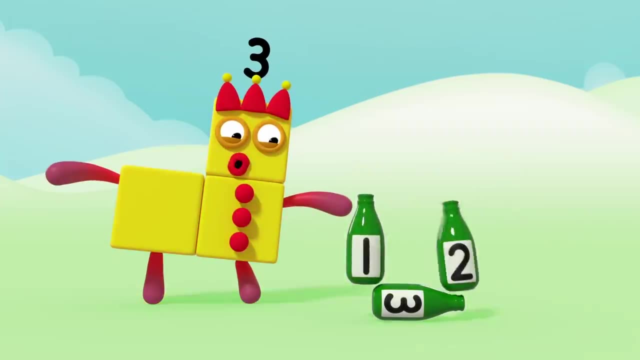 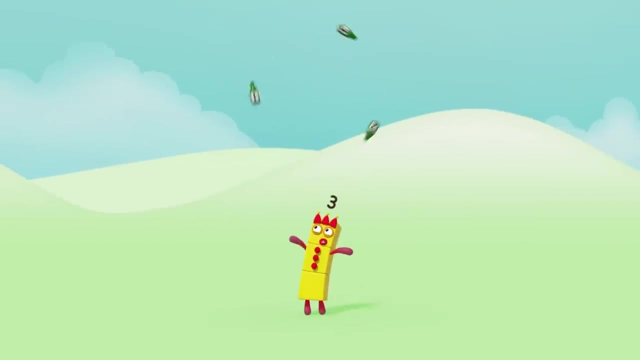 But if one green bottle should run to the bear, There'll be one, two, three, three green bottles Standing in a triangle. One, two, three, Three green bottles spinning in the sky. Three green bottles spinning in the sky. But if one green bottle should wrap its wings and fly? 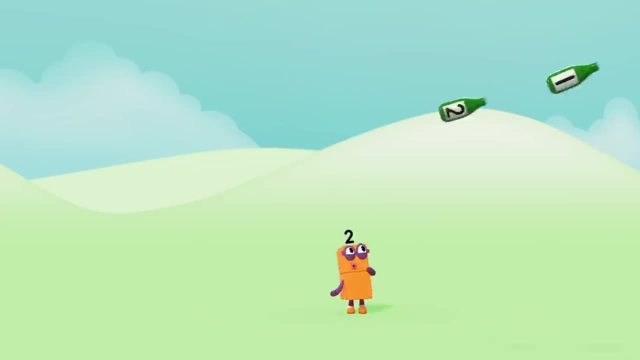 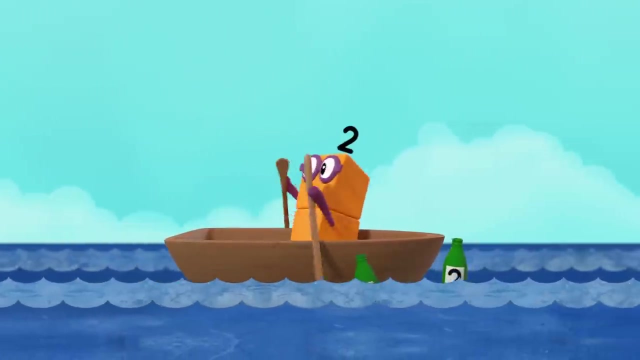 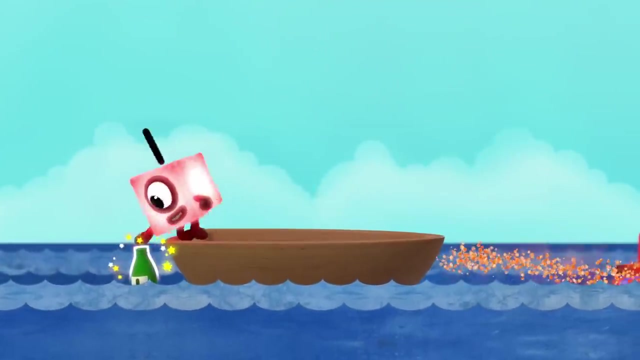 There'll be one, two, three green bottles spinning in the sky. Come back Two green bottles floating out to sea. Two green bottles, Two green bottles floating out to sea. But if one green bottle should learn to watch a sea, There'll be one. one green bottle floating out to sea. 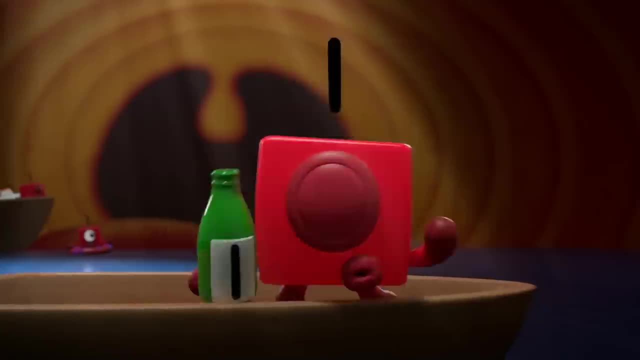 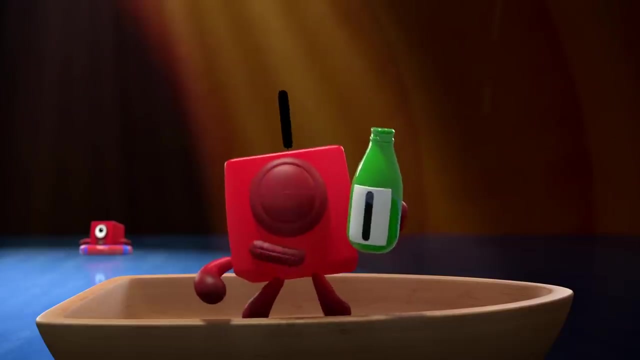 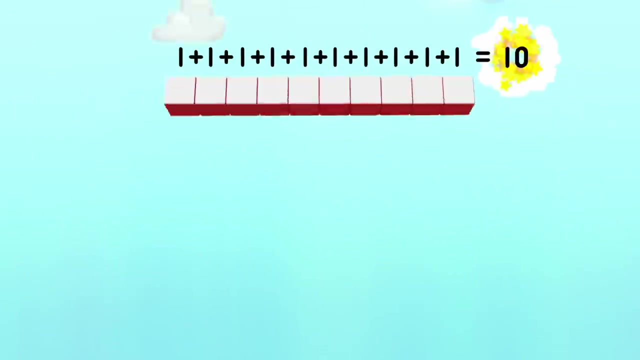 Two, three, four, five, six, seven, eight, nine, ten. One green bottle swallowed by a whale. One green bottle swallowed by a whale. But if that green bottle should grow a tickly tail, There'll be no green bottle swallowed by a whale. 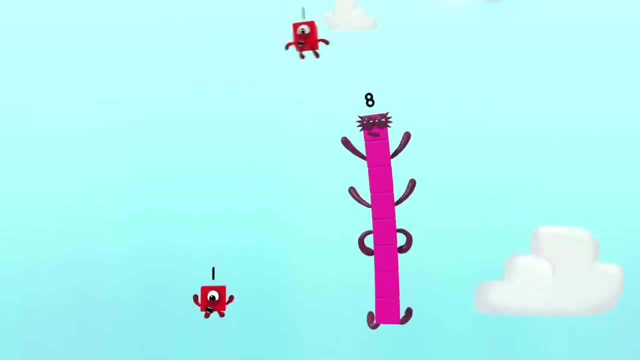 Three green bottles hanging on a wall, Slightly on the floor, hiding in a box, Flying through the air, lying on the ground. Ten green bottles rolling down a hill, Standing in a square, Spinning in the sky, Floating out to sea Swallowed by a whale. 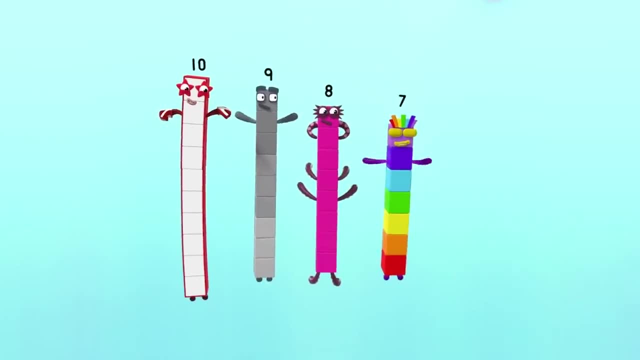 But if one green bottle should accidentally fall, Become a dinosaur, Wake a grizzly bear, Spin around up a hill, Flap its wings and fly, Learn to water-ski, Grow a tickly tail. There'll be nine, eight, seven, six, five green bottles hanging on a hill. 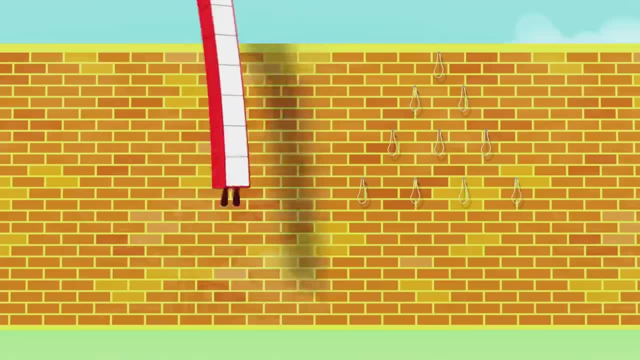 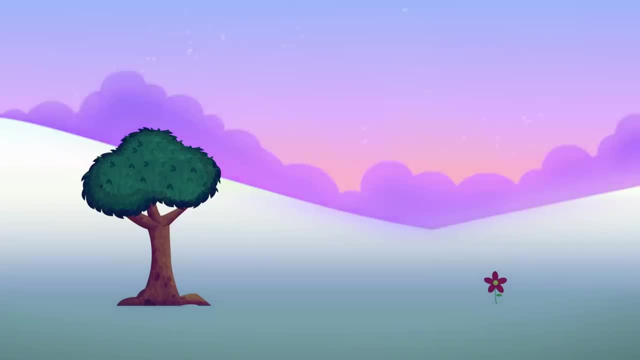 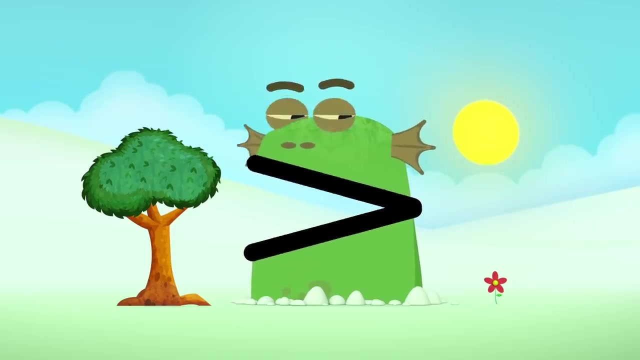 Standing in a square: Seven, six, five, four, three, two, one, No green bottles hanging on a wall, Me Bloxzilla. Me like big things. Which is bigger? Tree is bigger than flower, Me like tree. Nice to meet you, Tree. 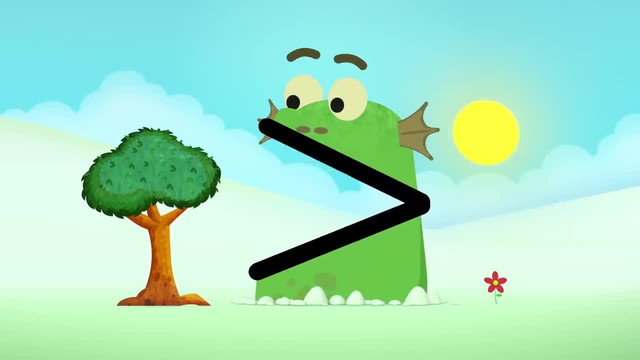 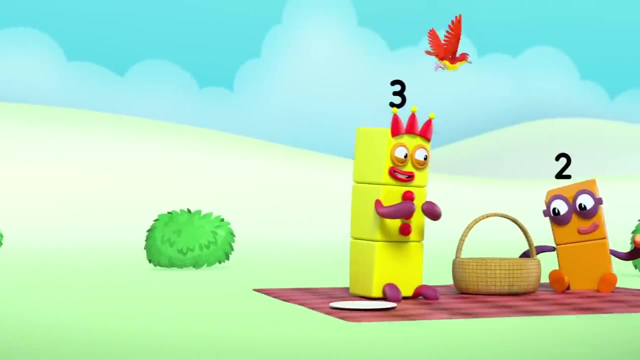 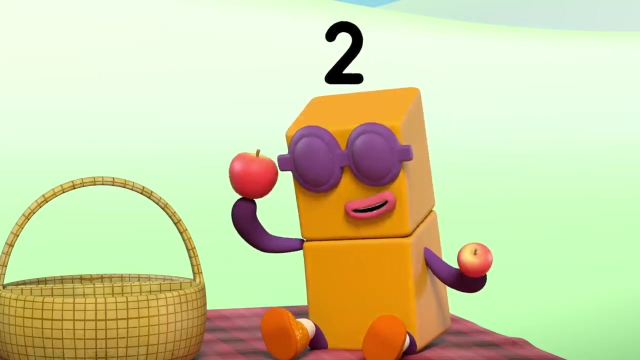 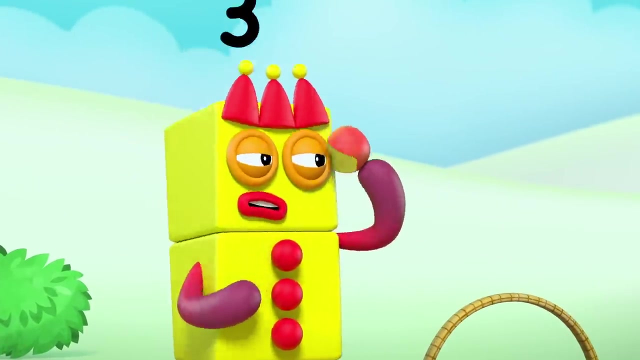 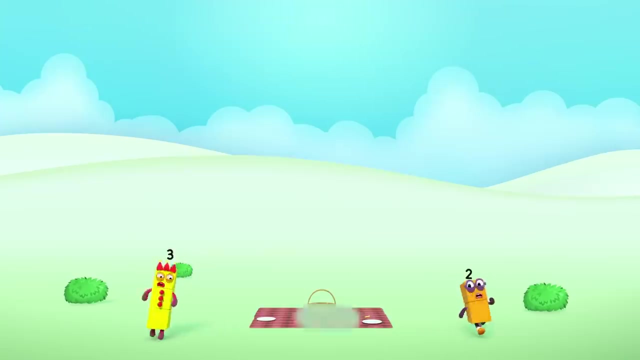 Will you play with me? This apple is bigger than this one And you're bigger than me, So you have it Tree. Thank you Two. I like apples. I like to munch them And crunch them And gobble them up, Me Bloxzilla. 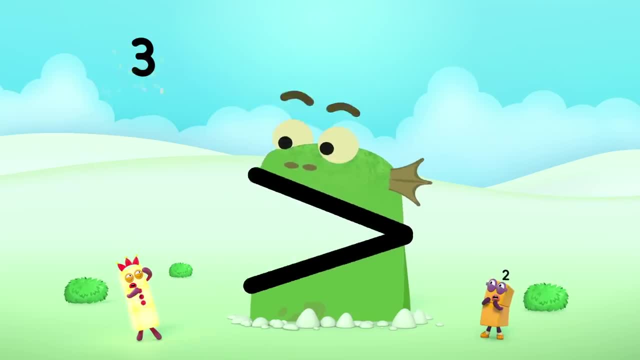 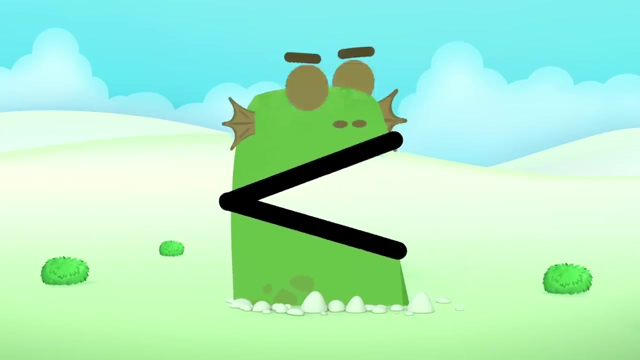 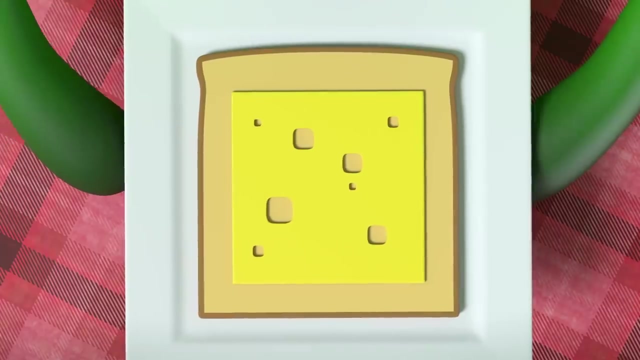 Three has more blocks than two. Three is greater than two. Greater means bigger. So me like three, Don't gobble me up. Oh Me, don't eat you silly. Me like you, I like square cheese. I like it in my tummy. 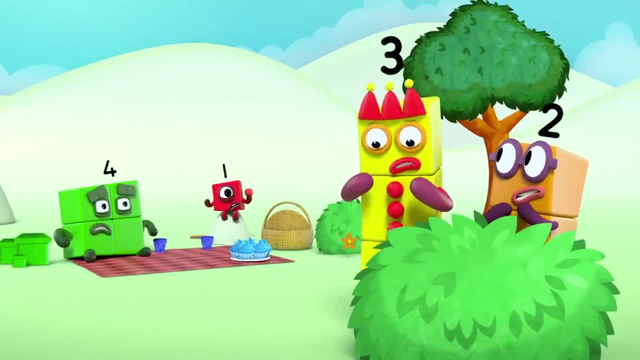 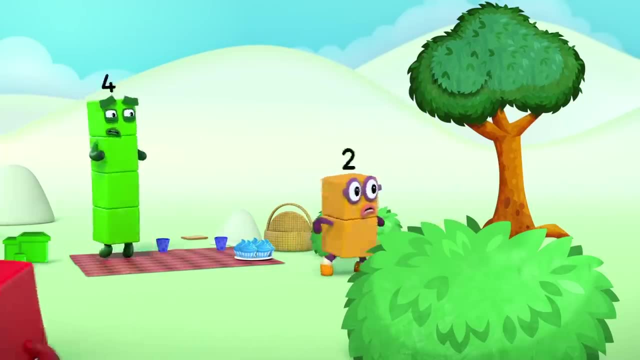 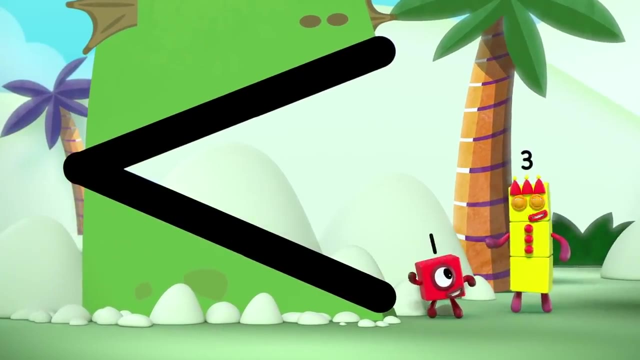 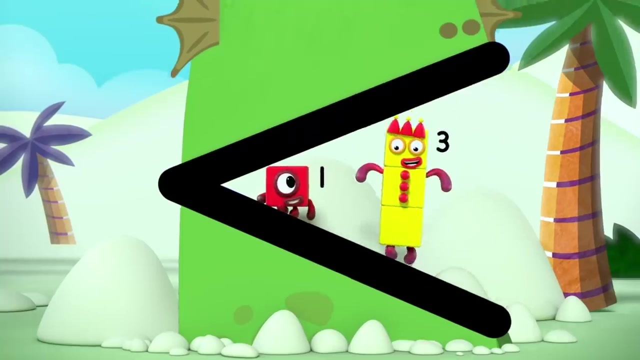 There's a monster. It wants to munch us, crunch us, gobble us up, Run Hide. Look A cave We can hide in there. You go first. One: You're smaller than me. We should be safe in here. One is less than three. 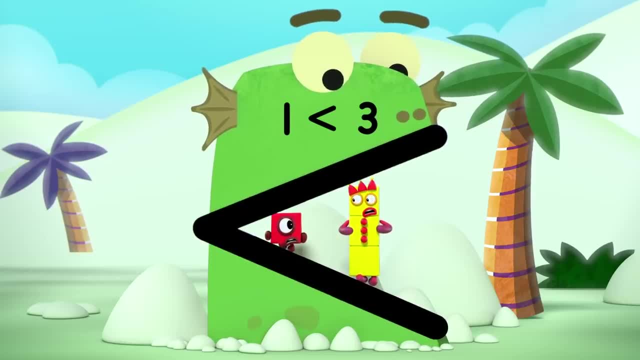 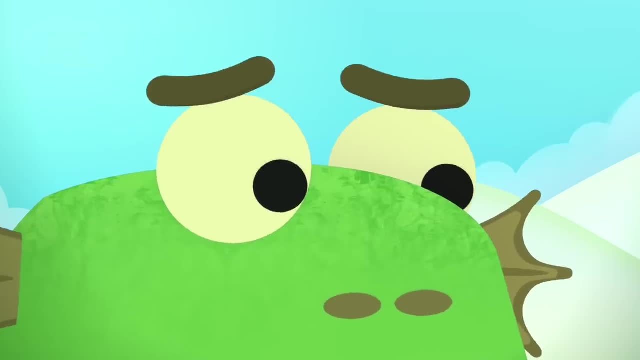 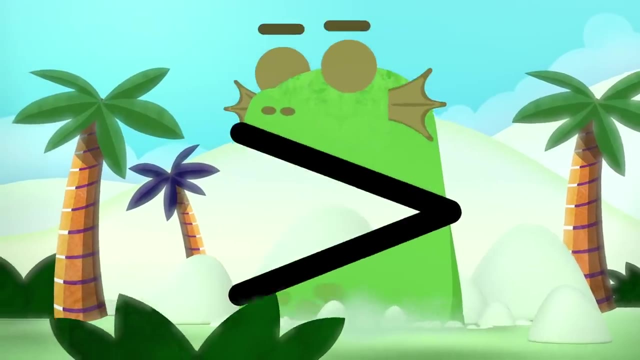 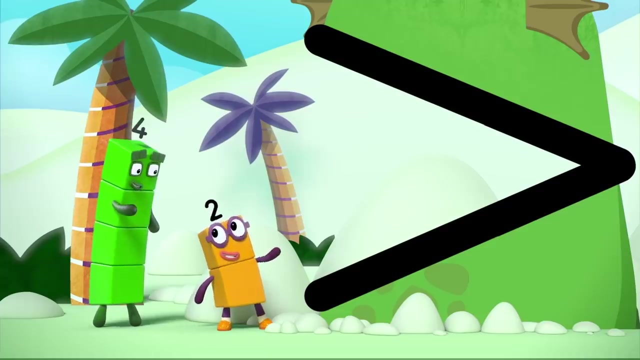 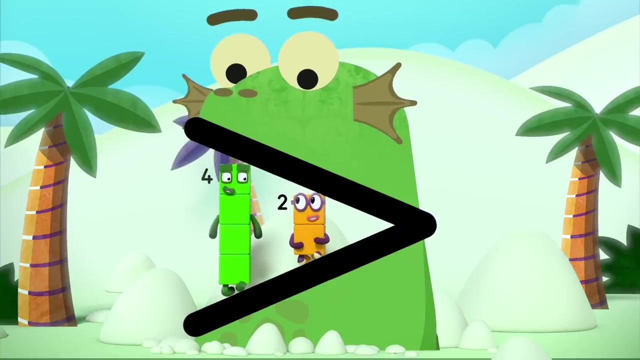 Me like bigger numbers, So me like three: Stop Four Me. want to meet you? No, Not eat you. Where can we hide? Look A cave, You go ahead. Two: I'm bigger than you. We should be safe in here. Four is greater than two. 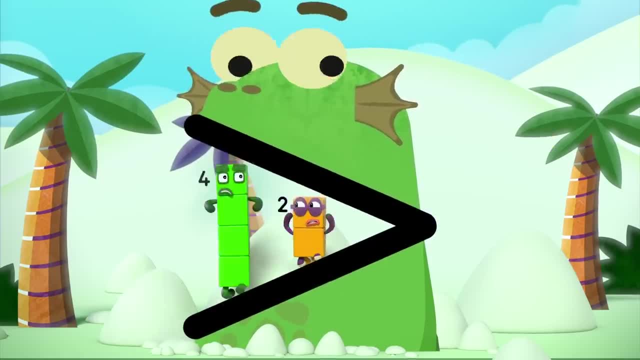 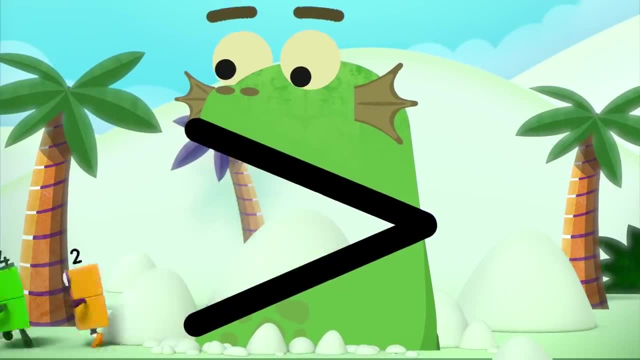 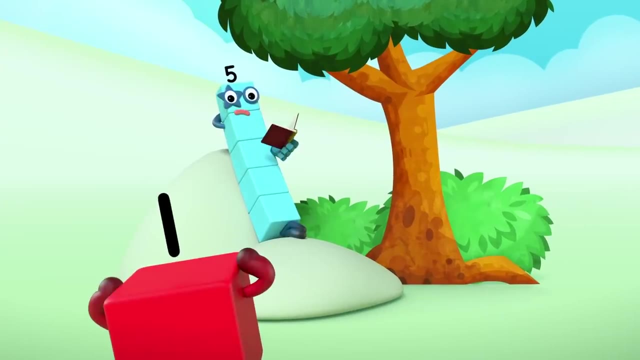 So me like four, Like I like square cheese In my tummy. Ahhh, No Silly, There's a monster. It wants to munch us, crunch us, gobble us up In its tummy, Oh dear. 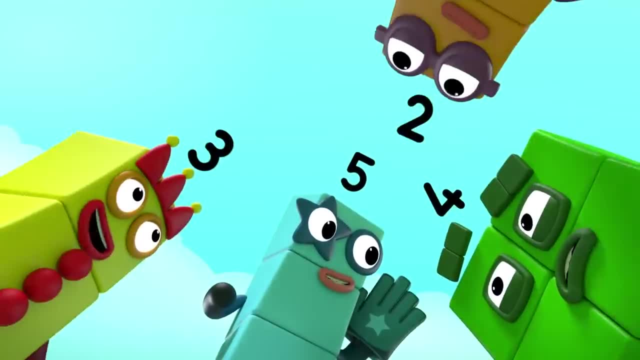 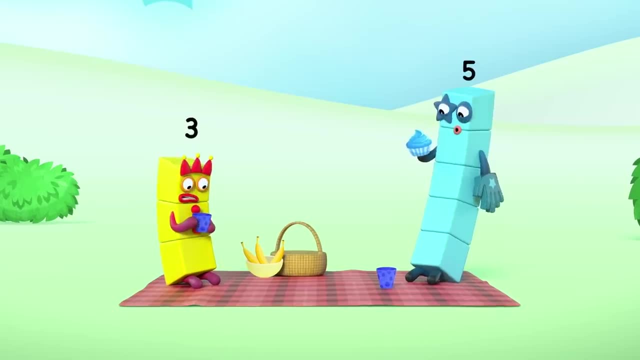 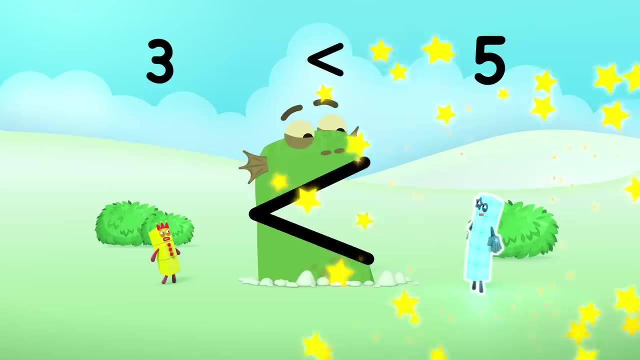 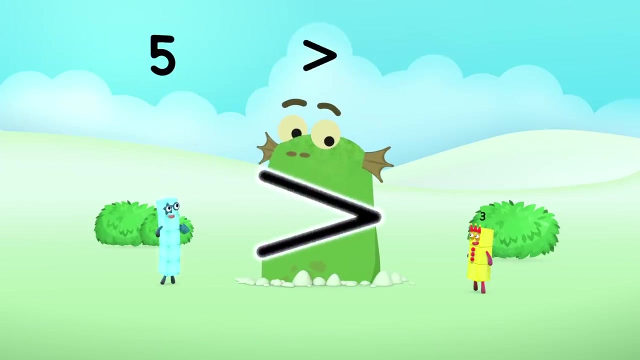 Sounds as if we need a plan, And I think we should. Well, what if I carry you? I'm doing it. Well, I guess Three is less than five. Me like five. Me mean five is greater than three. Me like five. 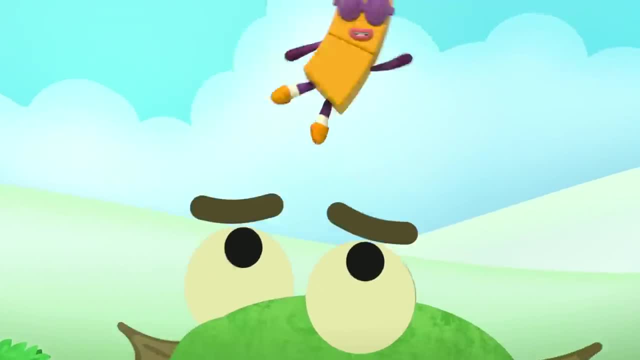 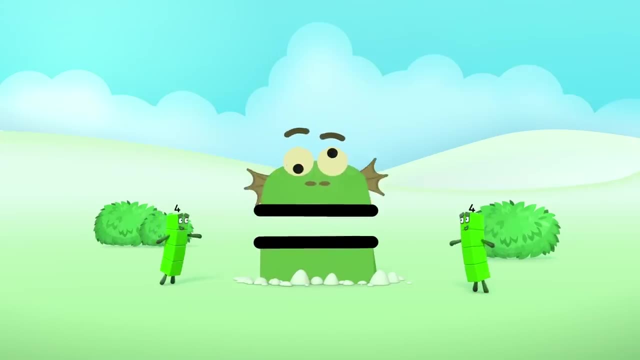 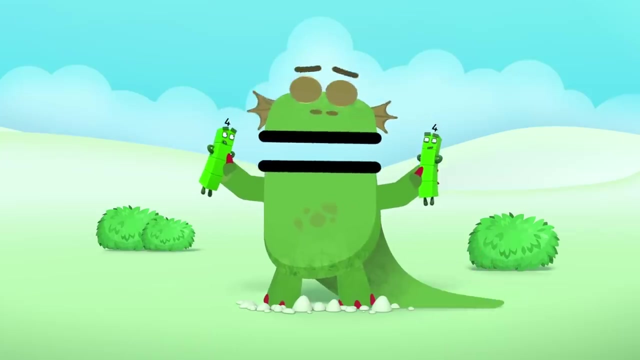 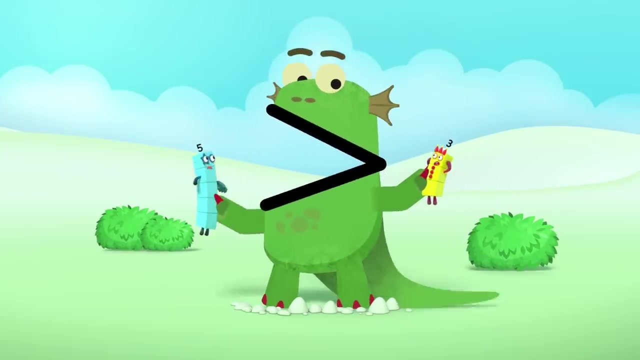 Three is less, Five is greater. Three, Five, One. We're both the same. Four equals four. You can't eat us now. Me no like to eat you, silly. What me like to play with you, Play with us. 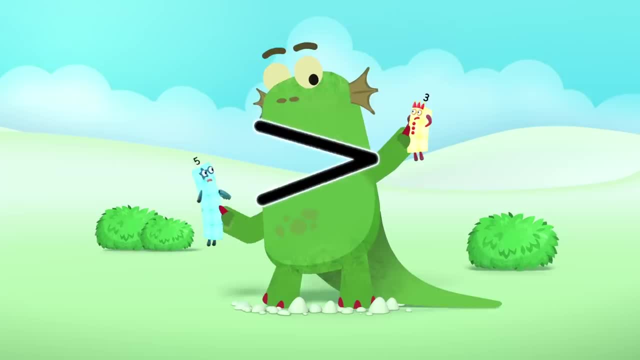 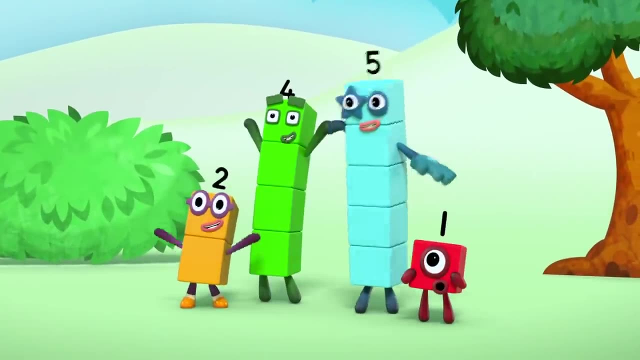 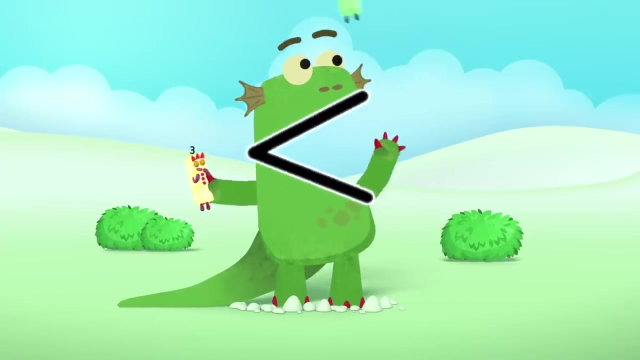 Five is greater than three. So Bloxzilla play with five. What Hooray, Play with me. Me too. Me too, Bloxzilla play with number blocks. Three is less than four. Three is greater than two. One is less than two. 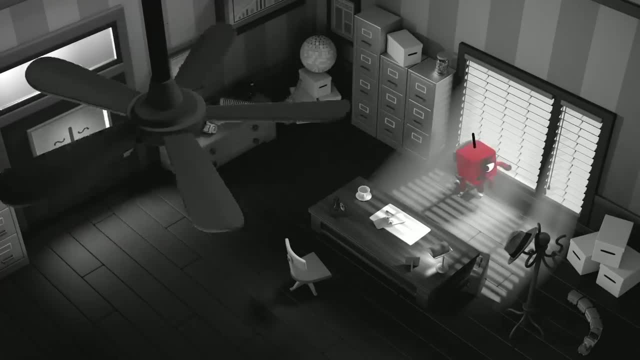 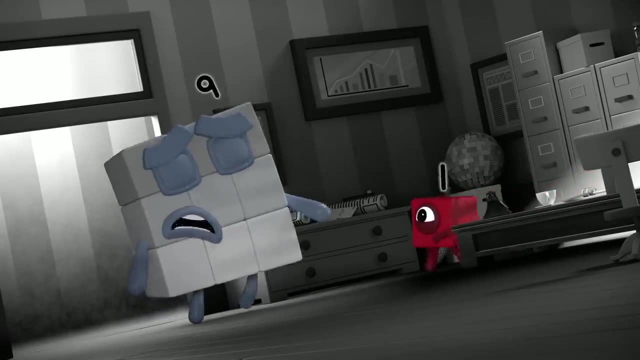 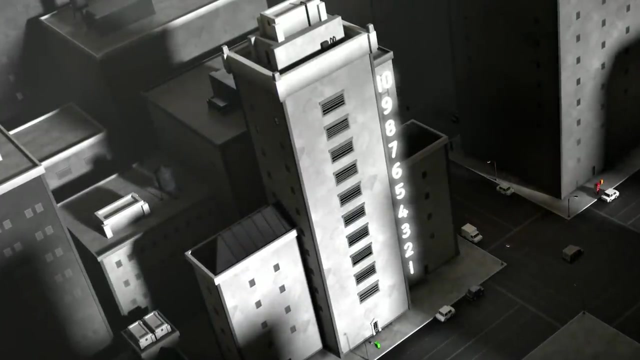 That was a great day in the big city. I was wondering where my next case would come from when You've got to help me. One It's gone, Everything's gone, Slow down. Nine: Tell me what happened. I live in apartment nine on the ninth floor of numerical towers. 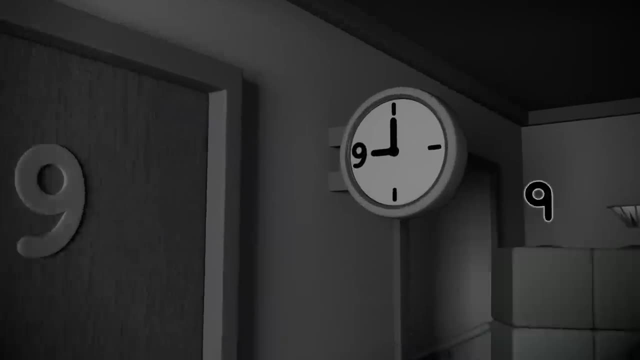 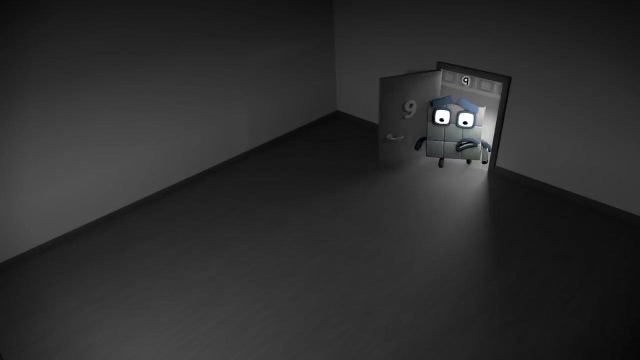 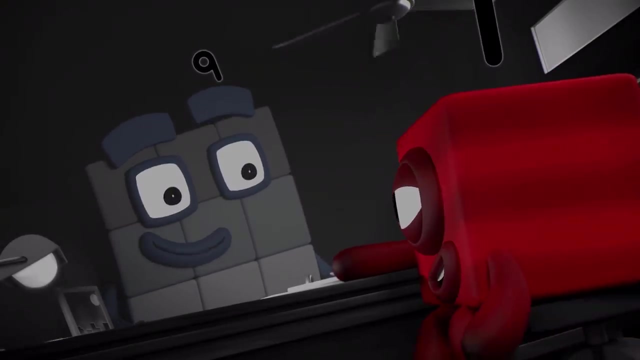 I left home this morning at nine o'clock to buy a newspaper. When I came back nine minutes later, the door was open. Everything was gone. A mystery indeed. I'll take the case. Let's look for clues. Did you notice anything strange or unusual when you got back? 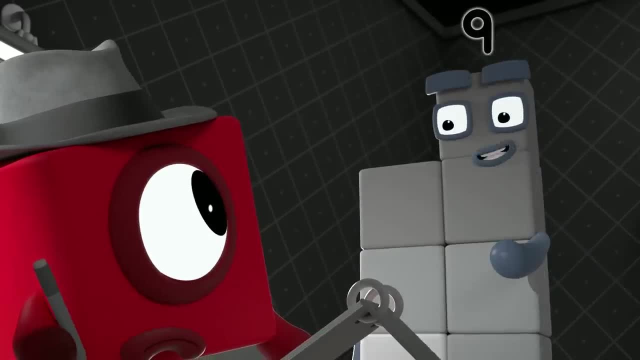 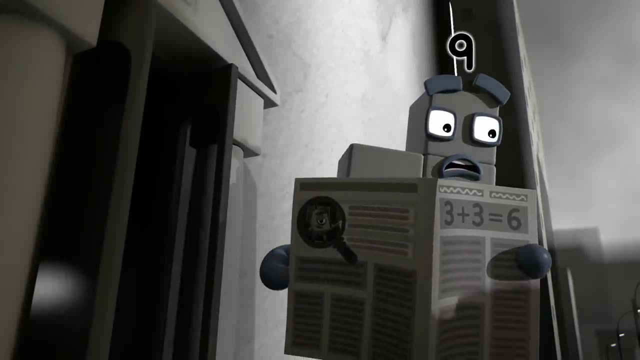 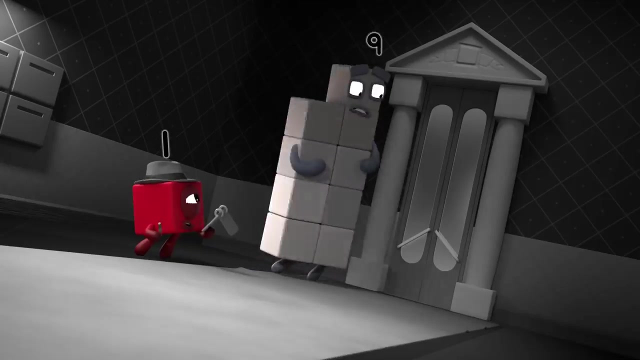 Er, no, nothing. Oh, there was one thing: A suspicious shadowy stranger in a coat and hat pushed past me and ran out of that door, But apart from that, nothing. Can you describe this stranger? They were as wide as the door, so two blocks wide, with a flat head. 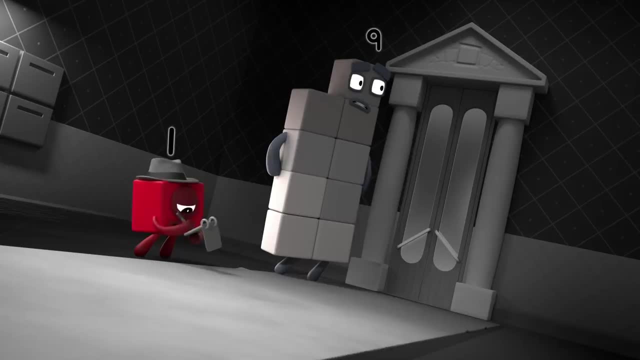 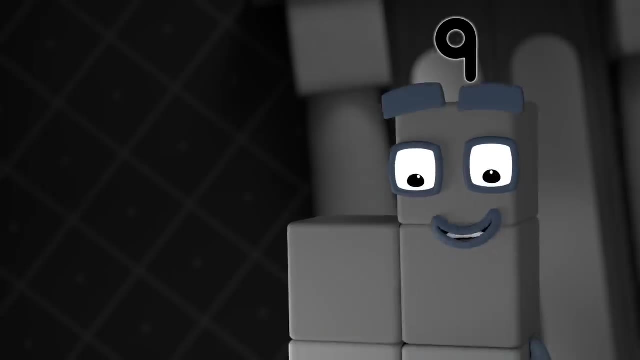 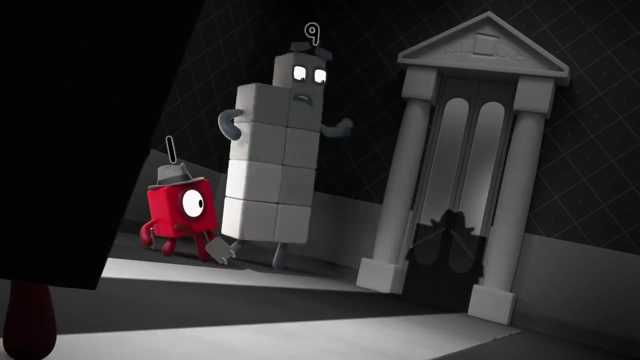 Clue one: Flat head when standing two blocks wide. Anything else I could see over their head when we were both two blocks wide, so they must have been smaller than me. Clue two: Smaller than nine. Look, Hat, Coat, It's them. 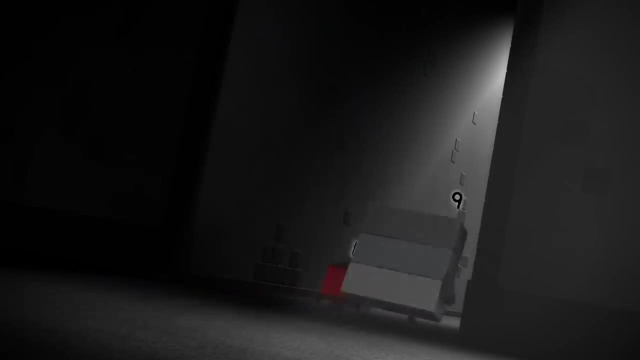 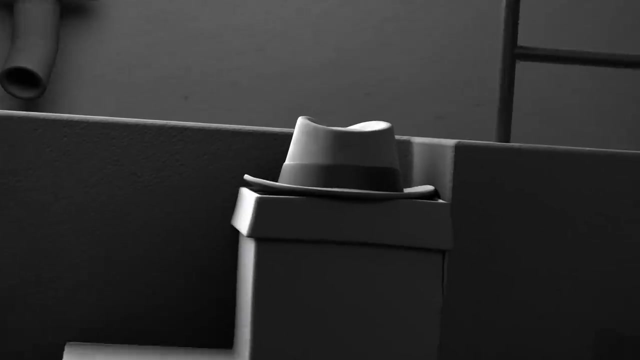 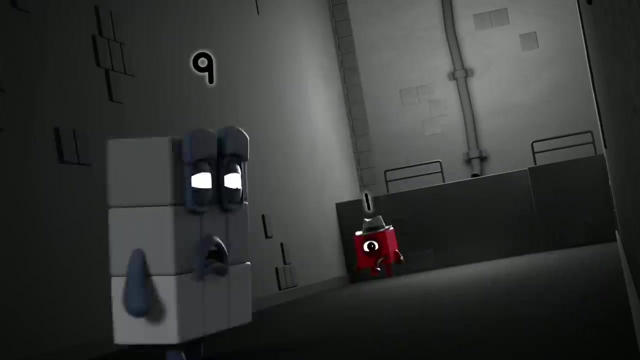 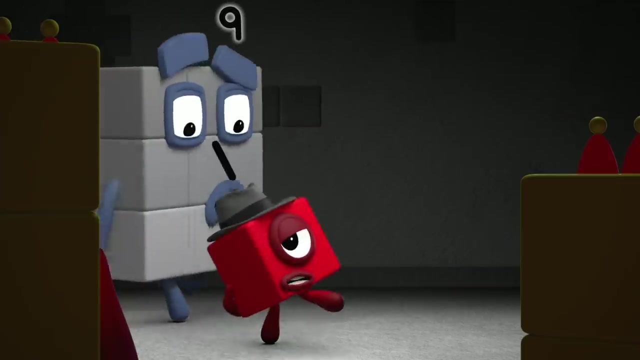 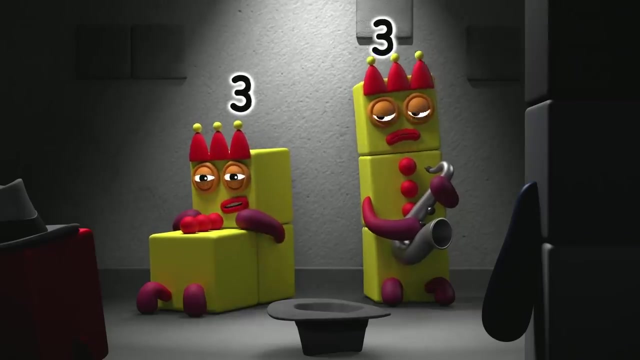 After them, Quick What There? On the steps, The hat, These aren't steps, It's. Did either of you see a suspicious step-shaped figure in a coat and hat? Sorry, friend, No one else down here, Just us. 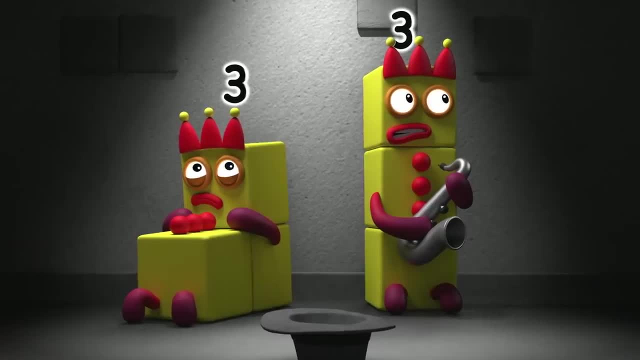 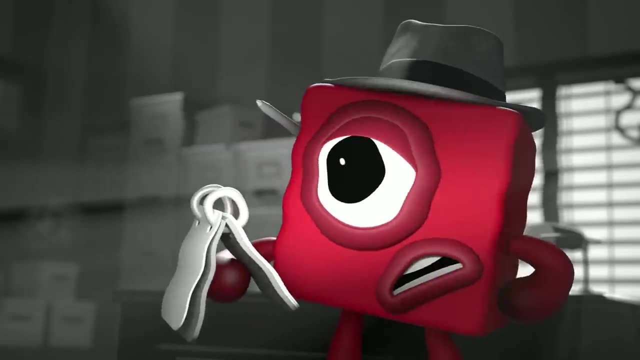 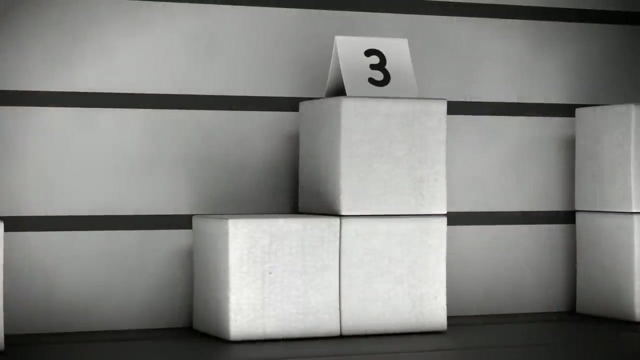 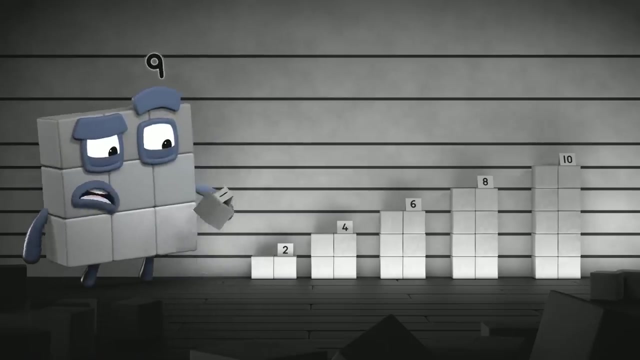 Something didn't add up, Ordid it. Let's look at what we know. Clue one: The suspect had a flat head when standing two blocks wide, So it can't have been three, five, seven or nine And it wasn't you, because you can't stand two blocks wide. 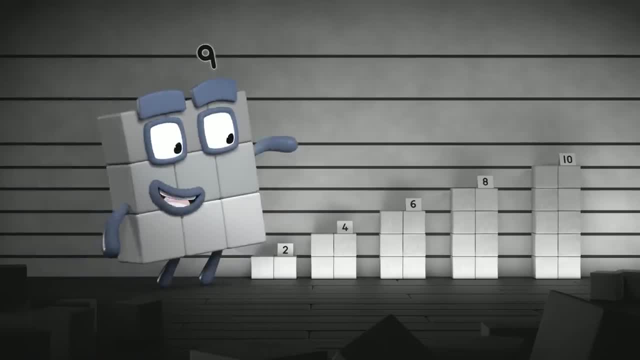 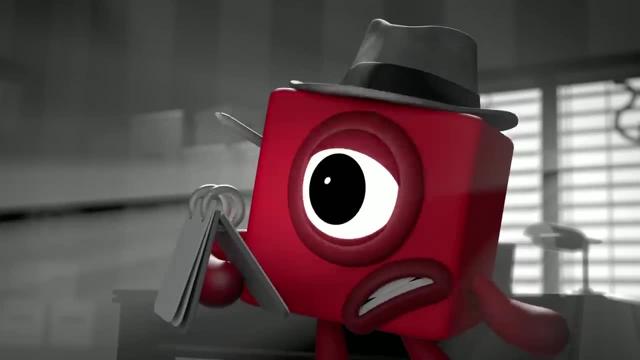 Two, four, six, eight, ten. The suspect must be an even number. Bingo And remember clue two. The suspect was smaller than nine, so it can't have been ten. That still leaves two, four, six and eight. 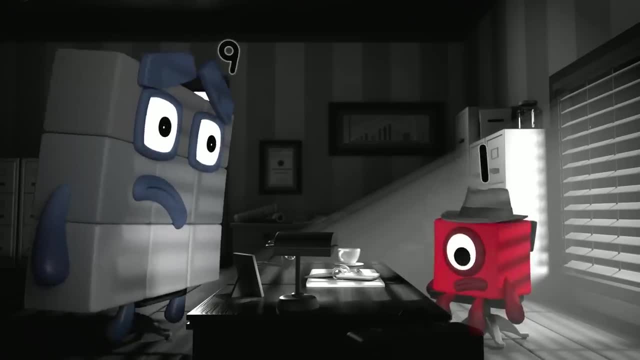 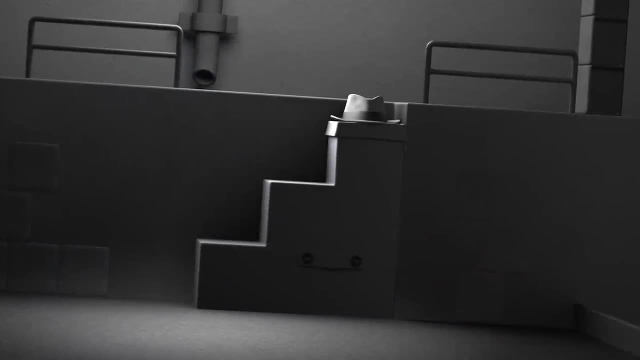 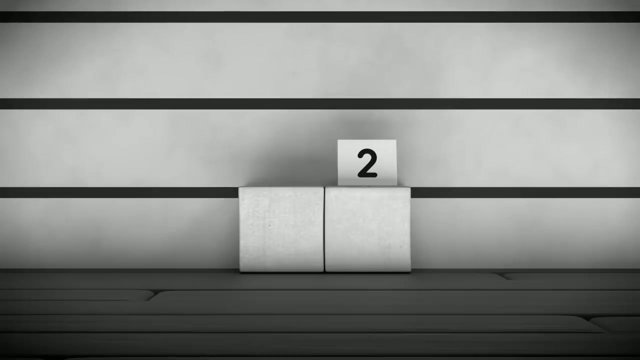 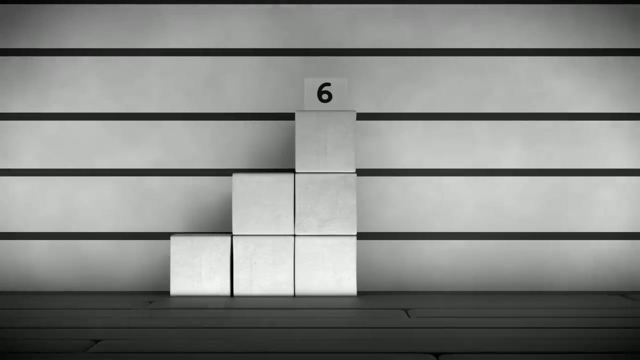 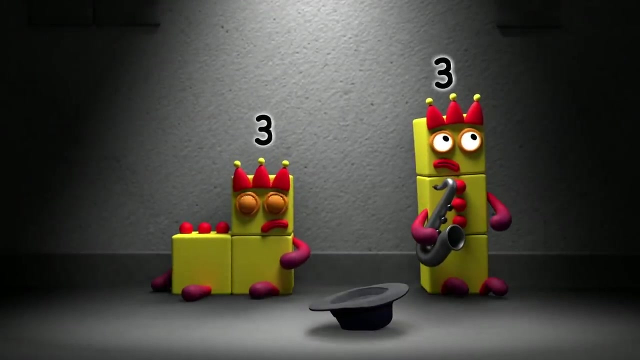 But which was it? Wait, There's one more clue, we nearly forgot: The suspect can make a step shape, Not two Or four Or eight, So it must have been Six. And who did we meet in the alley? Three And another three. 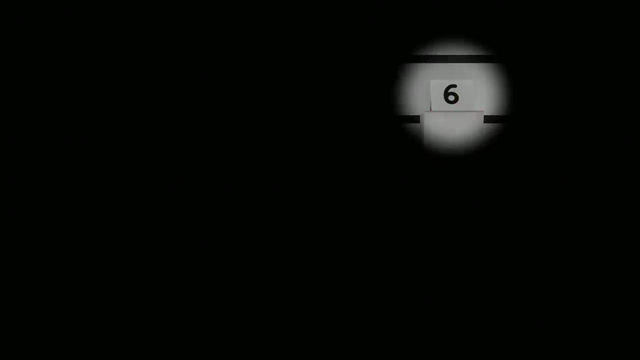 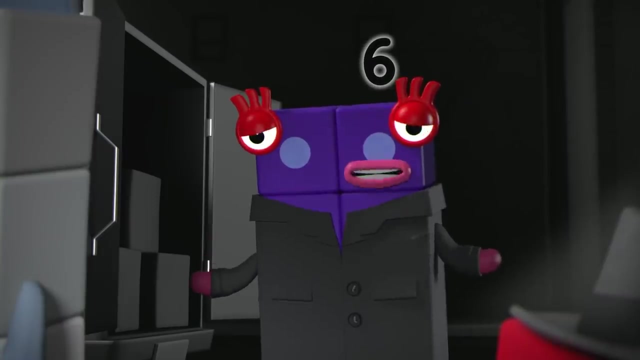 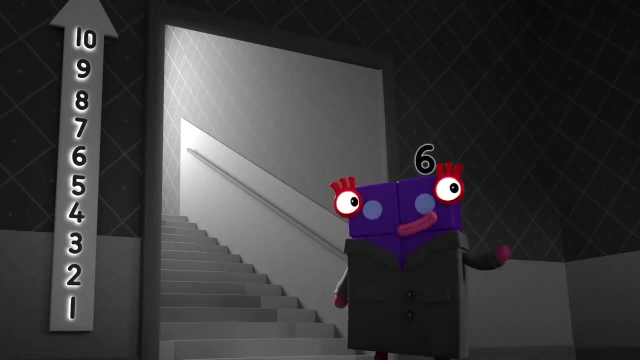 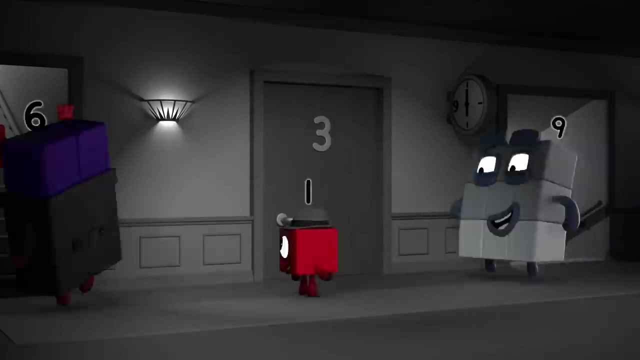 Equals six: Stop thief. You've got it all wrong. Where to begin? I'm not taking these things, I'm moving them in, Moving in. Come up and I'll show you One, Two, Three, Four, Five. 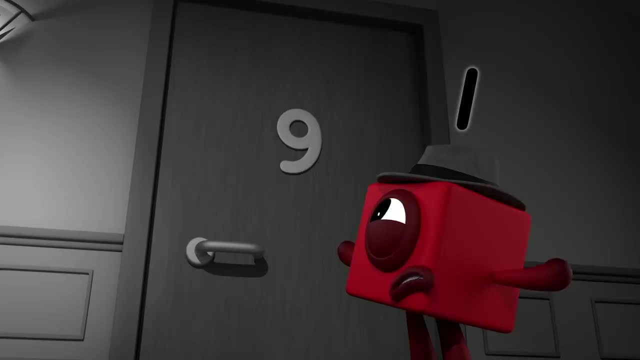 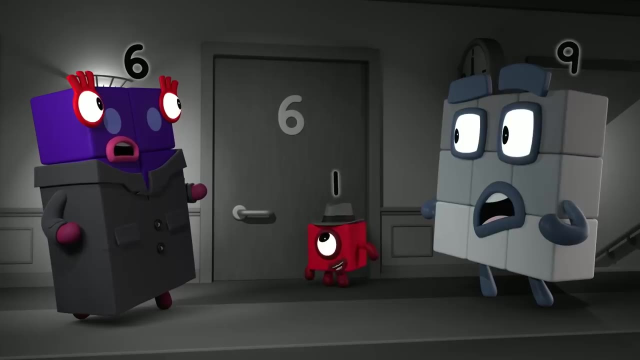 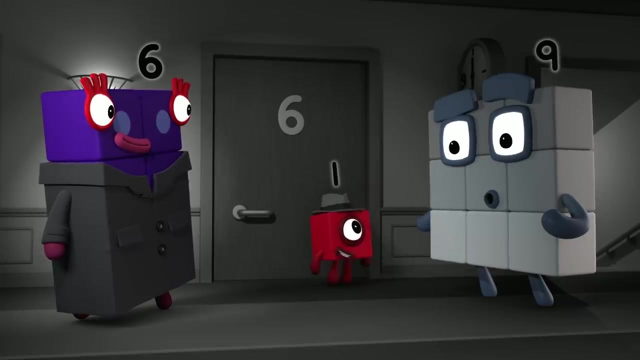 Nine. Wait, Nine doesn't come after five. This isn't apartment nine, It's apartment six. Look Number six turned upside down looks like a number nine. Oh, No one stole your things. nine, You went into six's empty apartment. 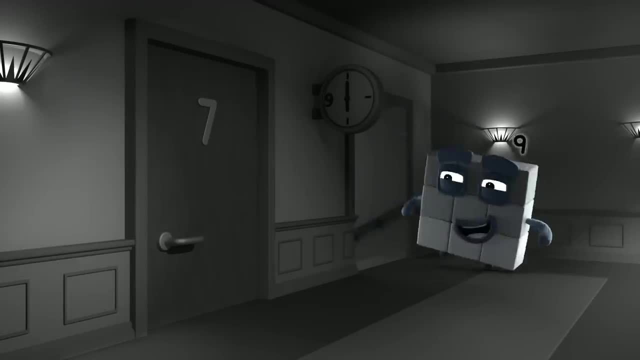 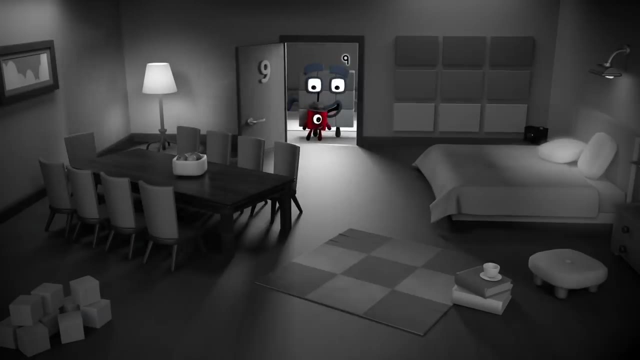 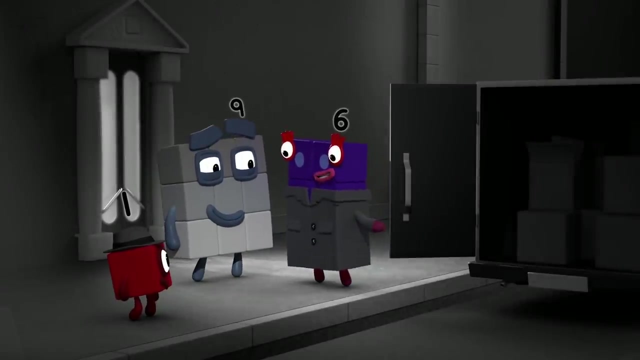 So my things must be Right where I left them. Case closed. Sorry, we chased you six. I thought that you were after me. That's why I hid as three plus three. Let's make it up to you by helping you move in. 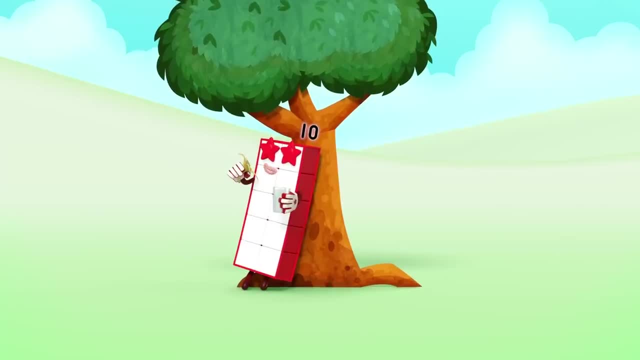 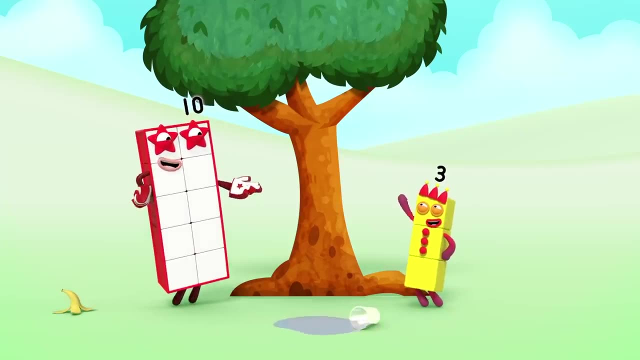 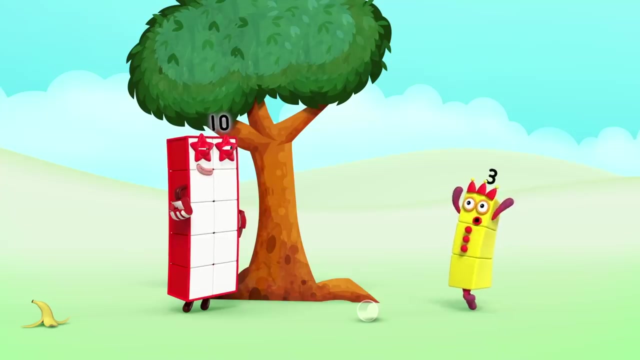 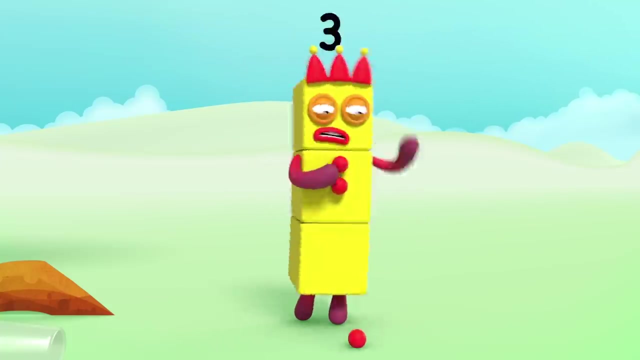 Welcome to the big city. Three, Oh Sorry, ten. I'm just so excited to show you my new trick. Look at this. Oh, Is that it? No wait, I'm not having much luck with my today. 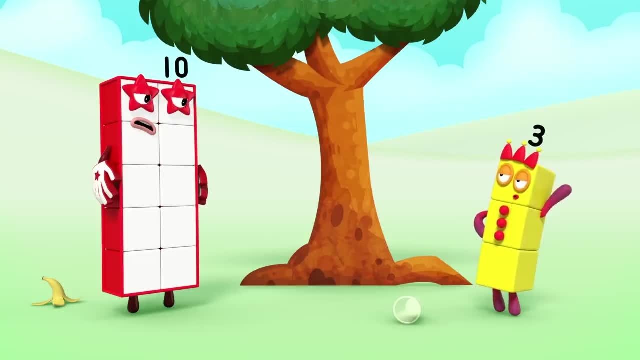 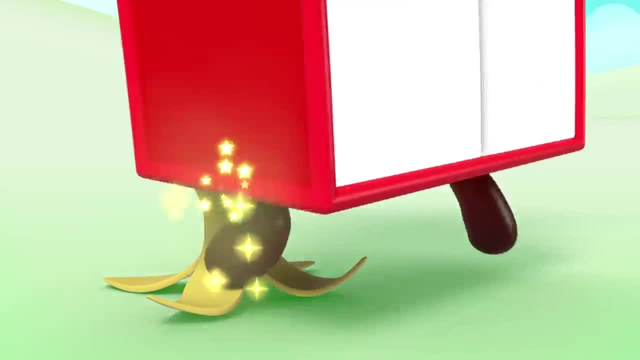 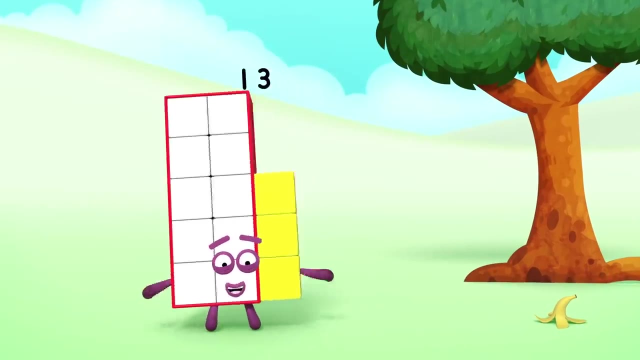 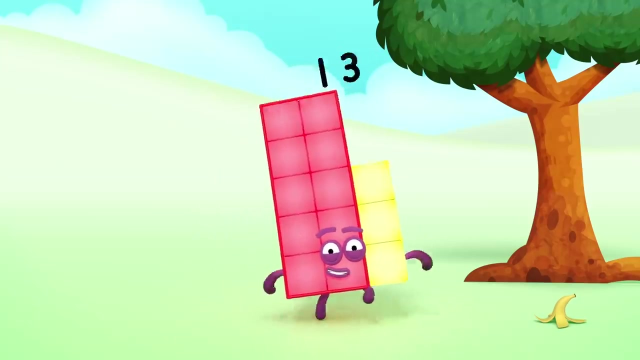 Oh no, My new trick: Ready, steady go, Oh unlucky. Oh Hi, Who am I? I'm one, two, three, four, five, six, seven, eight, nine, ten, eleven, twelve, thirteen. 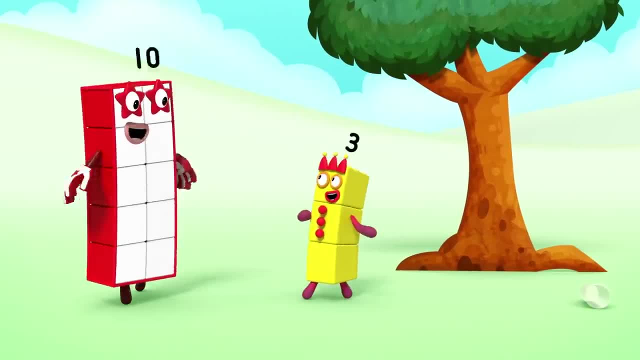 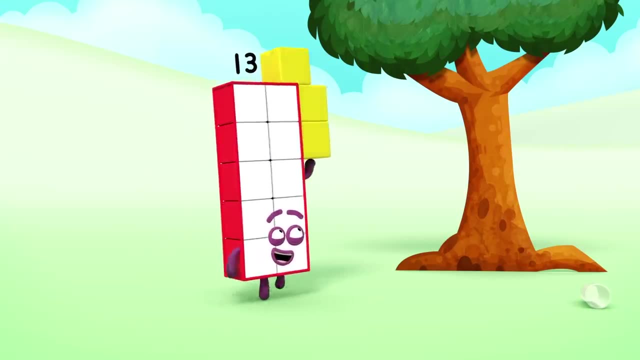 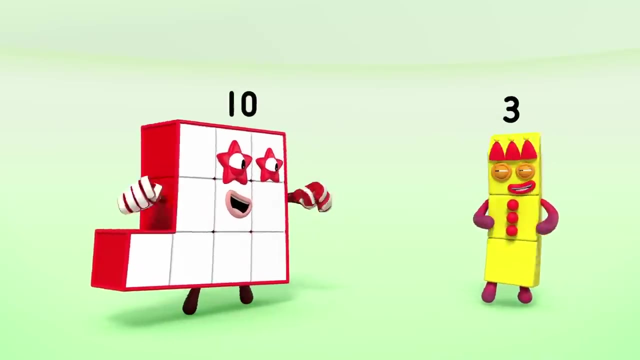 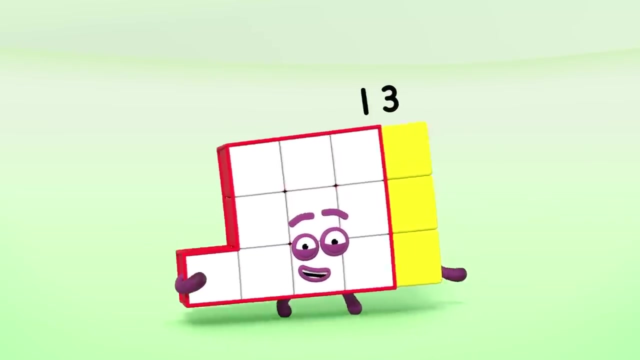 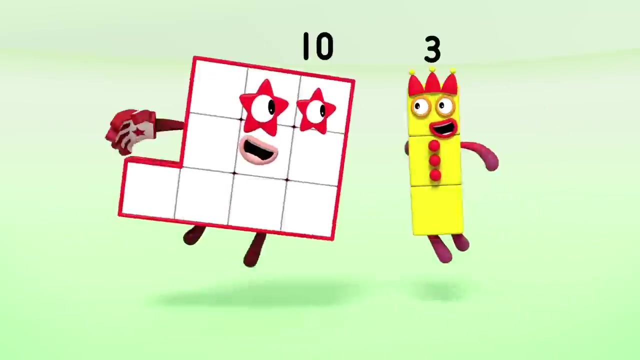 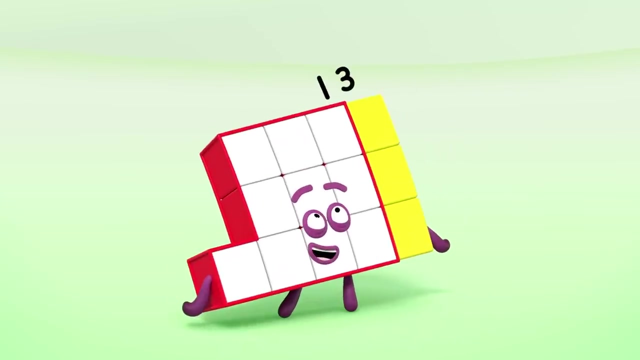 Whoa Wow. Oh, My three fell off. Never mind, I am thirteen. Oh, whoa, Unlucky. Try again. I am thirteen, Hooray, And I think I might be a little bitunlucky. 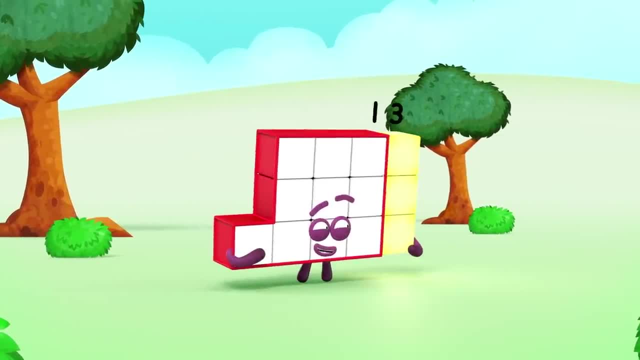 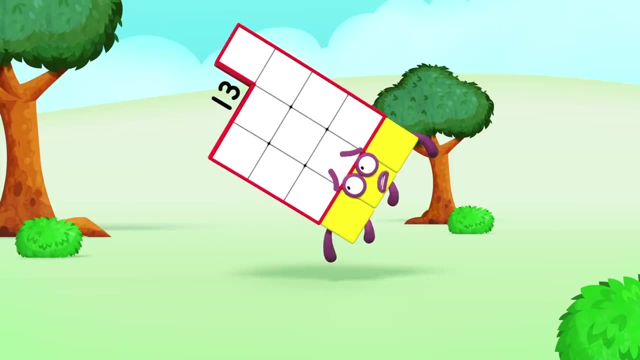 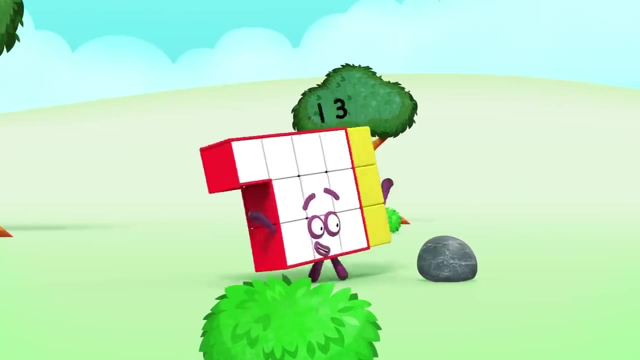 This is me, Ten and three, Expecting to run out of luck. Sorry, It's all jolly japes. when I get into scrapes I'm always coming unstuck. Oh, The clumsiest number you've ever seen. Unlucky. 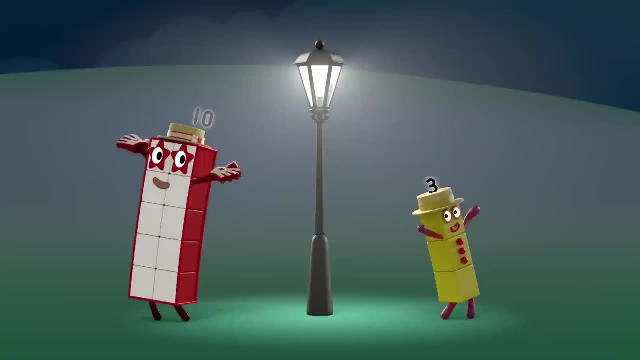 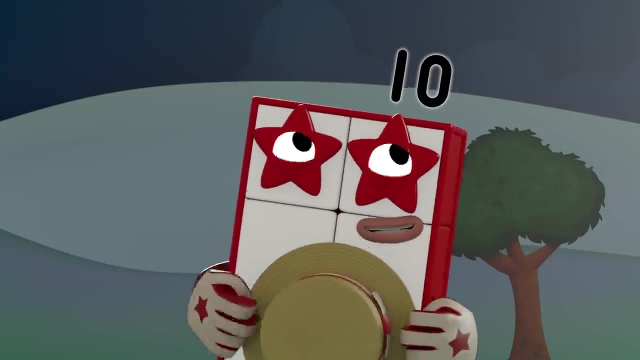 Number thirteen. It's happened again. A three and a ten. Somebody should tell him that it's happened again. I don't have the heart to be fussy or picky, But he's falling apart. He's a bit unsticky. 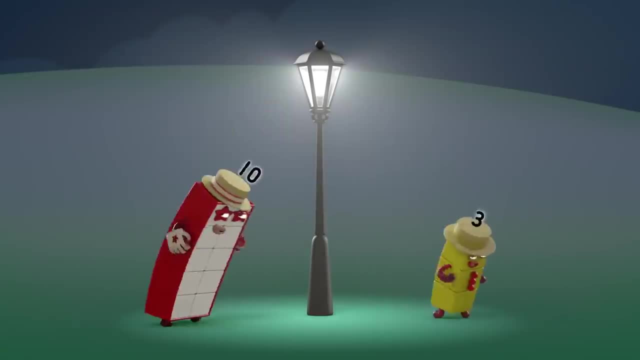 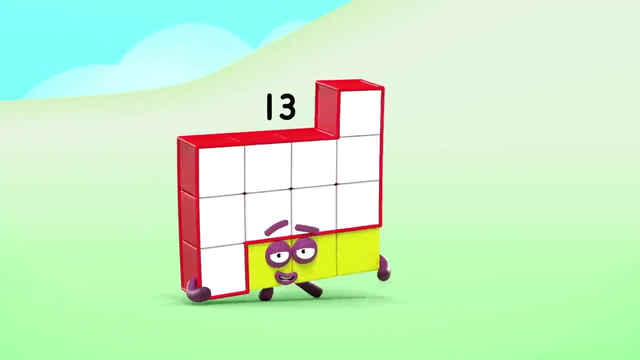 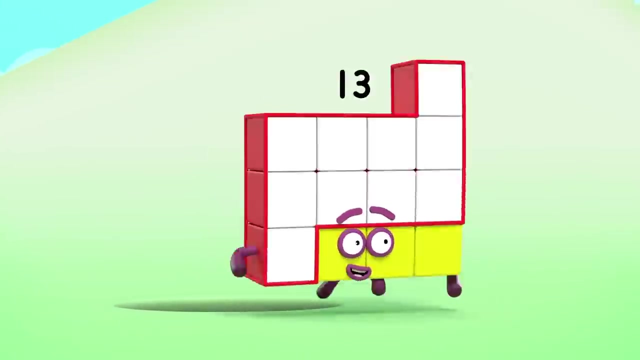 It's happened again And no one knows when Somebody should tell him that it's happened again. Me again, Three and ten, Expecting to fall down a hole. Ha, I jump through a hoop And step in the puddle. 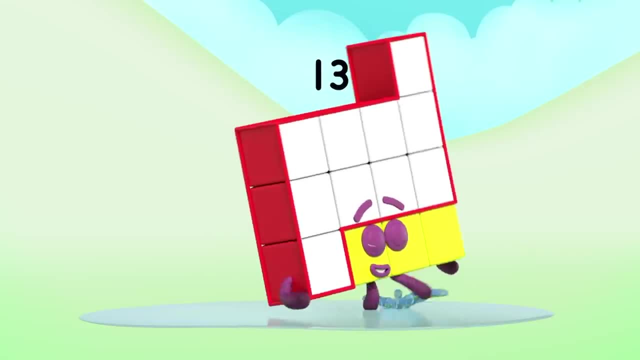 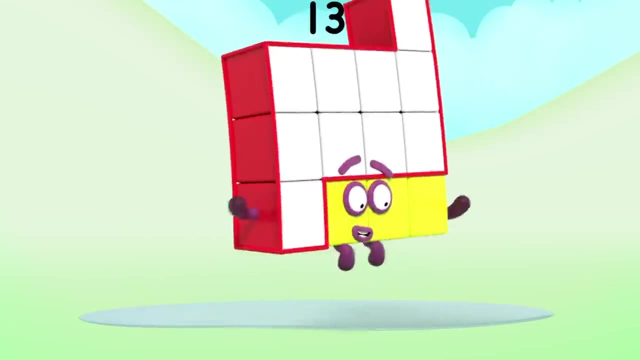 That seems to sum up my role, And wherever I end up, I'm un-cus-tine, Unlucky Number thirteen. Oh whoa, It's always the same When he says his name. Somebody should tell him that it's happened again. 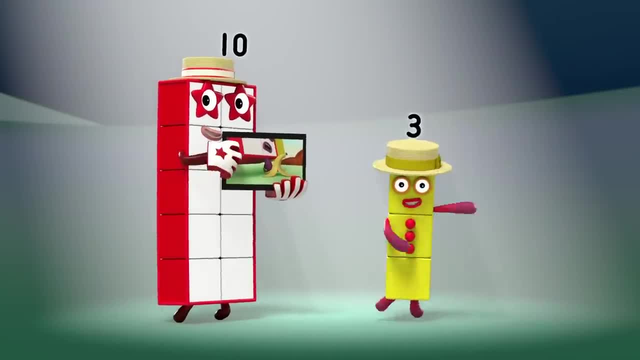 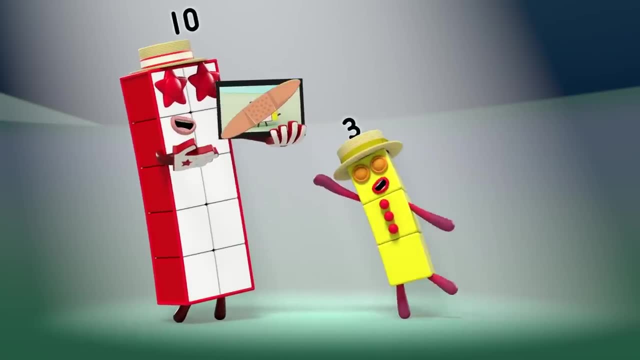 Somebody should tell him that it's happened again. Somebody should tell him that it's happened again. Somebody should tell him that's the name of the game. It's happened before A total disaster. But he's going to need more than a sticking cluster. 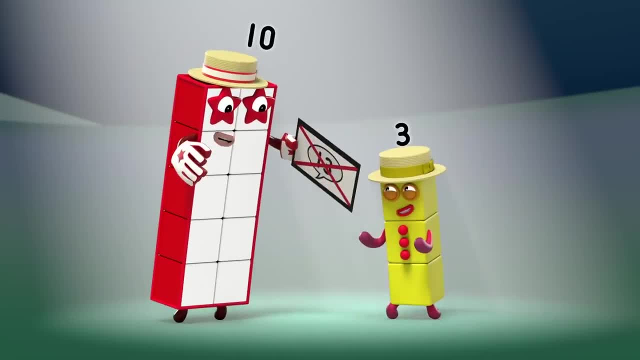 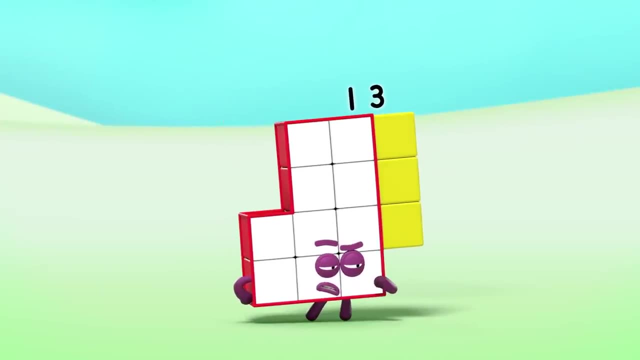 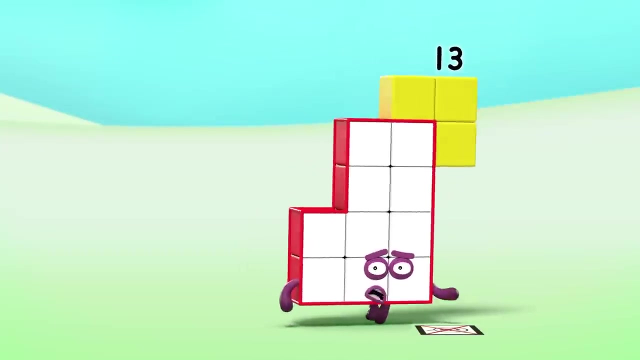 It's always the same. We know what to blame. Somebody should tell him not to mention his name. It's getting routine. I say I'm thirteen, Keep it together. This is absurd. You know what I mean. I say it's thirteen. 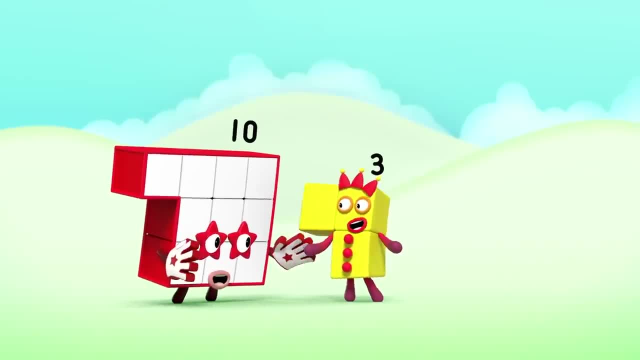 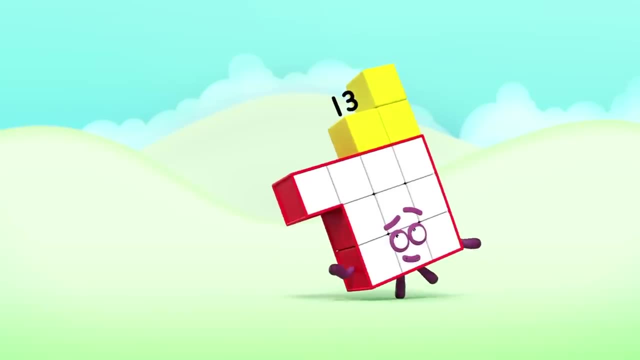 End up my tether to say that word. It's always the same, It's getting routine. They ask me my name. I say I'm fir- Thirsty, I say I'm thirsty. They ask me my number. You know what I mean. 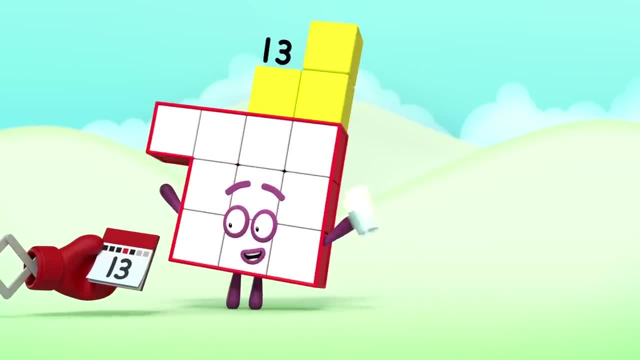 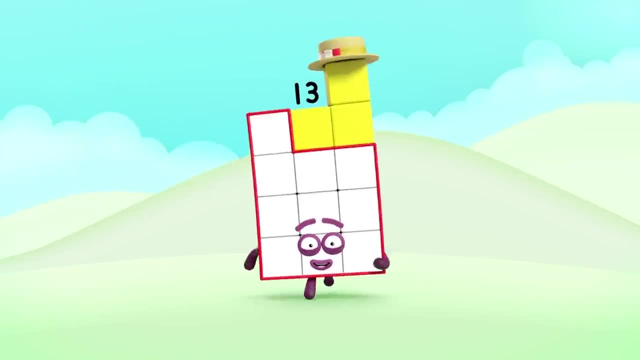 And I always say it's fir- Thursday. I always say it's Thursday, Frankly, Jack, and it's dizzying their time. This is me, 10 and 3, turning this into a game. I'm changing my luck. I won't come. 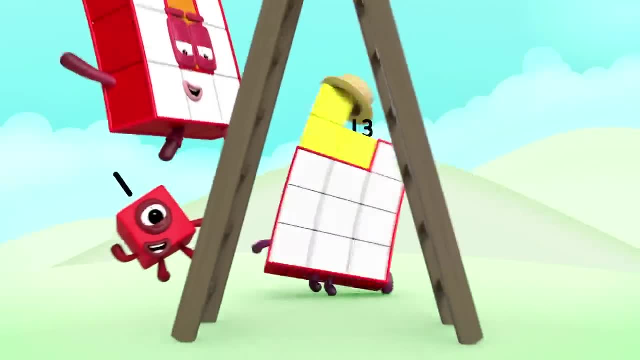 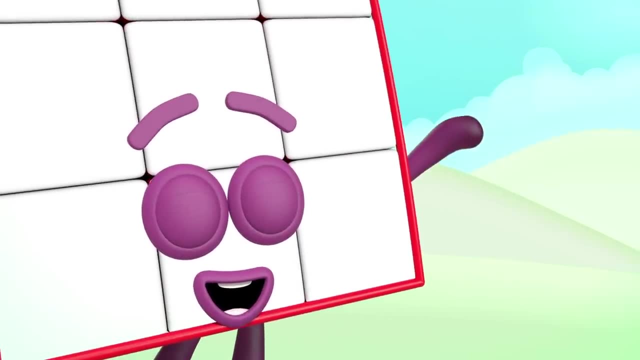 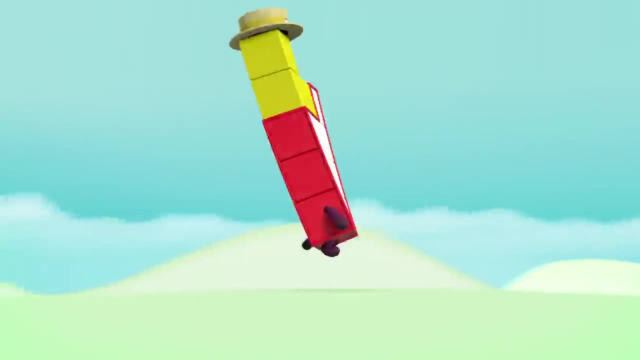 unstuck as long as I don't say my name. Call me one more than 12, or 10 and 3,, whatever you call me, I'm still me. I'm the happiest number you've ever seen, So lucky to be unlucky Number 13.. 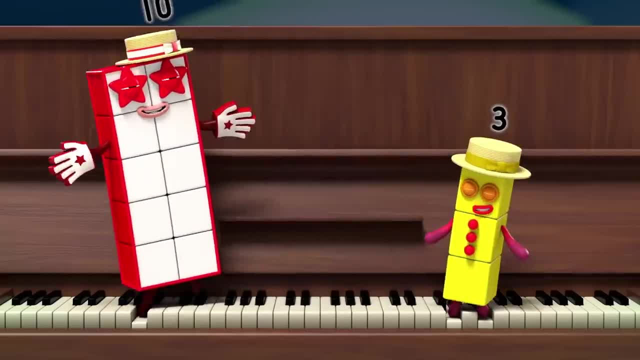 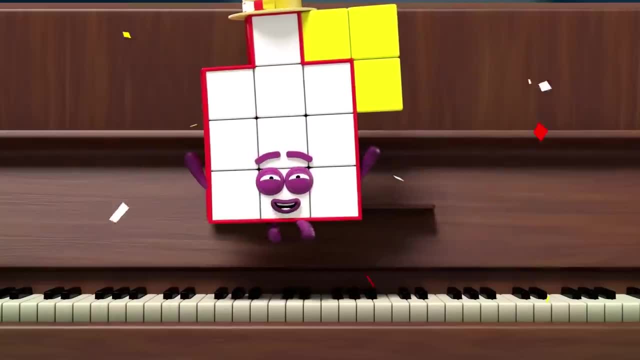 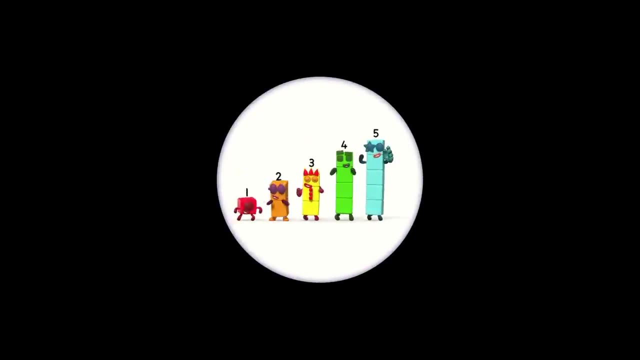 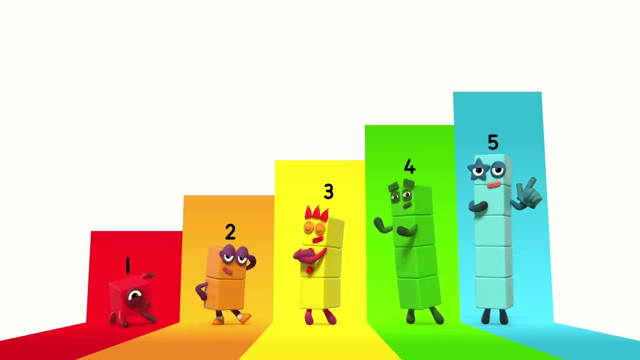 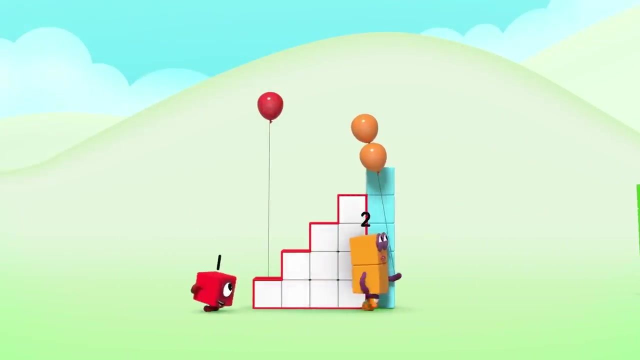 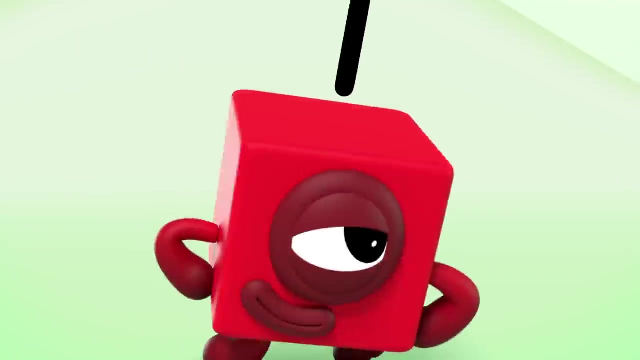 13. 13. 13. 13. 13. 13.. Unlucky me, Step Squad Agent 15, ready for action. The super special secret step squad is here. Oh, oh, free balloons. Oh, no, my balloon. This is a job for step squad. 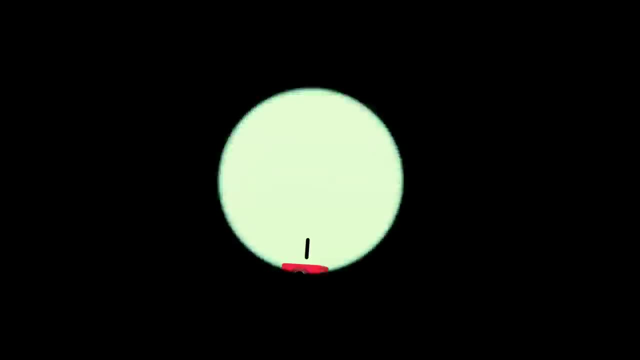 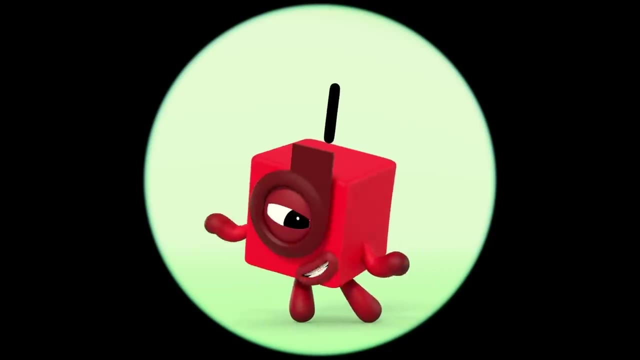 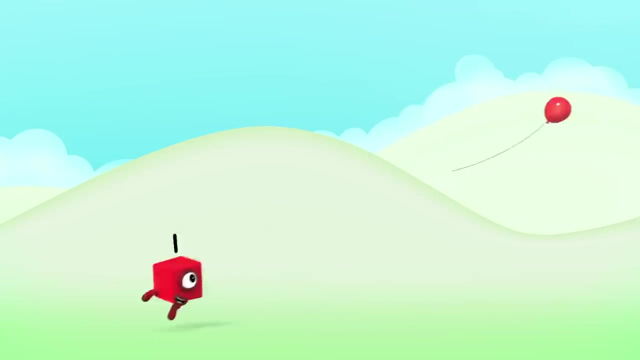 The super special secret step squad is here. Oh me A step squad, all by myself. I'll give it a go. Oh, step one, chase the balloon. My plan is working perfectly. One plus two equals three. One, two, three, Three escaped balloons. 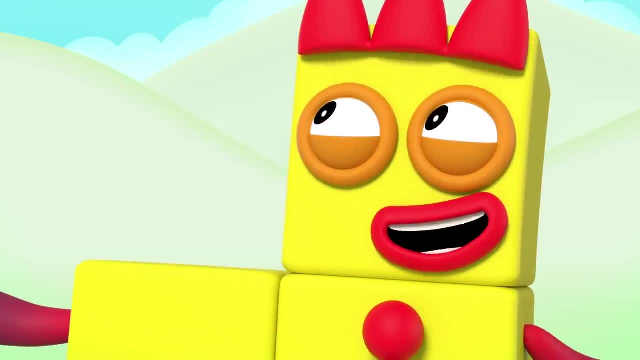 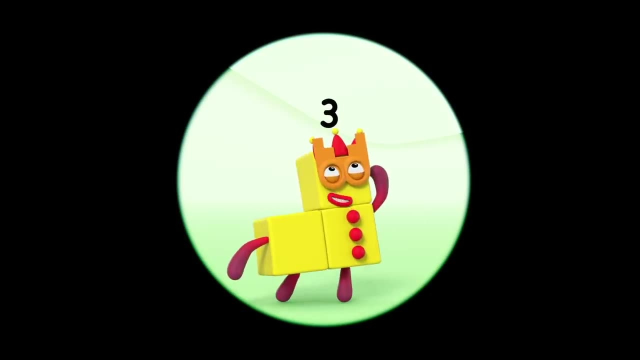 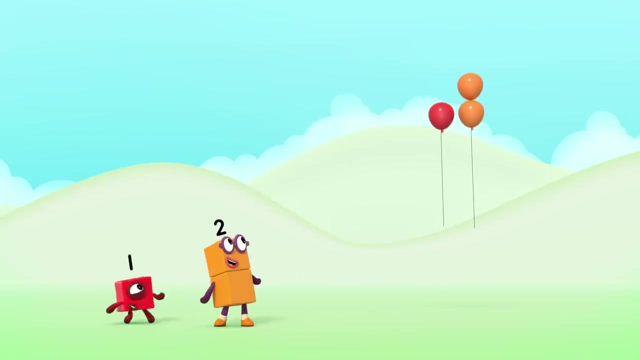 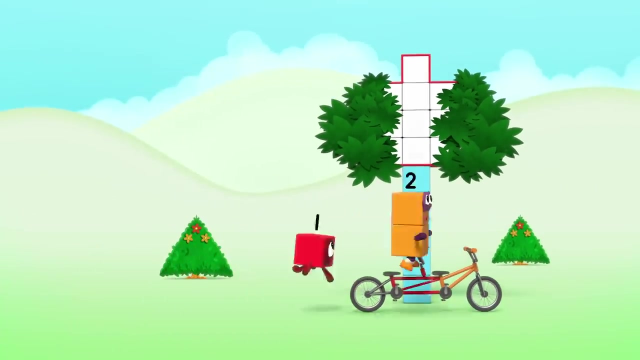 If only step squad were here. The super special, secret step squad is here. Look at me, I'm step shaped too. Maybe I can be a step squad. Step one chase, Step two, peddling hard, Hush, Hush, hush. 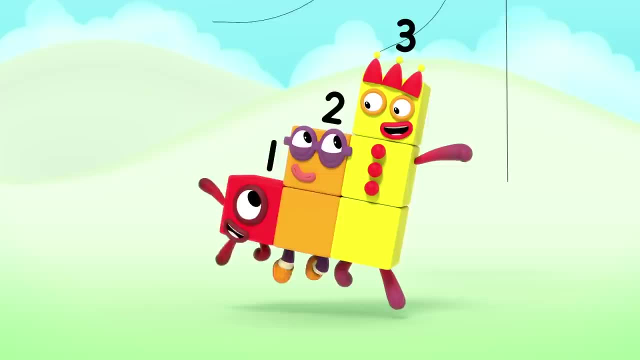 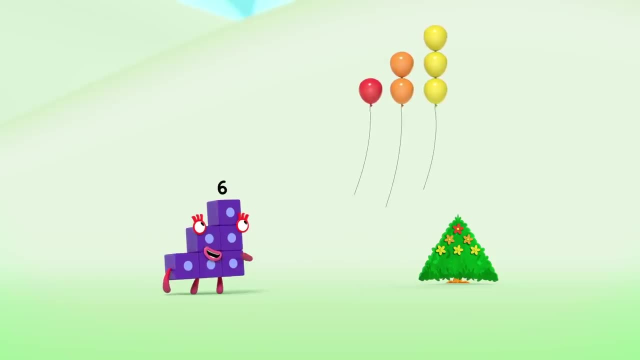 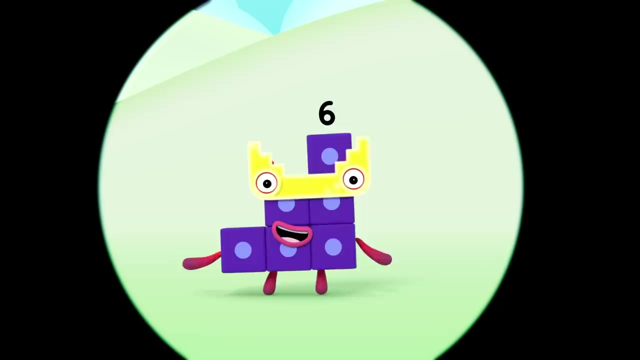 Look out: One plus two plus three equals six. One, two, three, four, five, six. Six balloons have now been freed. I know exactly who we need. The super special secret step squad is here. Look at that. It must be true. 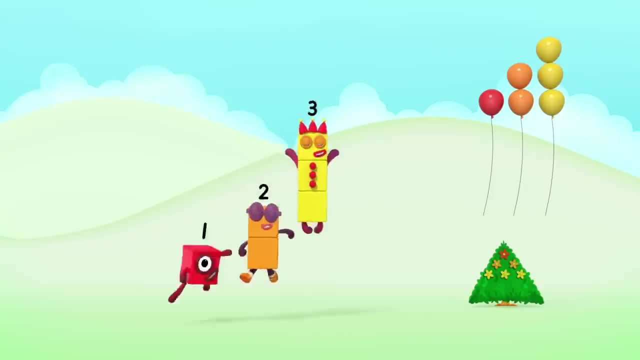 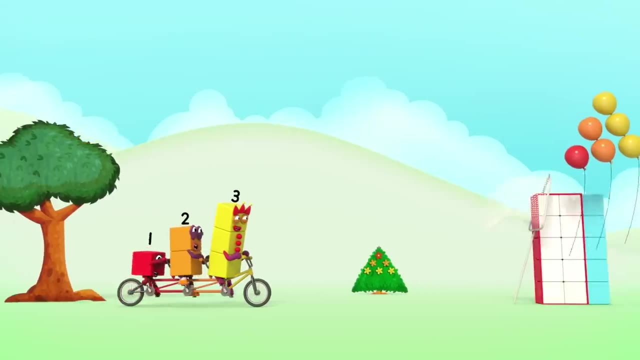 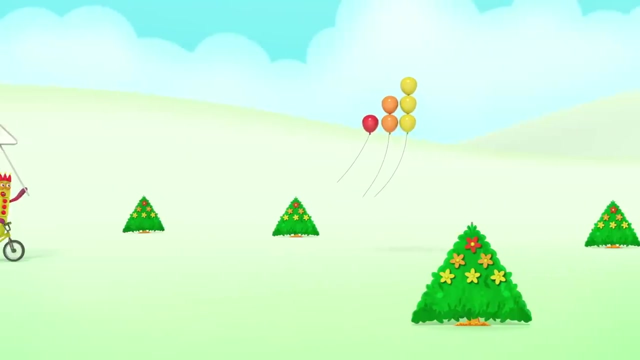 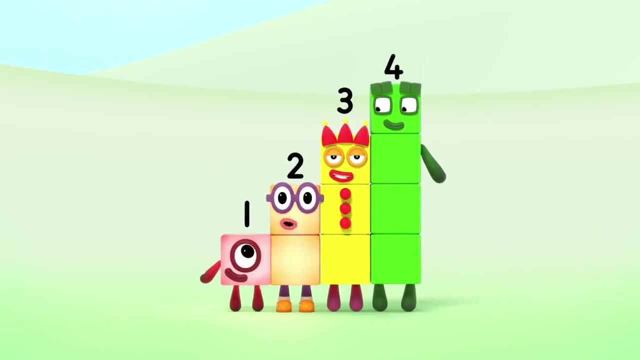 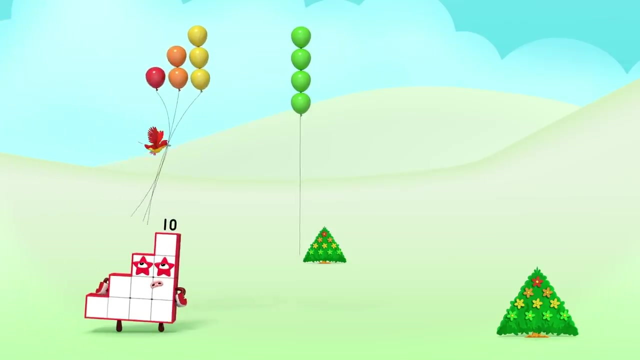 I can be a step squad too. Step one, chase. Step two, peddling hard. Step three with a net: Hush, hush, Hey, One plus two plus three plus four equals ten. You, naughty bird, You bring that to me. 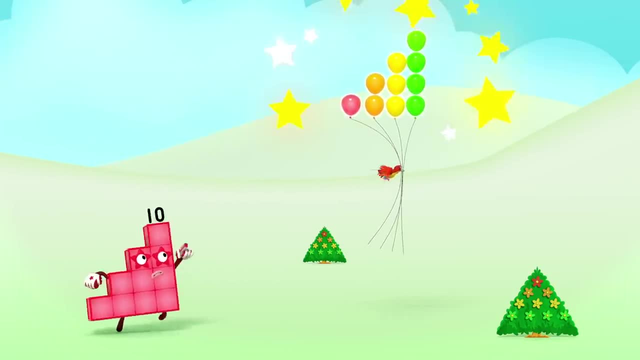 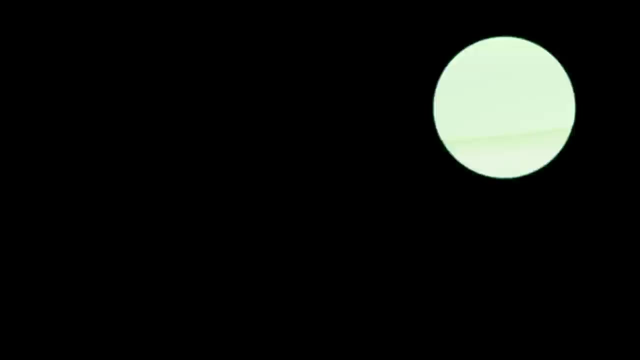 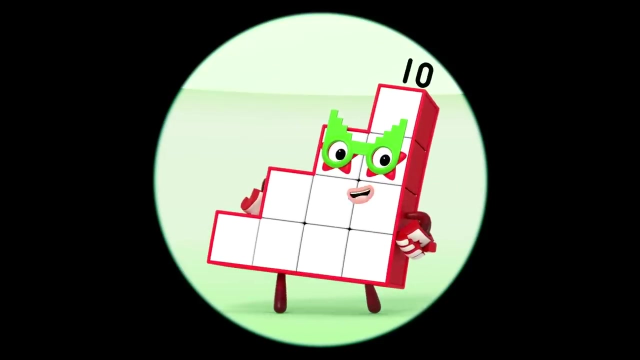 One, two, three, four, five, six, seven, eight, nine, ten, Ten balloons back. I need step squad. The super special secret step squad is here. Can it be? Yes, it can, I'm a step squad too. 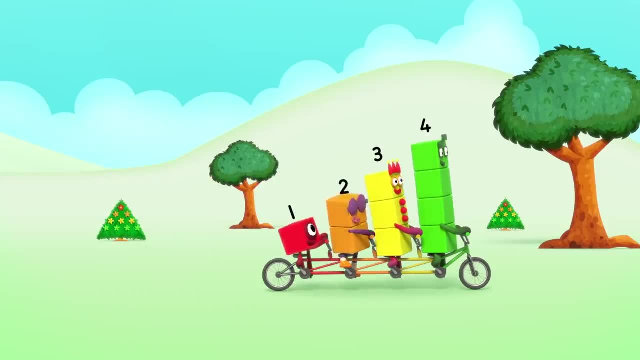 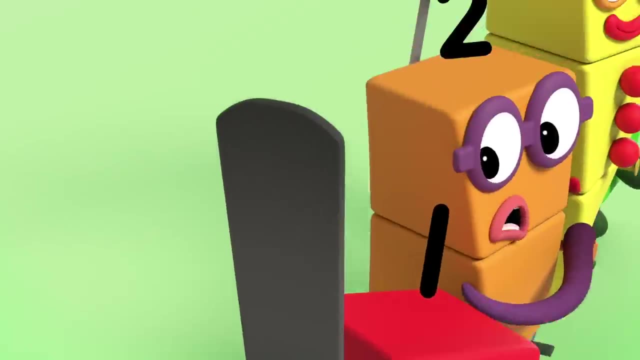 Step one: chase. Step two, peddling hard. Step three: with a net. Step four: rest the square One. two, three, four, five, six, seven, eight, nine, ten. I'm a step squad too.